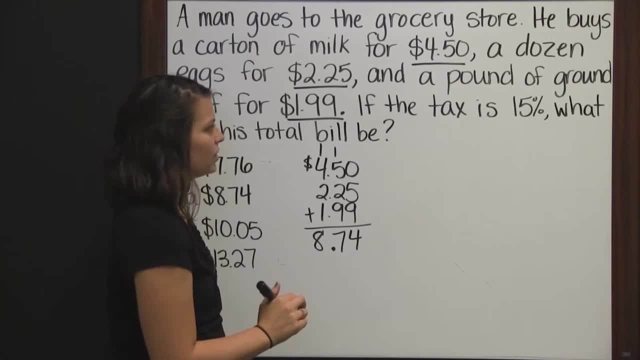 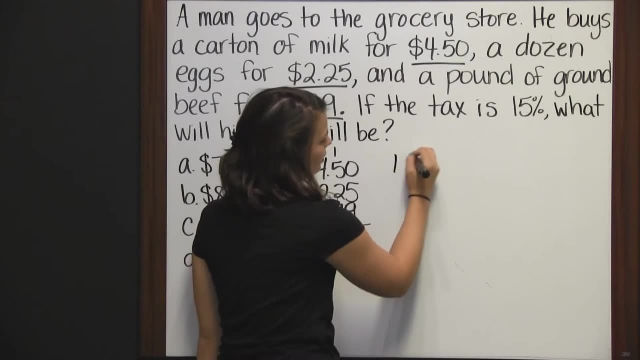 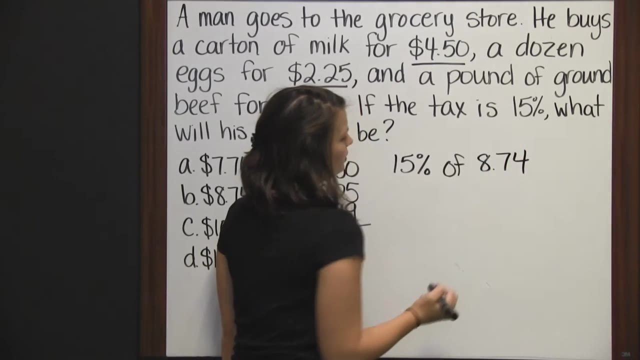 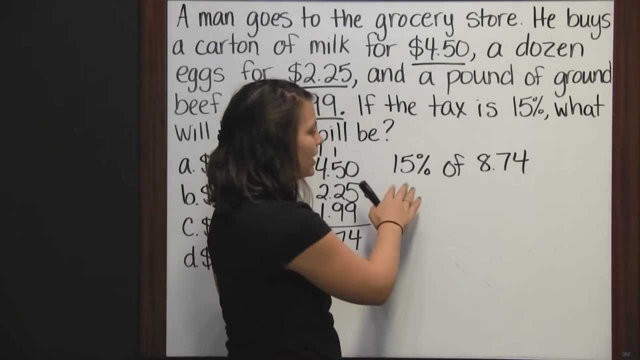 he's going to pay on what he's buying, So he's going to pay 15% of his total. Let me write that out: 15% of his total, which is $8.74.. Now of and math usually means to multiply, But I can't take this percent and multiply. it times $8.74. 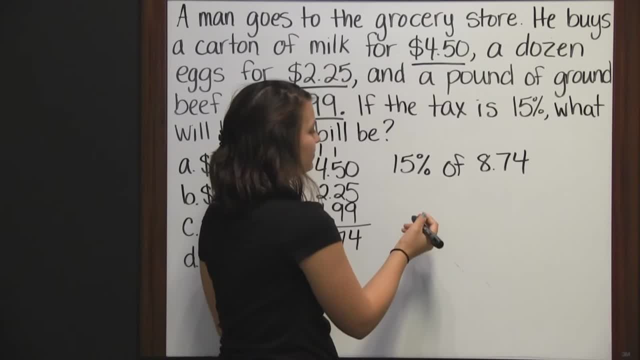 First we have to change the percent into a decimal And to do that, the decimal is at this point behind our number. To change our percent into a decimal, we have to take it and move it two places to the left. So to find the tax, we'll take the tax and we'll 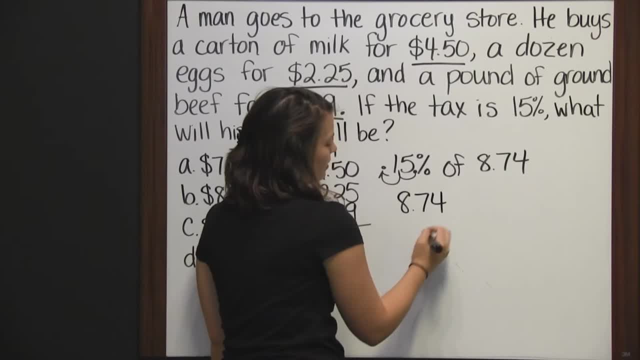 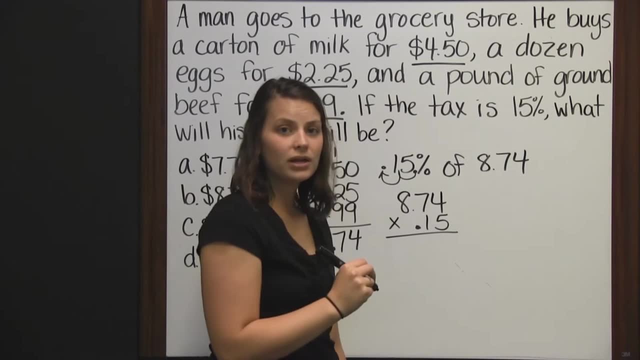 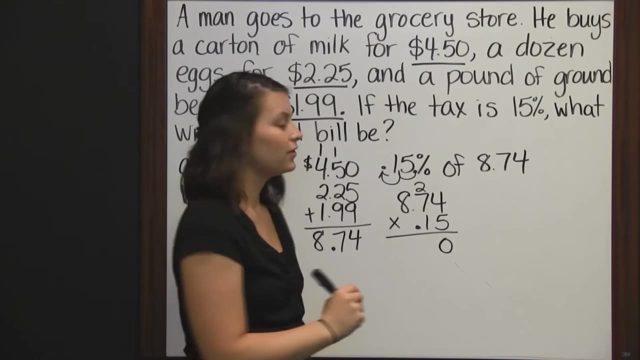 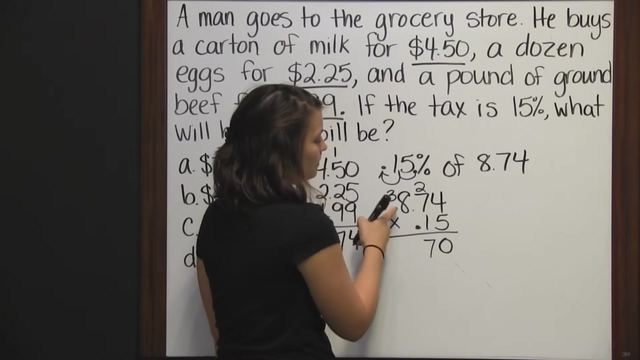 take $8.74 and multiply it times 15 hundredths. 5 times 4 is 20.. Write the 0, carry the 2.. 5 times 7 is 35, plus 2 is 37.. Write the 7, carry the 3.. 5 times 8 is 40, plus 3 is. 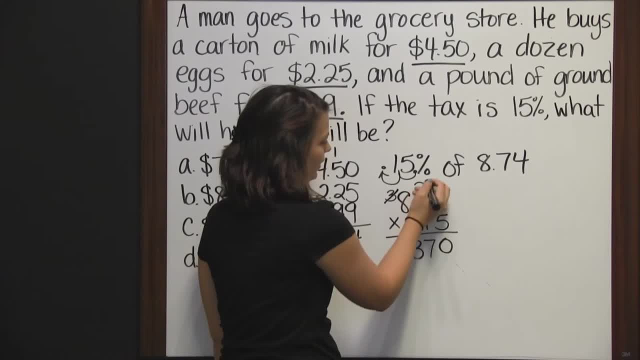 43. And then we'll get rid of these, because now we need to multiply times 1.. So first write a 0 placeholder, since we're not multiplying in the ones place anymore, And then take 1 times 4 to get 4.. 1 times 7 is 7.. 1 times 8 is 8.. And now we can add those together. 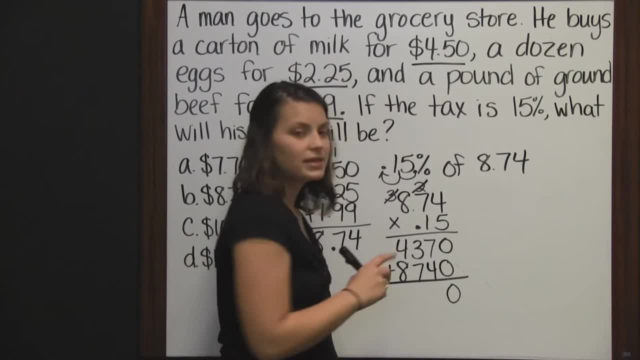 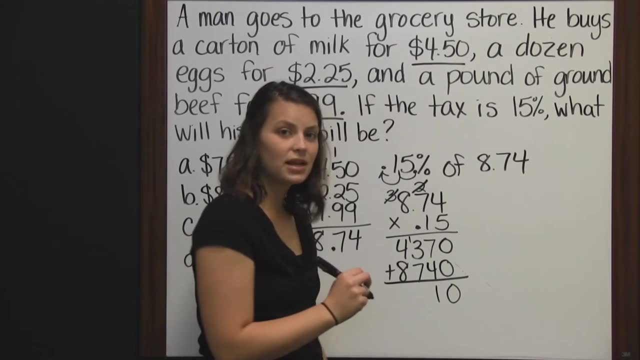 0 plus 0 is 0.. 7 plus 4 is 11.. So write the 1, carry the 1.. 3 plus 7 is 10, plus another 1 is 11.. Write the 1, carry. 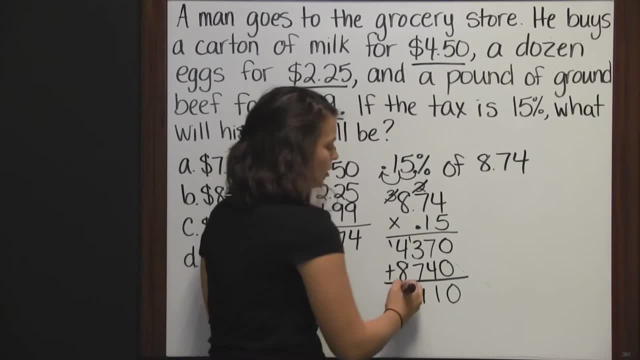 the 1.. Then we have 8,, 9, plus 4,, 13. And there are 4 numbers total behind the decimal places, which means our answer will also have 4 numbers behind the decimal places. So we'll. 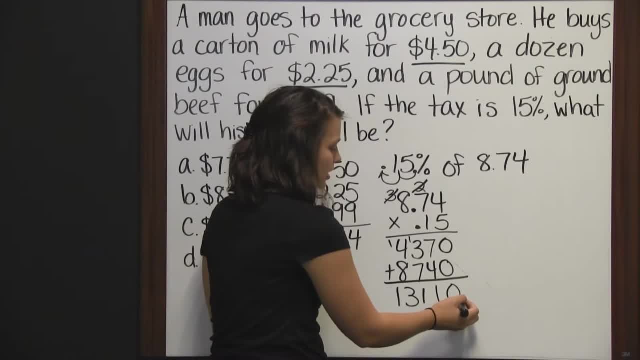 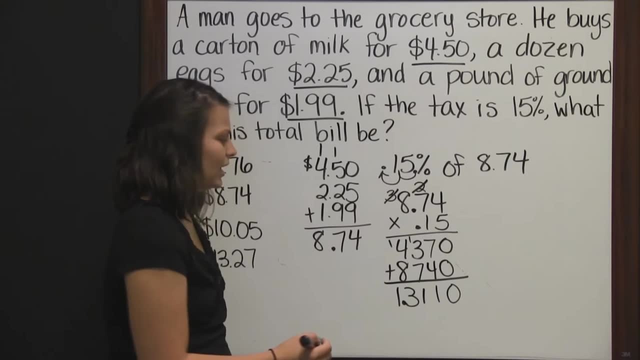 have 4 numbers behind the decimal. So here's our decimal: We have 1,, 2,, 3, 4 numbers behind the decimal And that doesn't look like an amount of money I've ever seen. but if we 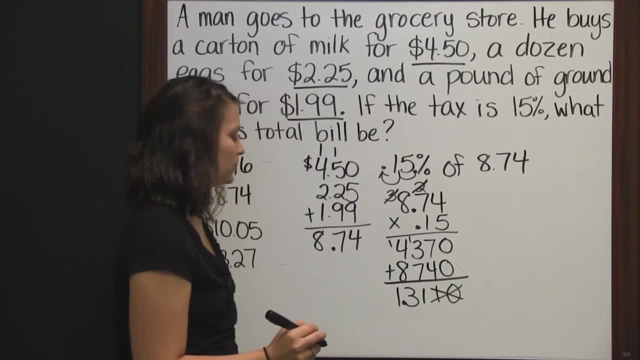 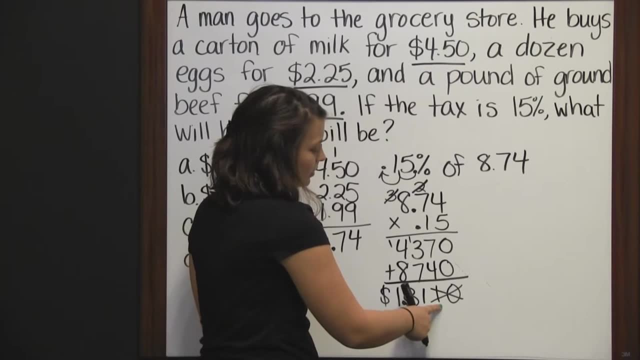 take. get rid of these last two, then we have $1.31.. And we can do that, since 1 wouldn't cause this 1 to be rounded up, Since we only round up if the number is 5 or above. So we can really just get rid of. 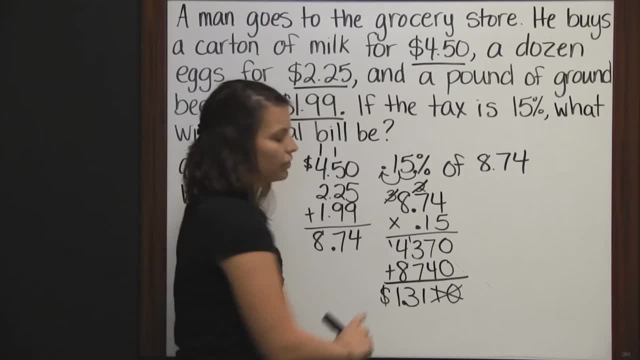 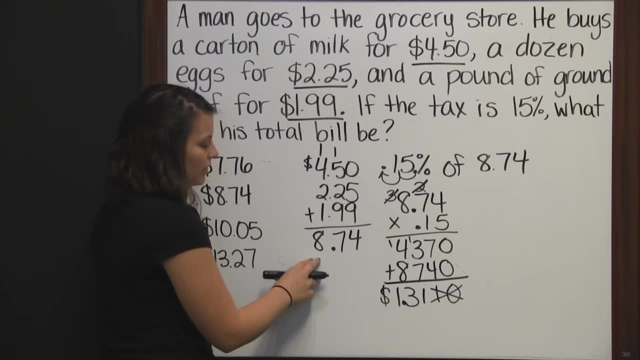 them. So that means that he's going to pay $1.31 in tax. So we take his total before tax and then add the tax to it, So $1.31.. And don't forget to line up those decimals. 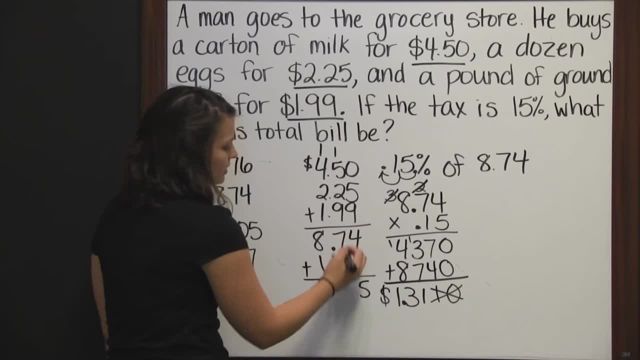 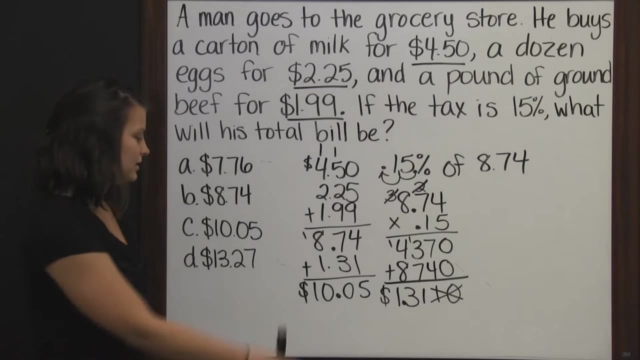 4 plus 1 is 5.. 7 plus 3 is 10.. So write the 0,, carry the 1.. Bring that decimal down to the answer. Then we have 8,, 9,, 10.. So his total with tax and everything is $10.05,, which is answer. 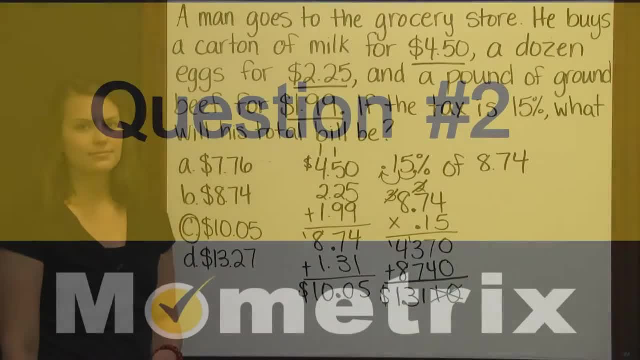 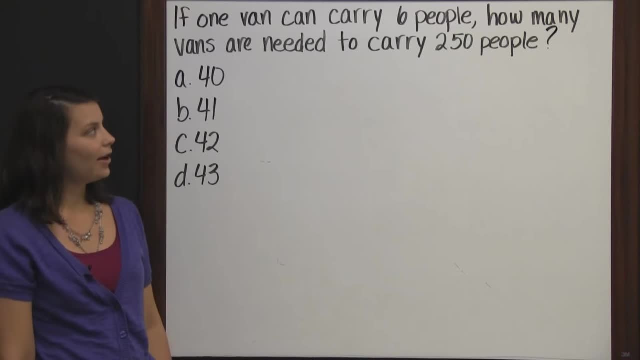 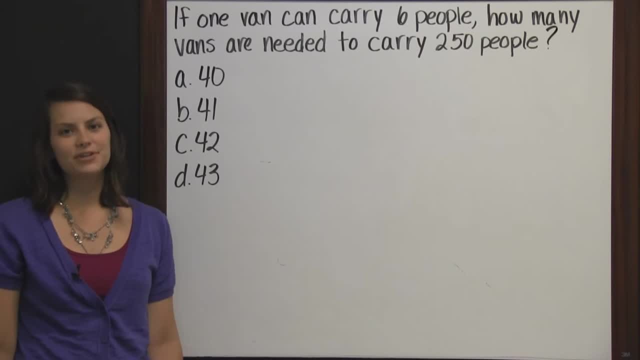 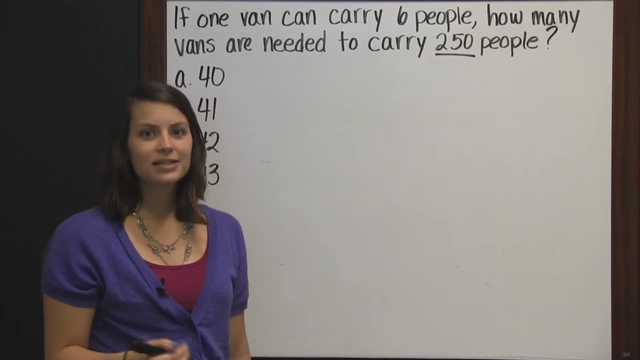 How many vans are needed to carry 6 people? How many vans are needed to carry 250 people? Well, this is a division problem, Because we're going to divide up these 250 people into vans: 6 people in each van. 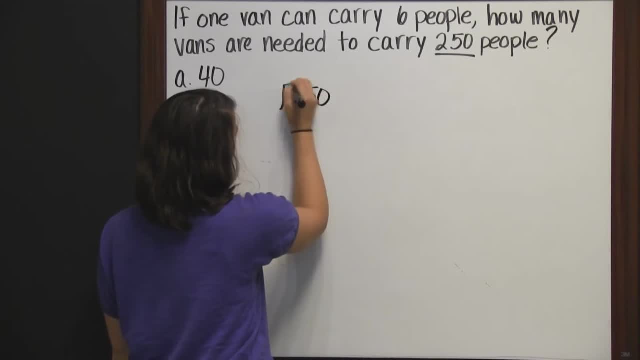 So we take 250 and divide it by 6.. 6 doesn't go into 2, but it does go into 25.. 6 goes into 25. 4 times 4 times 6 equals 6 times 25.. 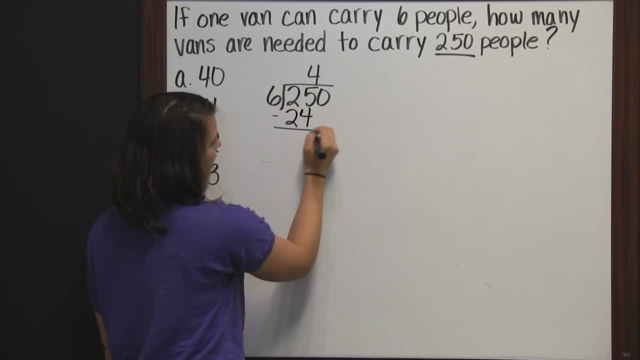 6 times 5, equals is 24.. We subtract and get 1, and bring down the 0. Then 6 goes into 10. one time. 6 times 1 is 6.. We subtract and we get 4.. You might be tempted to think that the answer is 41. 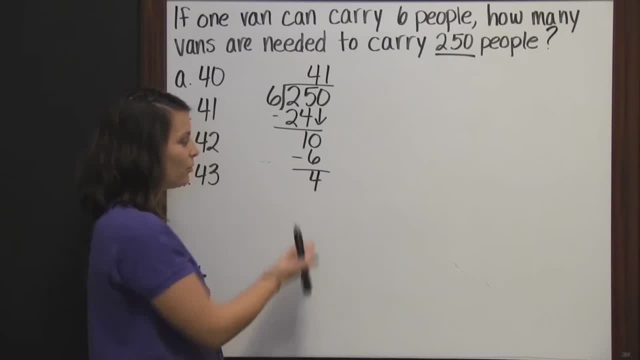 bands with 4 left over. but are we just going to leave those 4 people stranded? No, we're going to have to put them in a van as well. Since it will take 41 vans to carry all but 4 people, we'll need 1 more van for those 4 people. So we'll need to take 42 vans. 10. If one plant requires 2 litres of water each day, how many litres are required to water the plant plant for 13 days? For one day, this plant requires 2 liters of water, but we're going to water this plant for 13 days. That means we're going to water this plant 13 times. 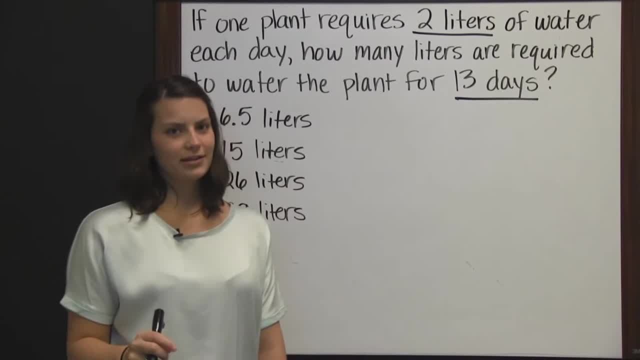 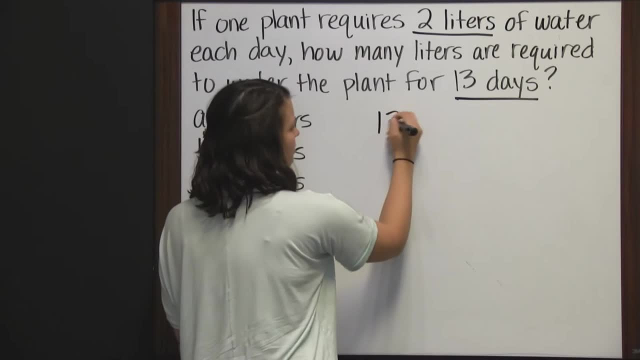 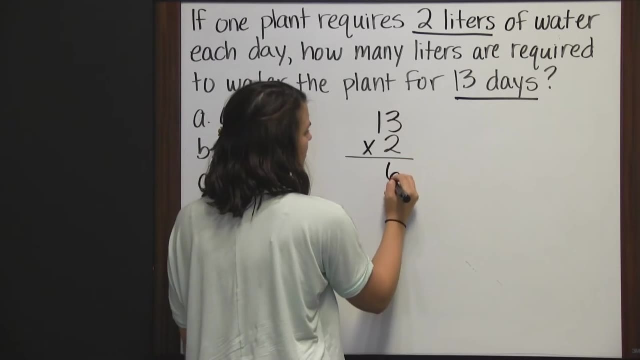 Each time we water it, we're going to put 2 liters of water in it. Since we're going to water this plant 13 times, we're going to multiply 13 times 2.. 2 times 3 is 6, and. 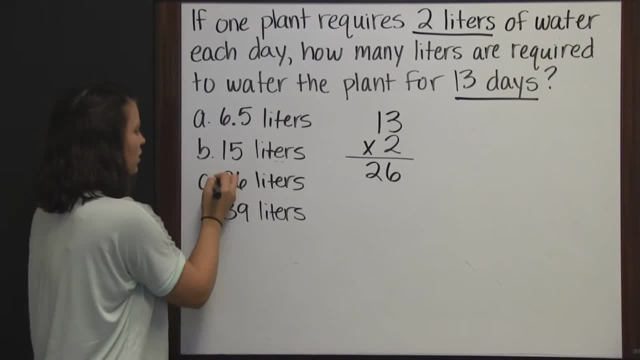 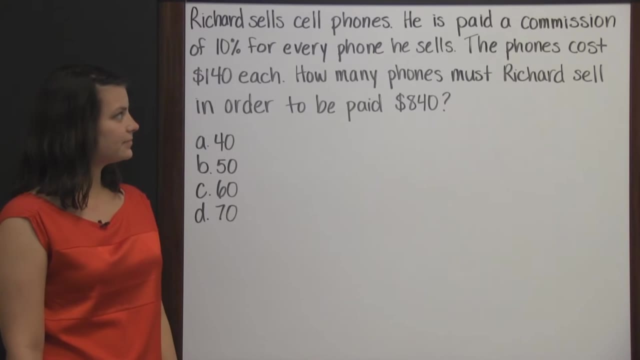 2 times 1 is 2.. That means it will take 26 liters of water for this plant to be watered for 13 days. Richard Sells Cell phones. He is paid a commission of 10% for every phone he sells. The phones cost. 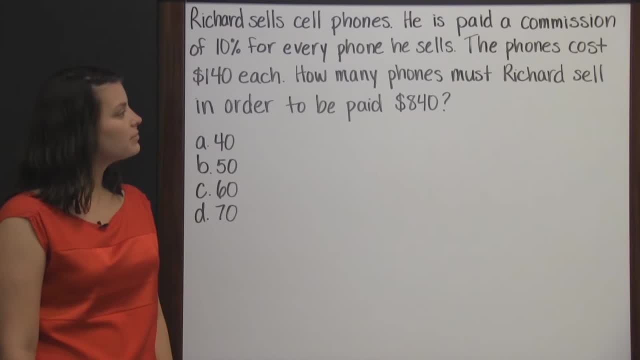 $140 each. How many phones must Richard sell in order to be paid $840?? First we want to figure out how much he makes from selling each phone. We know that he makes 10% of the cost of selling each cell phone. We know that he makes 10% of the cost of selling each cell. 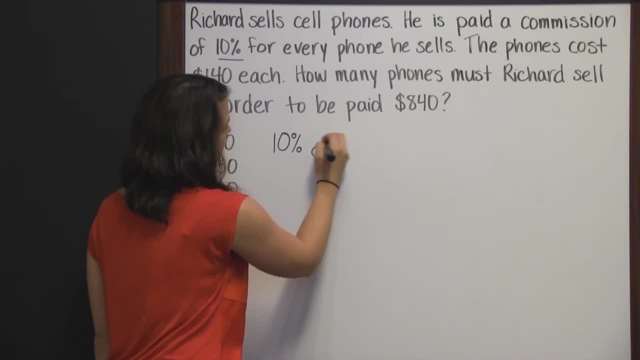 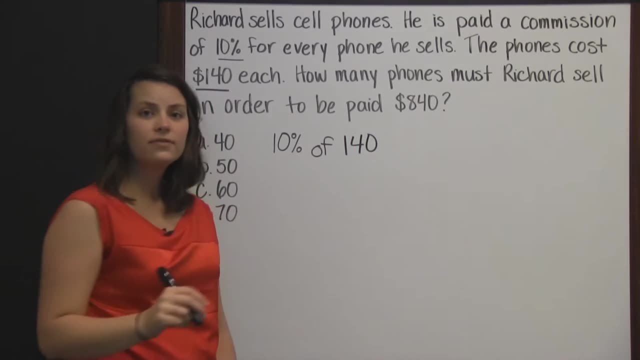 phone. To get 10% of the cost of selling the cell phone, we need to multiply. If we can do this, then we have an estimated cost of $140. Of the cost of the phone, which is 170, as well as the cost of 10% of the cost of the cell phone. Of means to multiply We need 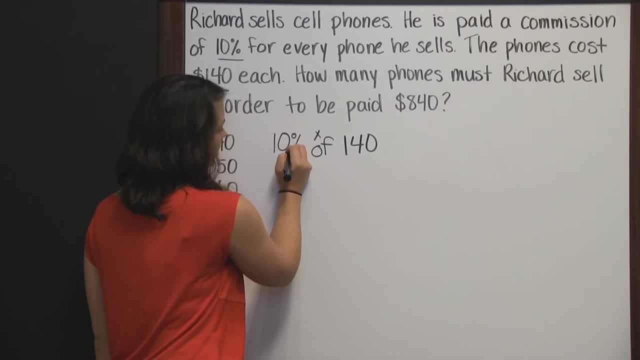 to change our percent to a decimal. We take the decimal and move it two places to the left. so that means we're multiplying 140 times 1 tenth. 1 times 0 is 0,. 1 times 4 is 4,, 1 times 1 is 1.. 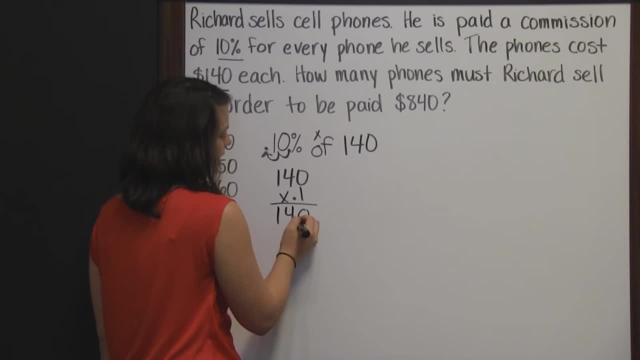 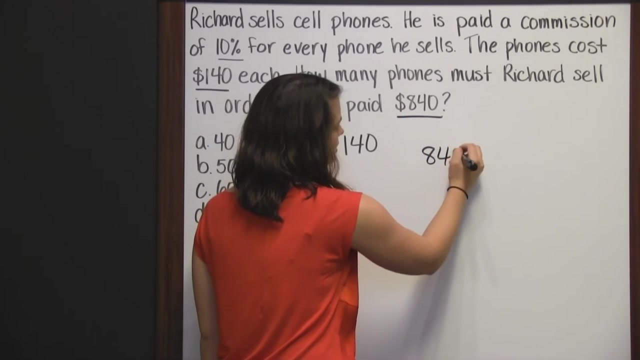 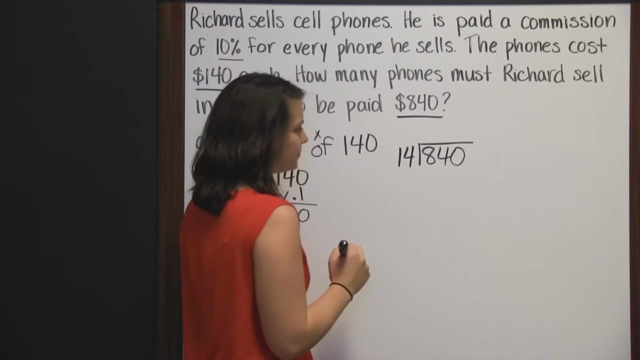 We have one number behind the decimal, so our answer should have one number behind the decimal. So that means that he's making $14 for every phone he sells And if he wants to be paid $840, then we need to take that $840 and divide it by $14. 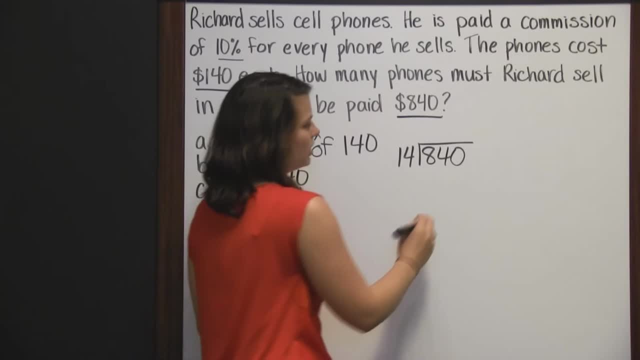 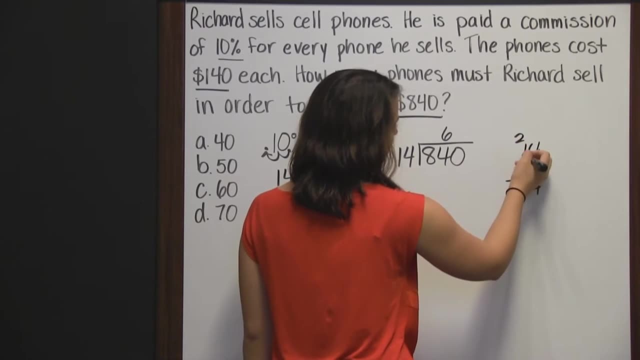 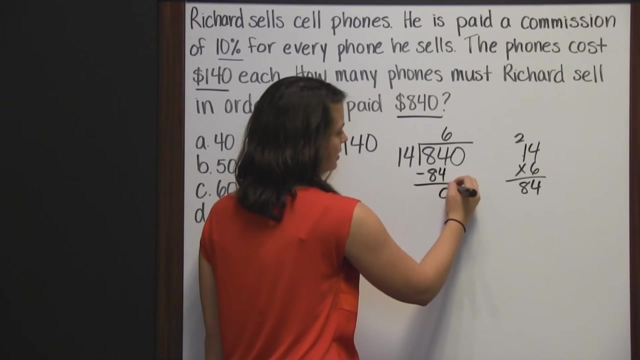 So 14 goes into 84. six times 14 times 6, 24,. carry the 2, 6 times 1 is 6, plus 2 is 8.. So it goes in perfectly. When we subtract, we get 0, and bring down 0.. 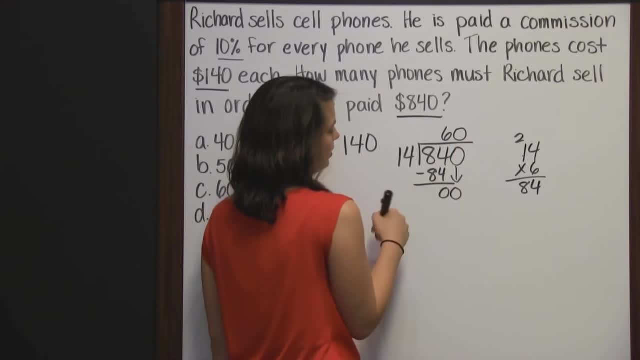 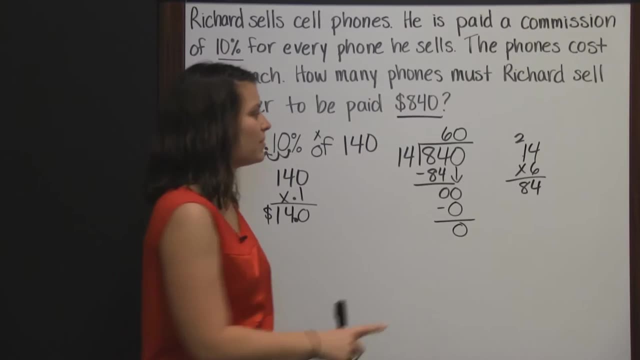 And we subtract And 14 goes into 0, 0 times 14 times 0 is 0.. When we subtract, we get a remainder of 0.. So that means that Richard needs to sell 60 phones in order to make $840. 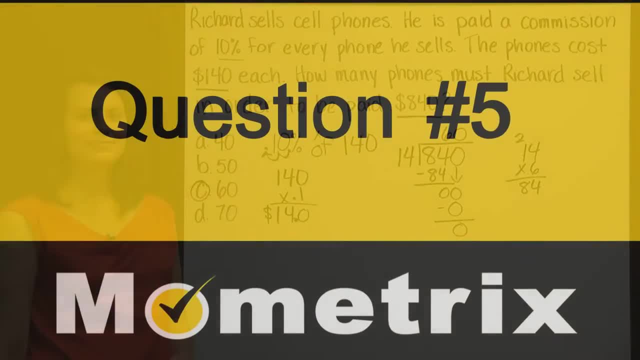 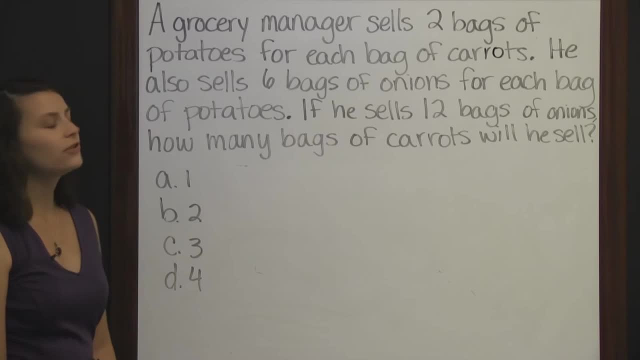 Answer C: A grocery manager sells two bags of potatoes for each bag of carrots. He also sells six bags of onions for each bag of potatoes. If he sells 12 bags of onions, how many bags of carrots will he sell? Let's start by picking out the important information. 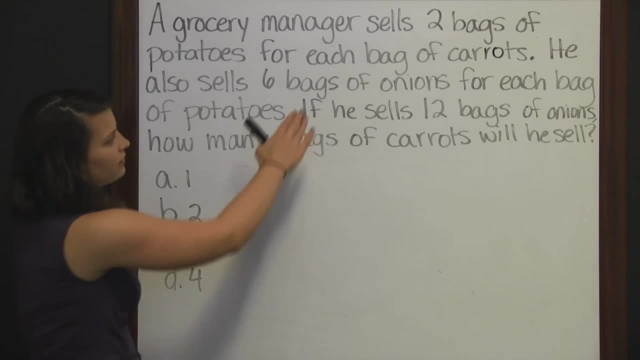 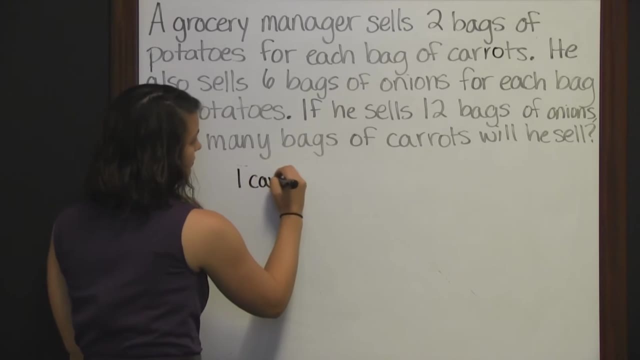 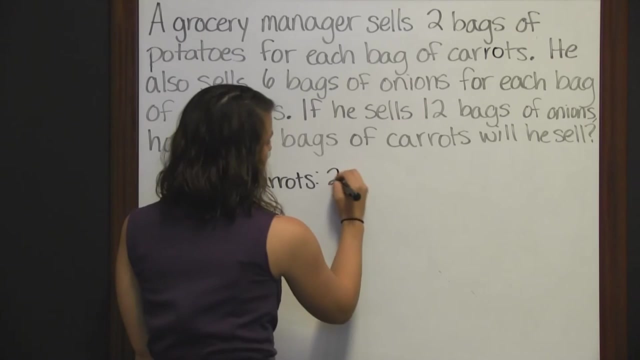 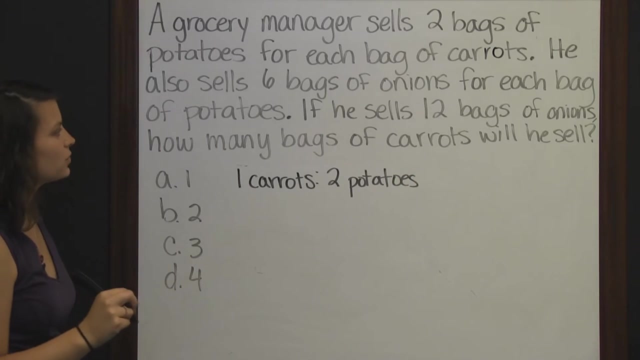 In the first sentence we're told that for each bag of carrots- so each- that means one. so for one bag of carrots he sells two bags of potatoes. In the second sentence, we're told that for each bag of potatoes. 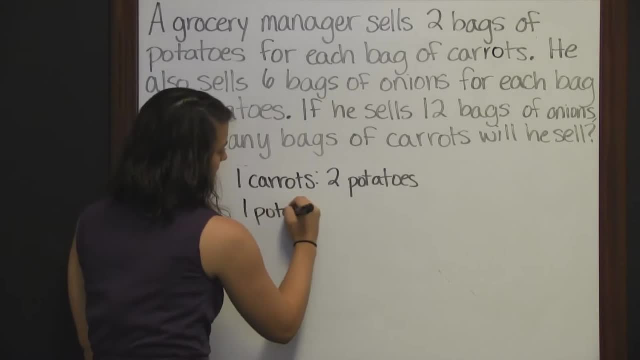 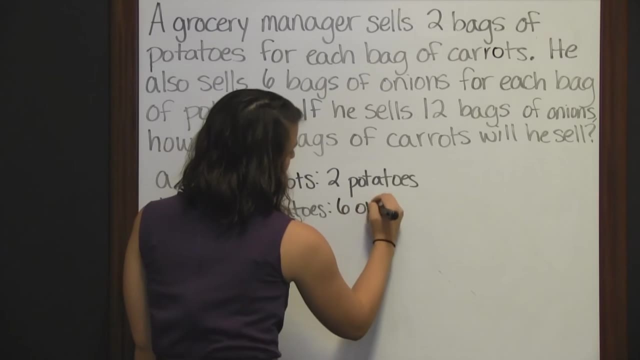 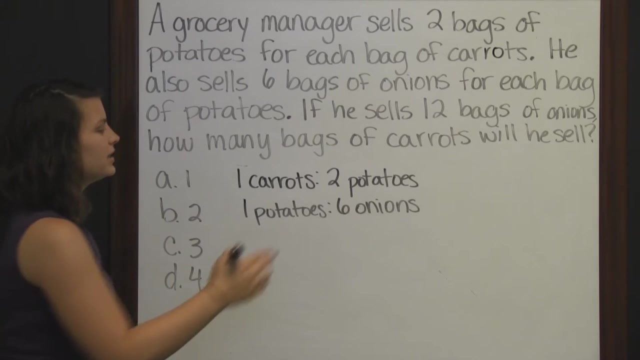 he sells six bags of onions. Then in the third sentence we're told that for each bag of potatoes he sells 12 bags of onions. Then in the third sentence in our question it says: if he sells 12 bags of onions, 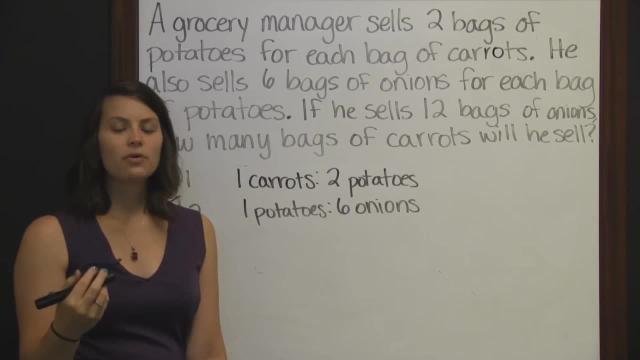 how many bags of carrots will he sell? So let's start with what we know. He sold 12 bags of onions. So where do we find that in our information? Well, six bags of onions is one bag of potatoes, So 12 bags of onions would be how many bags of potatoes? 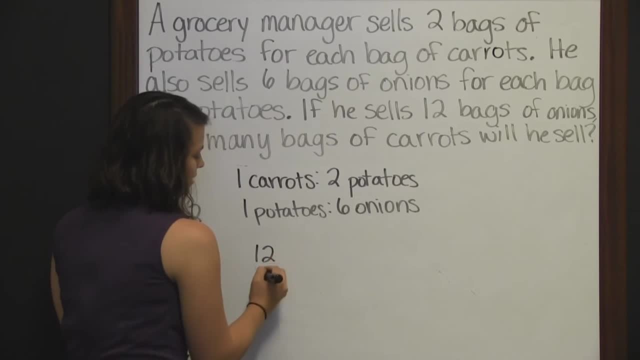 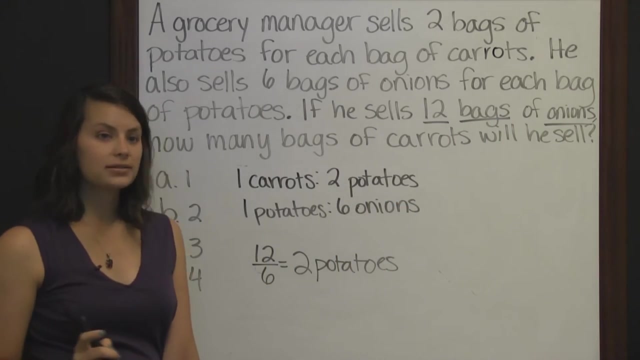 So we take 12, and divide that by six and we get two. So that's two bags of potatoes. If he sold 12 bags of onions, then that means he sold two bags of potatoes And if we go back to that information we were given, 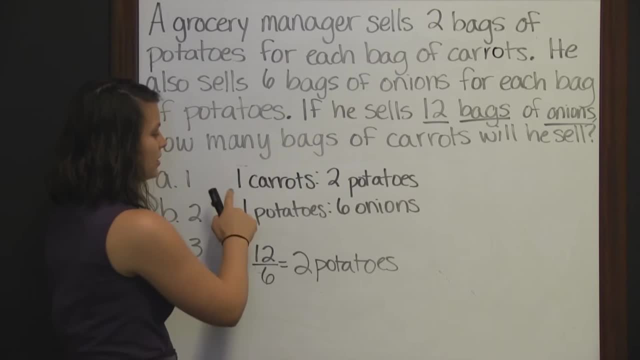 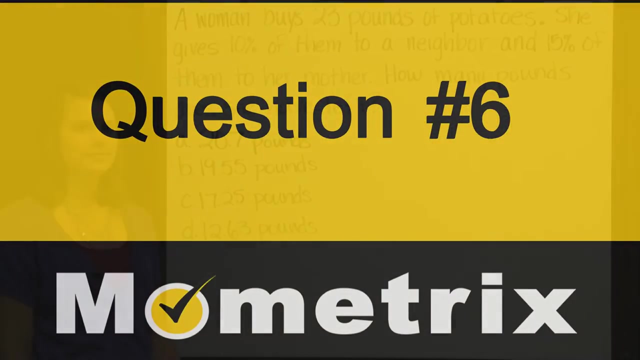 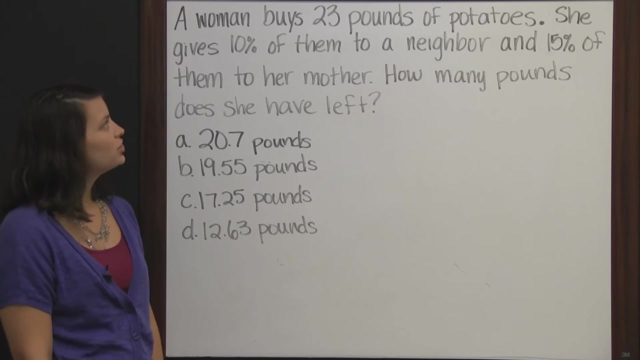 if he has sold two bags of potatoes, then that means he sold one bag of carrots, which is what they asked us to find out How many bags of carrots? And the answer is one. A woman buys 23 pounds of potatoes. She gives 10% of them to a neighbor. 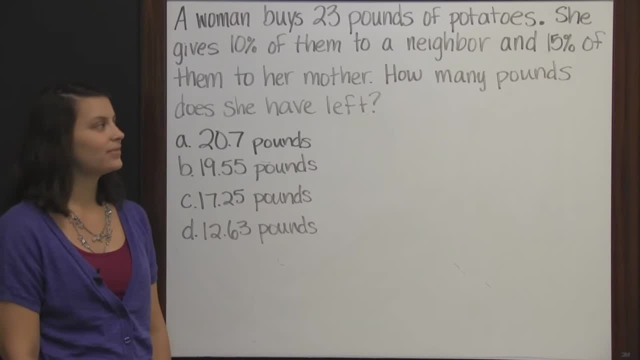 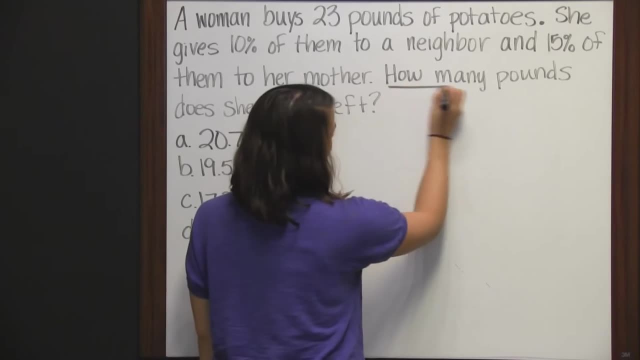 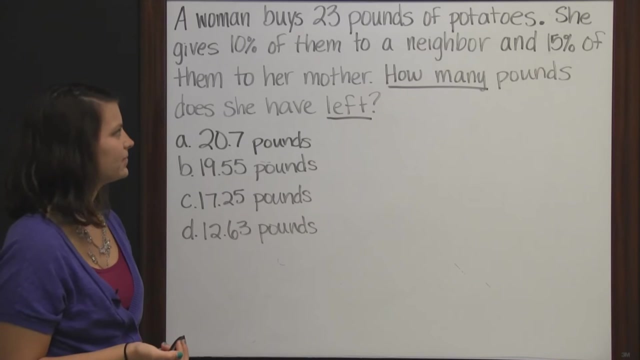 and 15% of them to her mother. How many pounds does she have left? So this phrase how many left? tells us that we're going to need to subtract, But subtract what She starts out with: 23 pounds, But it doesn't tell us. 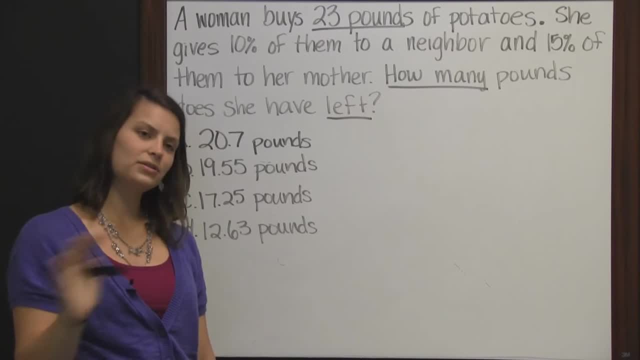 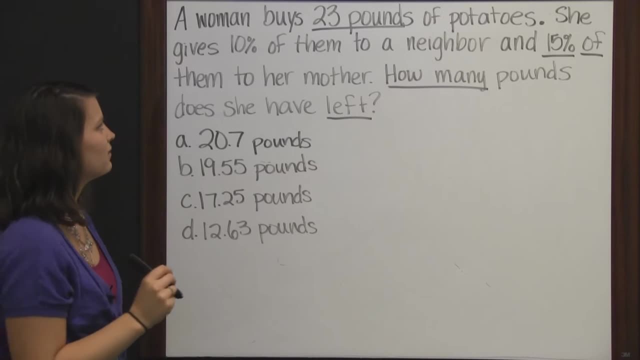 and she gives two pounds away to this person and four pounds away to this person. They tell us what percent of 23 pounds is given away And again, what percent of the 23 pounds is given away. So we need to figure out how many pounds that is. 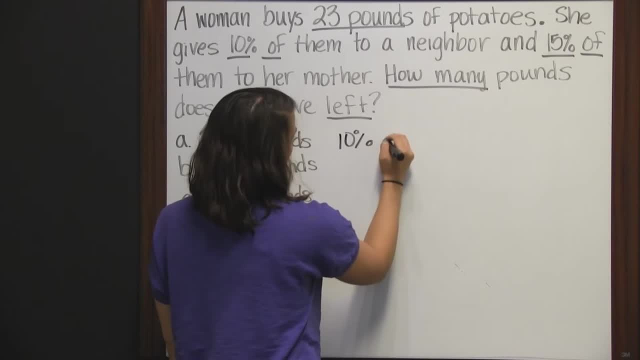 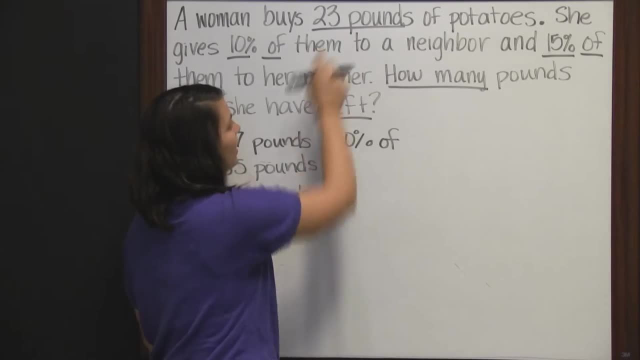 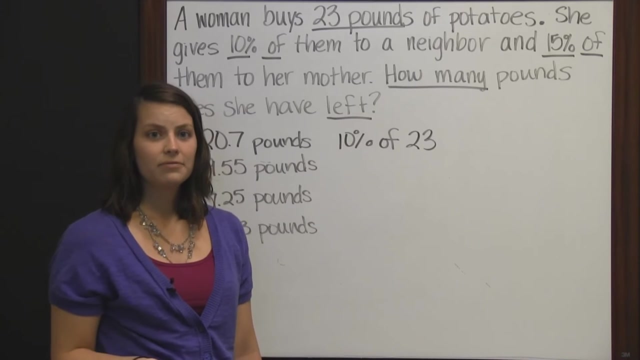 Let's start with 10% of, and it says of them. And what does them refer to? Well, it refers back to the 23 pounds. So it's 10% of 23 pounds Of means to multiply And we're going to multiply 10% and 23.. 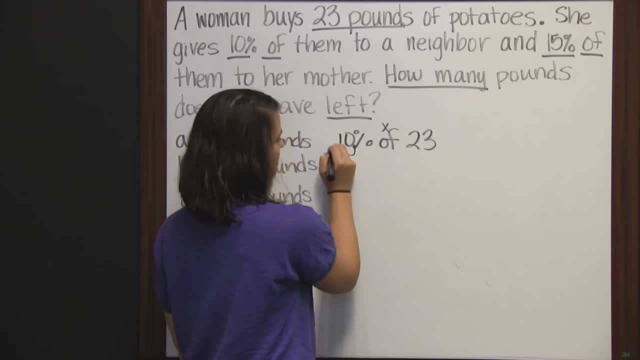 But first we have to take our percent and change it to a decimal. So we move the decimal two places over. Now we can multiply 23 times 1 tenth, or 10 hundredths, and those are the same. So I'm just going to multiply times 1 tenth. 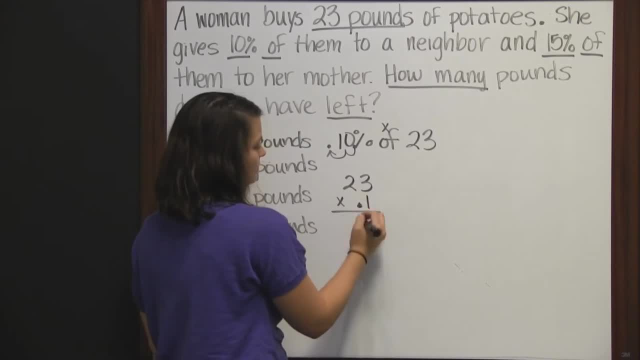 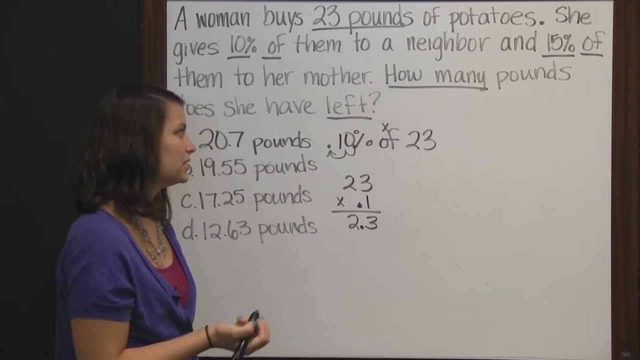 1 times 3 is 3, and 1 times 2 is 2,, with one number behind the decimal. So that's 2 and 3 tenths pounds. that was given to the neighbor. Now we're going to do something similar. 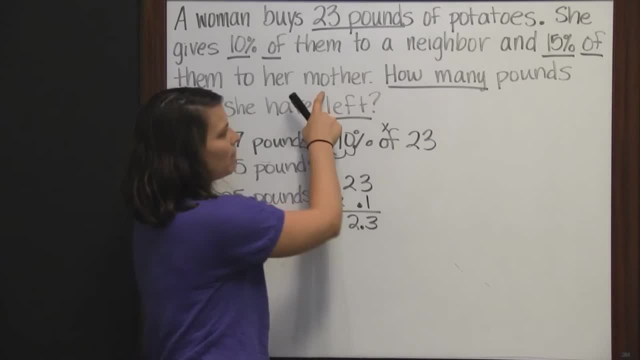 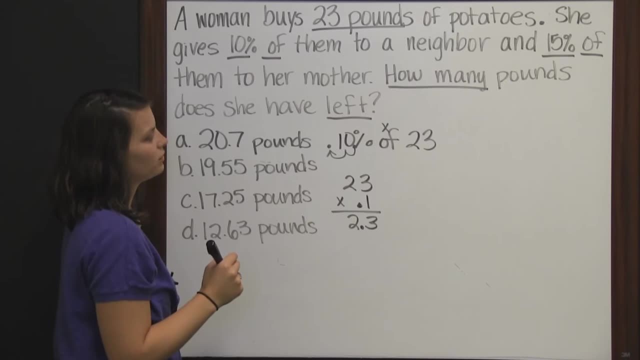 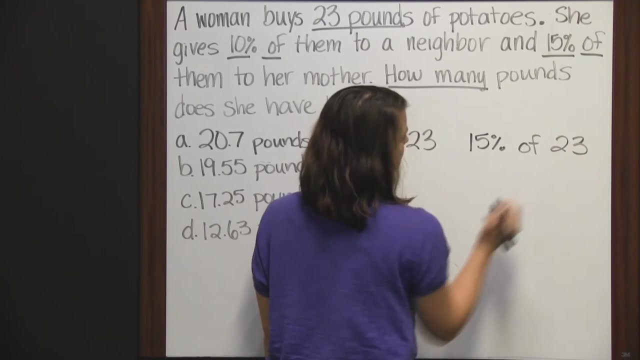 to figure out how much was given to her mother. To her mother she gave 15% of them And again the them refers back to the 23 pounds. So 15% of 23 pounds And again of means to multiply. 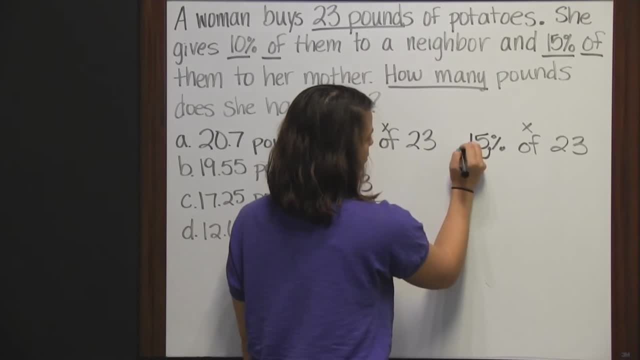 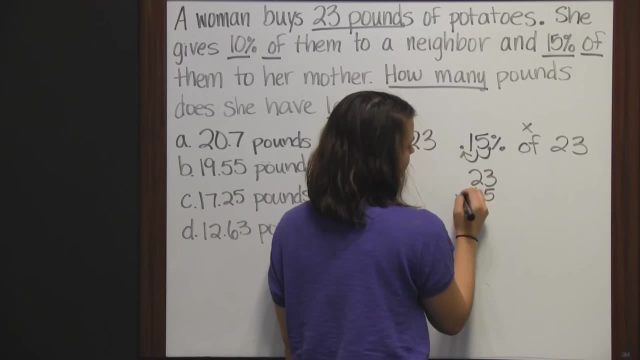 And we have to change our percent to a decimal, Move it two places to the left. So now we're multiplying 23 times 15 hundredths. 5 times 3 is 15.. 5 times 2 is 10, plus 1 is 11.. 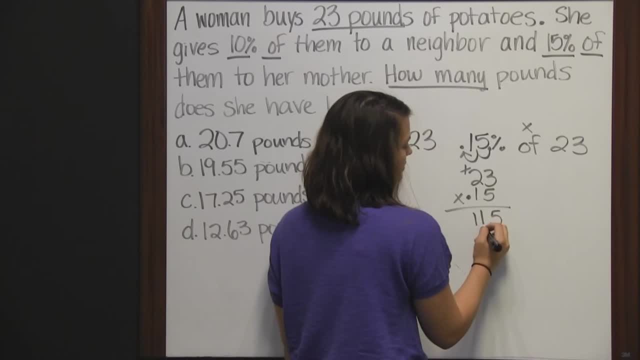 We need to put a 0 placeholder: 1 times 3 is 3, and 1 times 2 is 2.. Then we add these up, We get 5,, 4, and 3.. And then, looking back at those numbers we multiplied together, 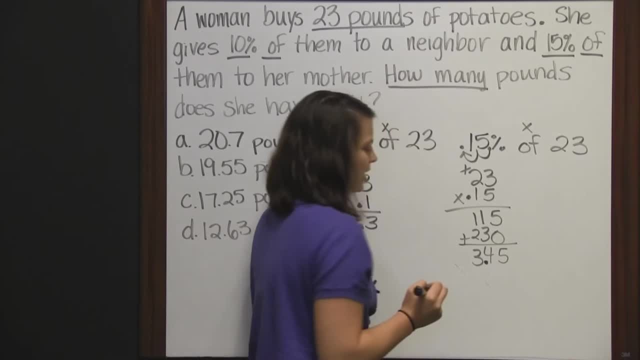 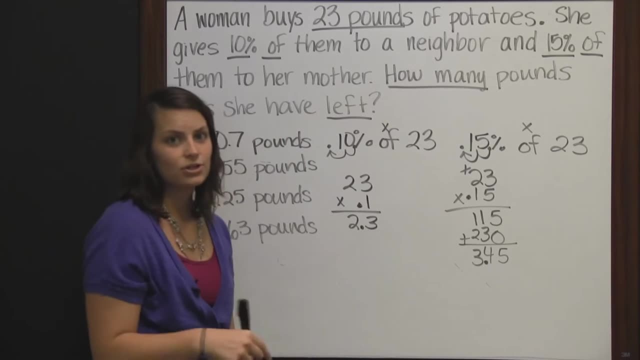 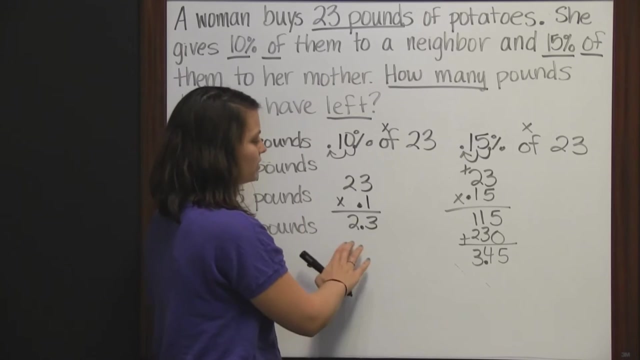 we have two numbers behind the decimal, So our product must have two numbers behind the decimal. which means that she gave 3 and 45 hundredths pounds to her mother. Before we can determine how much she has left, we first need to total up how much she gave away. 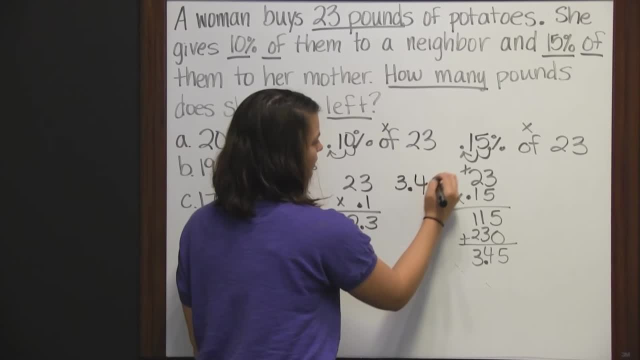 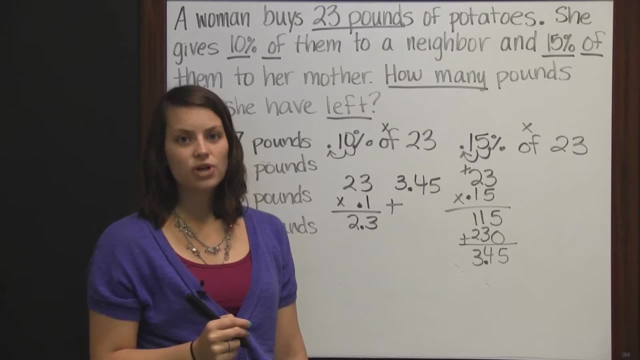 So we're going to take the 3 and 45 hundredths and add the 2 and 3 tenths to it. Remember, when adding or subtracting decimals we have to line up the decimals. So that's 2 and 3 tenths. 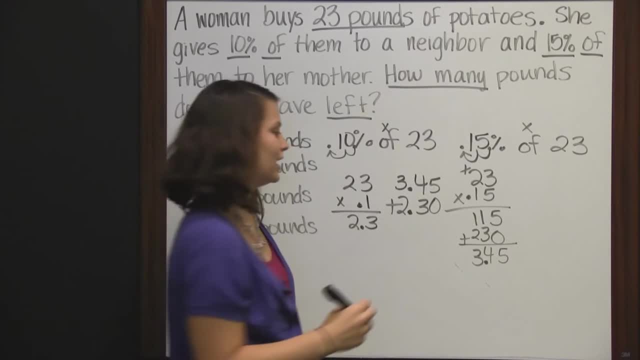 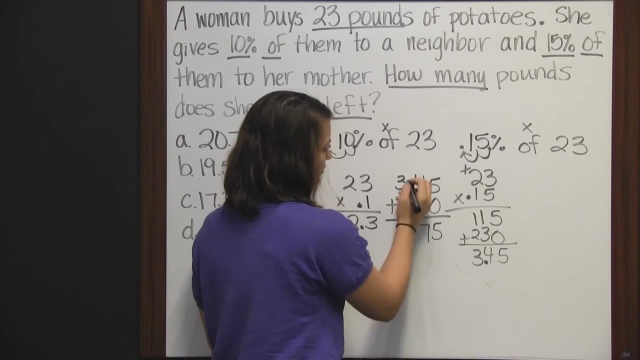 And then you can fill in with as many zeros as needed after the decimal 5 and 3, and 0 is 5.. 4 plus 3 is 7.. Bring down that decimal 3 plus 2 is 5.. 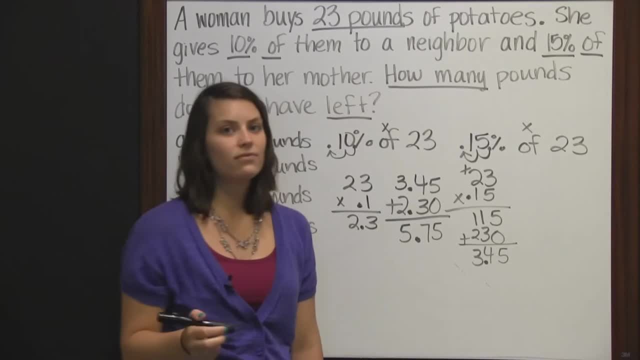 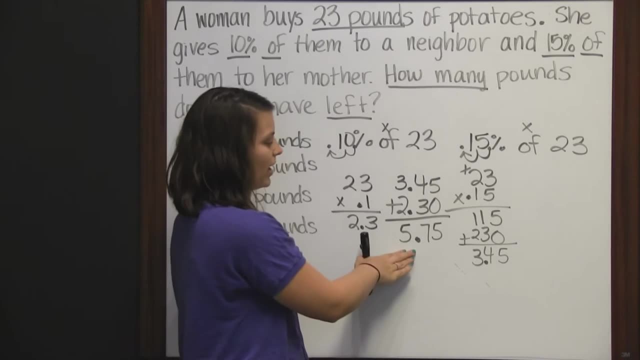 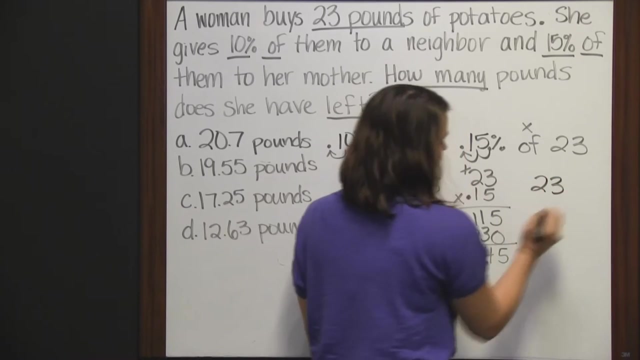 So now we know the total amount that she gave away And using that we can figure out how much she has left after she gave away the 5 and 75 hundredths pounds. So we'll take our 23 pounds and subtract 5 and 75 hundredths pounds. 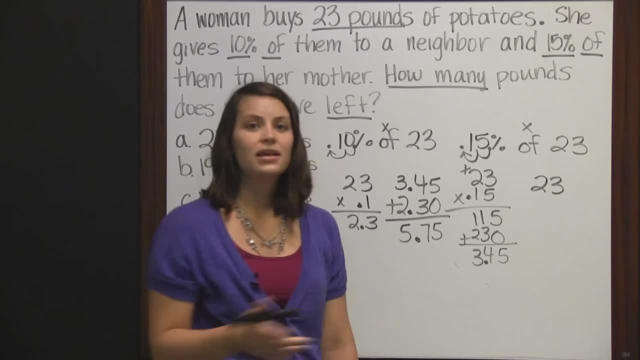 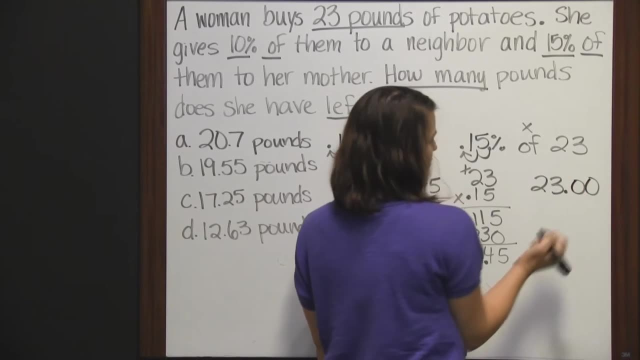 So we're subtracting with decimals, which means we need to line them up, And the decimal in 23 is at the back And we can add two zeros there, because the number doesn't change when you add zeros after the decimal. And then we can subtract the 5 and 75 hundredths. 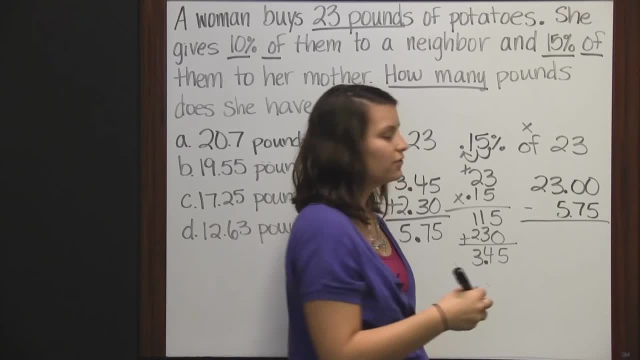 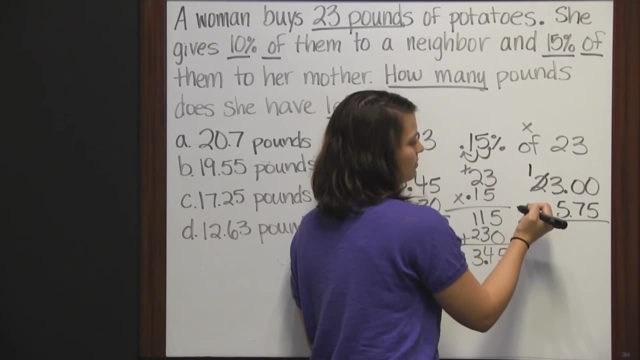 We can't take 5 from 0, or 7 from 0, or 5 from 3.. We're going to have to borrow, starting all the way over here with the 2, and it becomes a 1.. So this is 13,, but we've got to borrow from that. 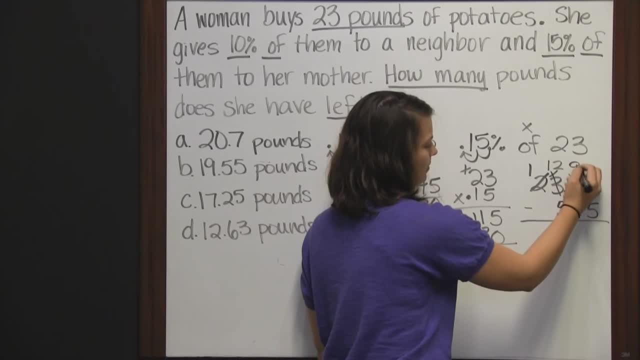 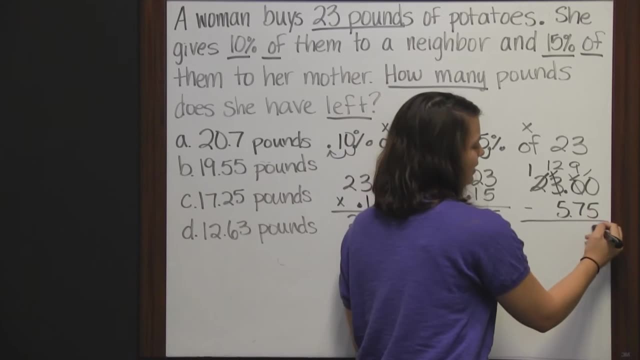 It becomes 12.. 10, but we've got to borrow from that- It becomes 9.. And then, finally, we have a 10 there at the end. So 10 minus 5 is 5.. 9 minus 7 is 2.. 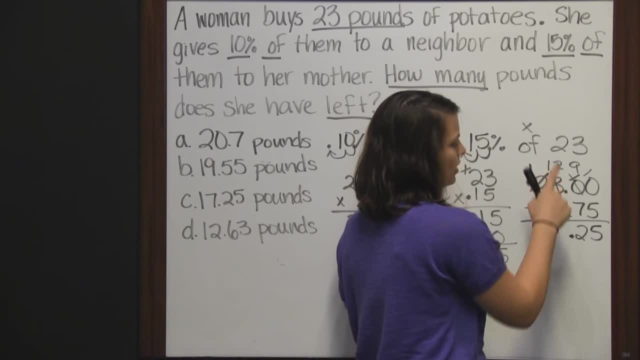 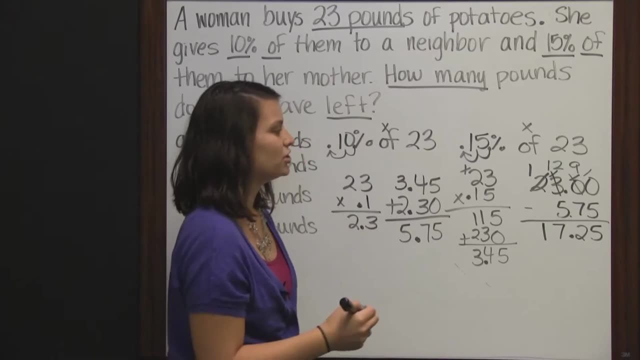 We bring that decimal down: 12 minus 5 is 7. And then we bring down the 1.. So that means that after she gives away the 5 and 75 hundredths pounds to her neighbor and her mom, she's left with 17 and 25 hundredths pounds. 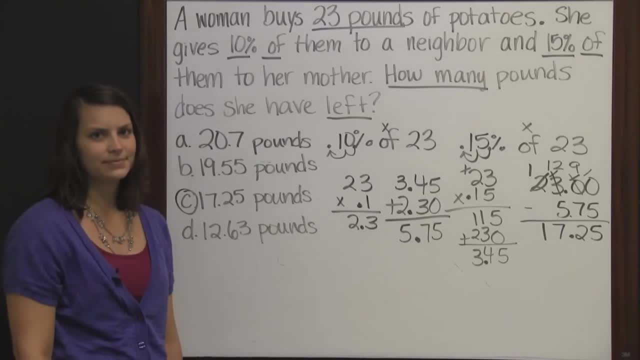 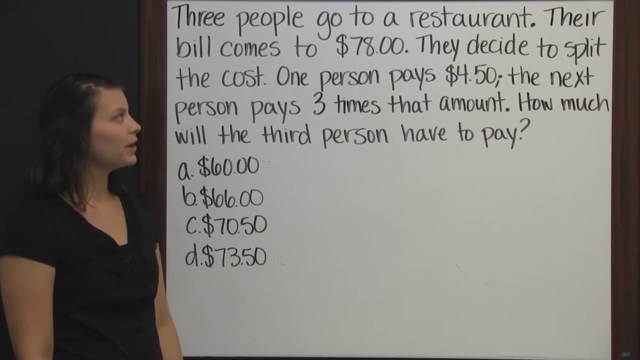 which is answer choice C. Three people go to a restaurant. Their bill comes to $78.. They decide to split the cost. One person pays $4.50.. The next person pays 3 times that amount. How much will the third person have to pay? 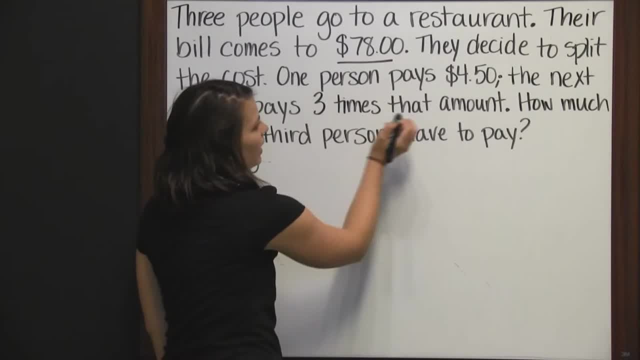 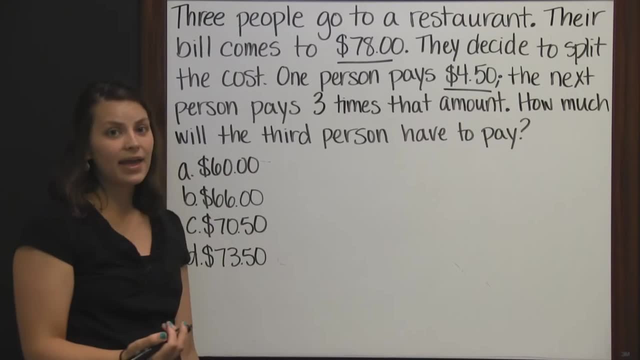 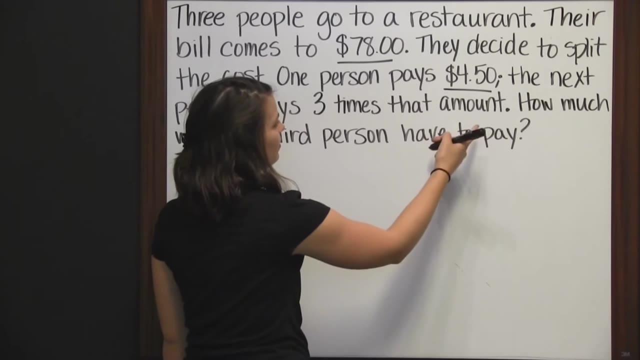 So we know the total and how much one person paid. We're also given an idea and a way to figure out how much the second person paid, So as the next person pays 3 times that amount, 3 times and that amount being $4.50.. 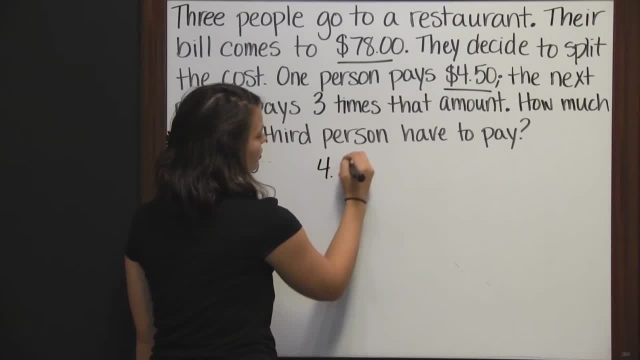 So to figure out how much they paid, we take the $4.50 and multiply it times 3.. 3 times 0 is 0.. 3 times 5 is 15.. So write the 5, carry the 1.. 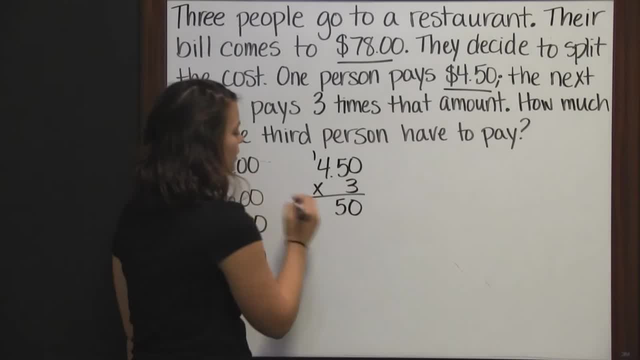 3 times 4 is 12, 12 plus 1 is 13.. Since we have two numbers behind the decimal place here, we have two numbers behind the decimal place in our product, So that means that the second person ended up paying $13.50.. 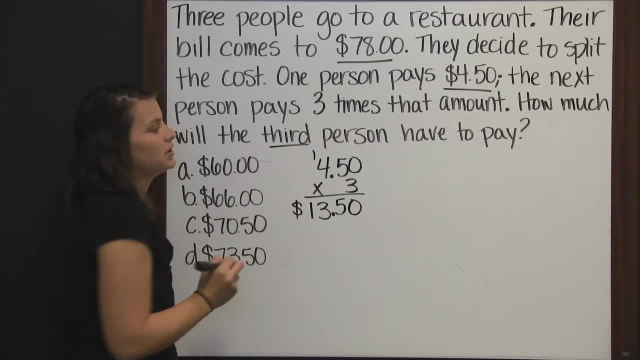 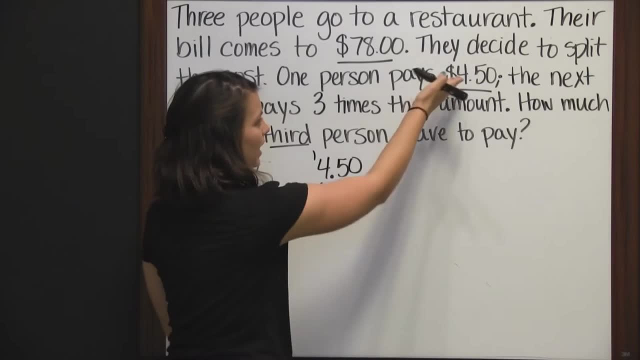 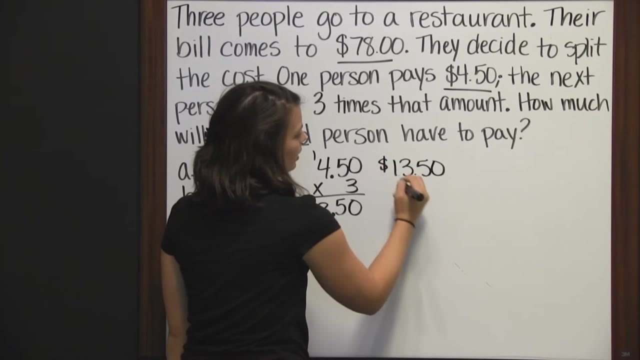 Still, though, that doesn't tell us how much the third person paid. In order to figure that out, we first have to figure out the total that was paid by the first two people, So take $13.50 and add the $4.50.. 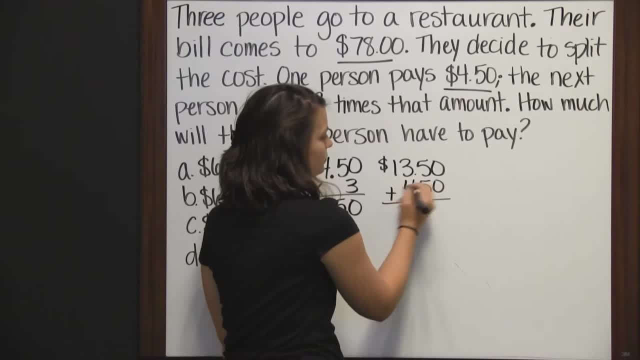 This will give us the total that was already paid. 0 plus 0 is 0.. 5 plus 5 is 10.. So write the 0, carry the 1.. Bring down the decimal to the answer: 4 plus 3 is 7, plus 1 is 8.. 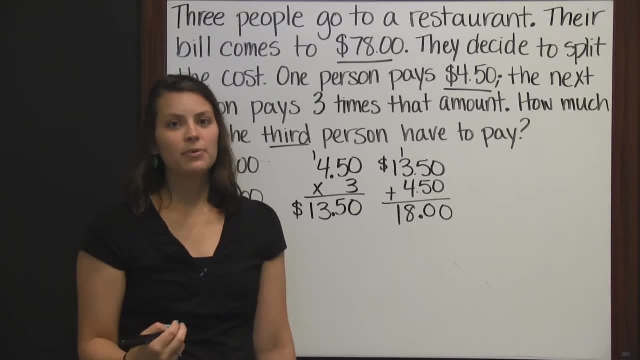 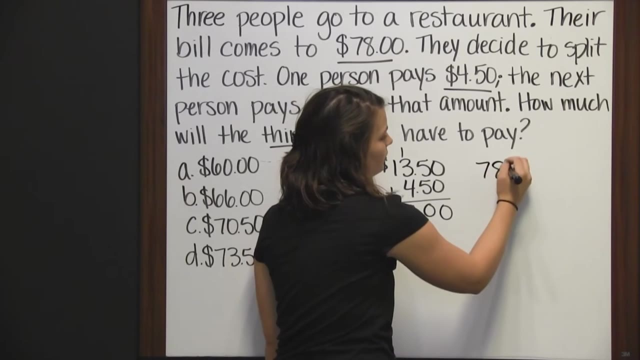 And then we bring down that: 1.. So the first two people paid a total of $18.. And the total bill was $78.. So how much was left for the third person? Well, we just need to take the total: $78,. 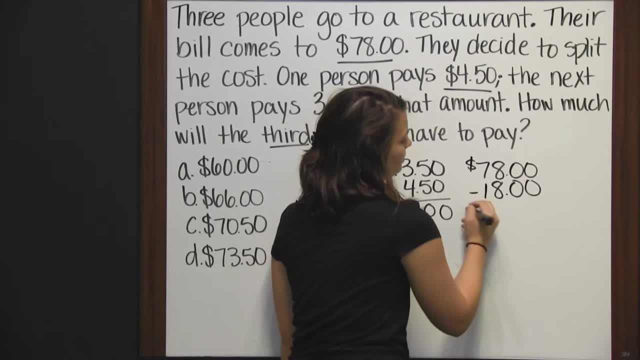 and subtract how much was paid by the first two people. 0 minus 0 is 0.. 0 minus 0 is 0. Bring down the decimal And then 8 minus 8 is 0. And 7 minus 1 is 6.. 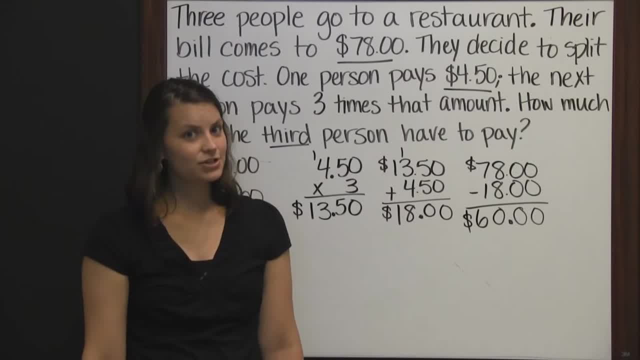 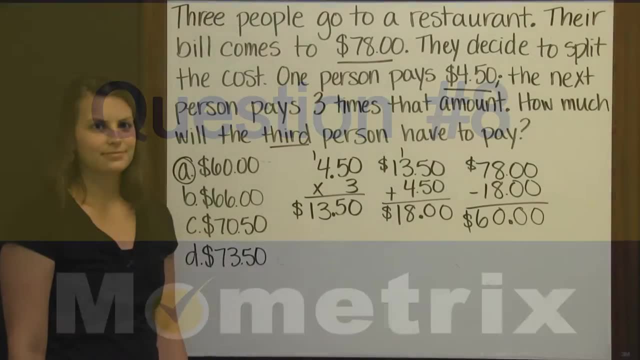 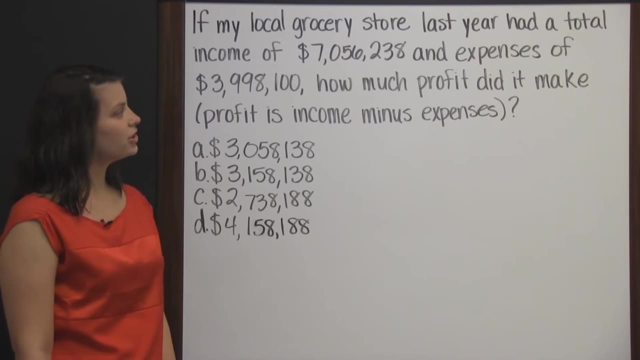 So that means that that third person got the biggest share of the bill. They'll have to pay $60, which is answer A If my local grocery store last year had a total income of $7,056,238 and expenses of $3,998,100,. 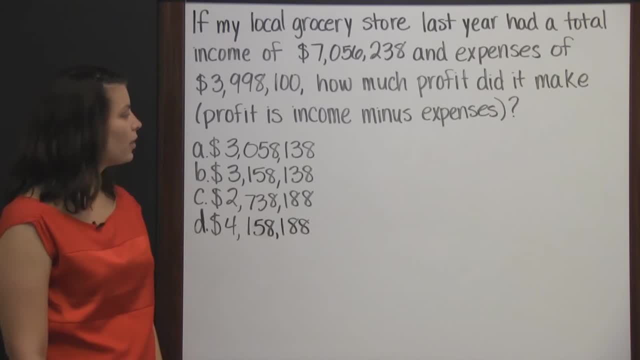 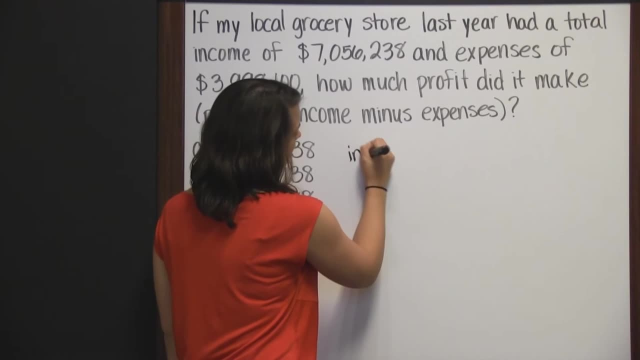 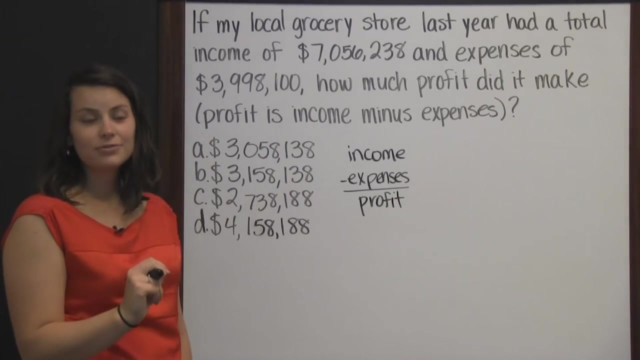 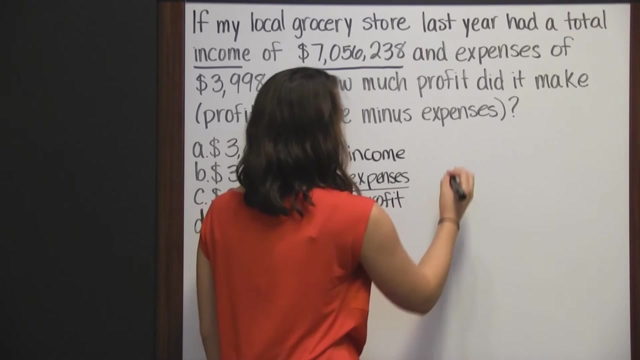 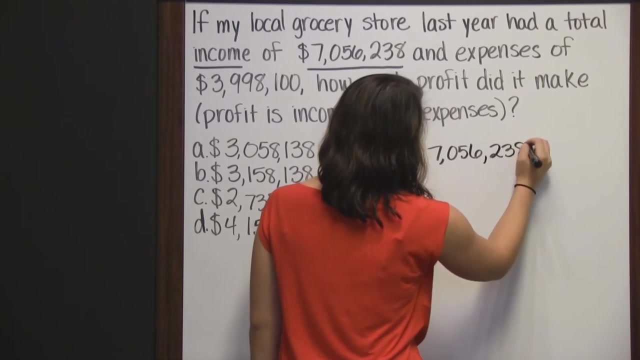 how much profit did it make? Profit is income minus expenses, So that's income minus expenses Equals profit, Which is what I'm trying to find. So that's exactly what I need to do. I need to take my income of $7,056,238. 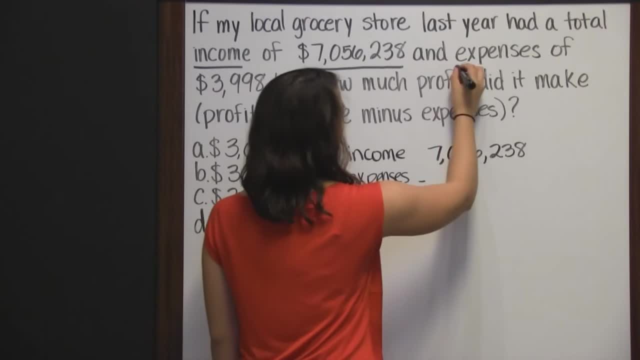 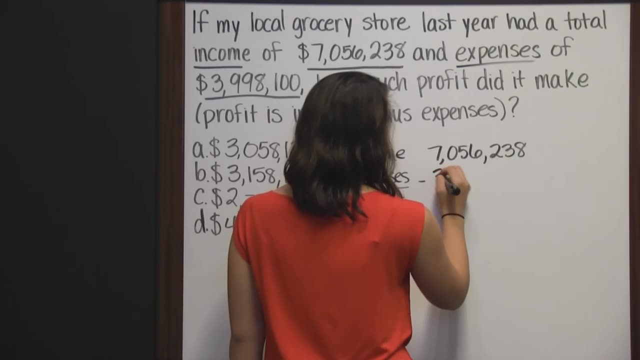 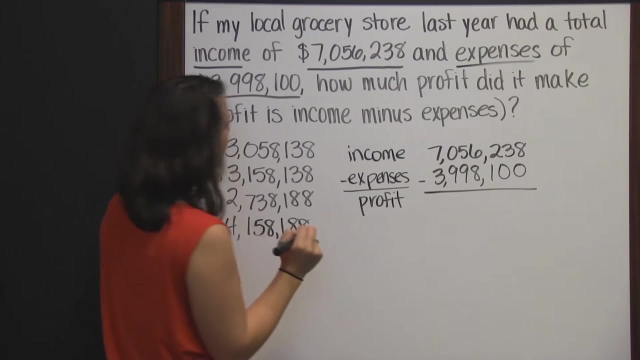 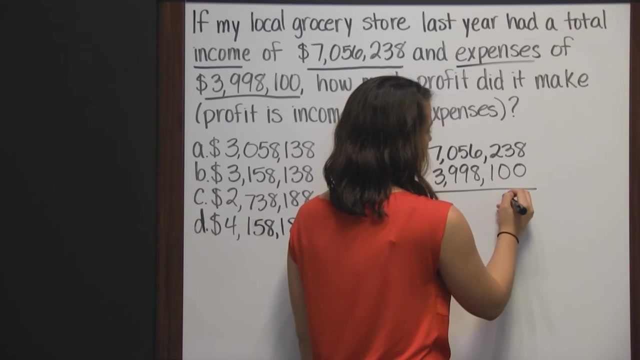 and subtract my expenses of $3,998,100, $3,998,100. And that will give me my profit. So I have: 8 minus 0 is 8.. 3 minus 0 is 3.. 2 minus 1 is 1.. 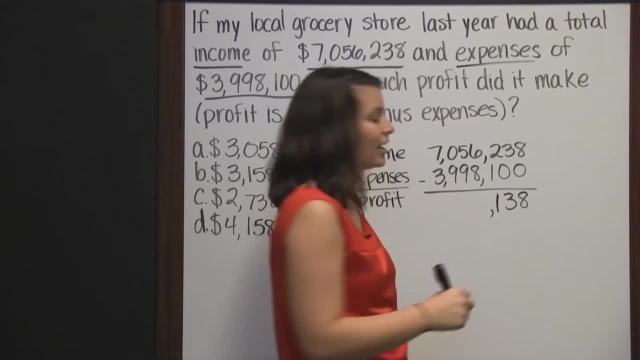 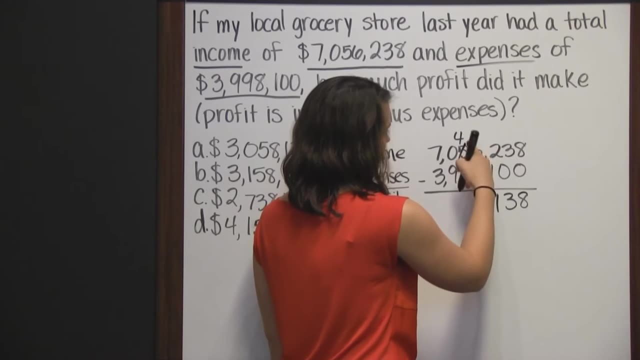 And I'll just bring that comma down, And I can't take 8 from 6, so I'm going to need to borrow from the 5.. It becomes a 4.. So 16 minus 8 is 8., And I can't take 9 from 4.. 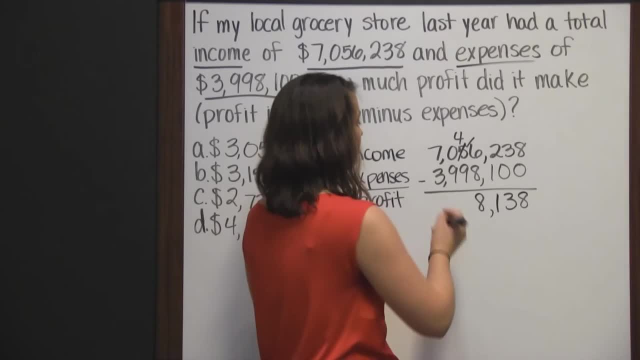 But I also can't borrow from the 0.. It can't get any lower, So I'm going to borrow from the 7.. It becomes a 6. And this is a 10. But I borrow from it. It becomes a 9.. 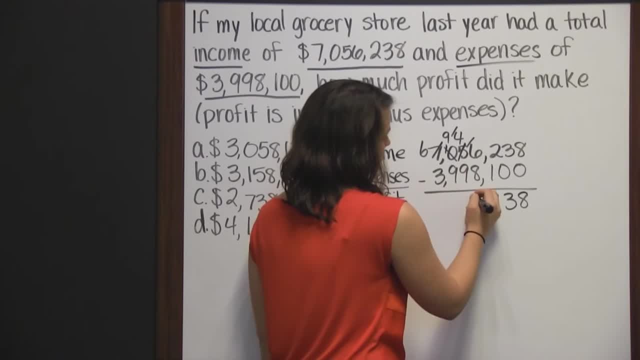 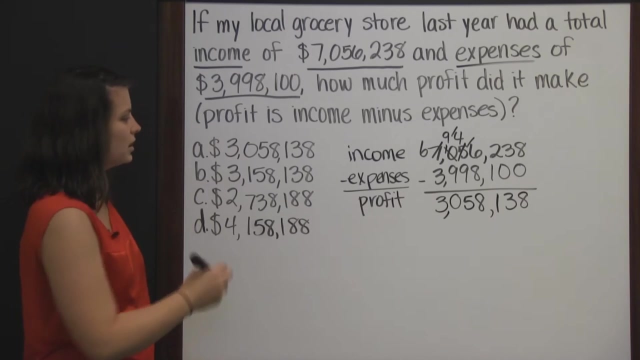 So I have 14 minus 9,, which is 5.. 9 minus 9 is 0., And 6 minus 9 is 1., And 6 minus 3 is 3.. So $3,058,138,. 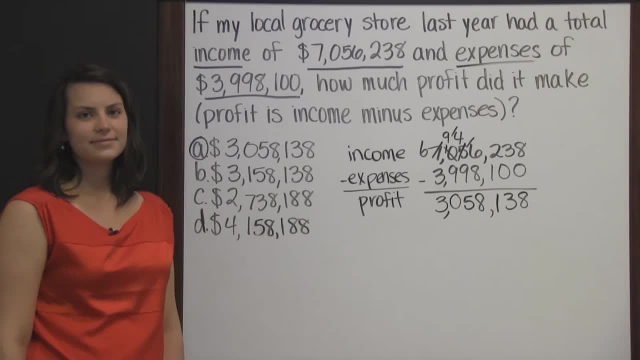 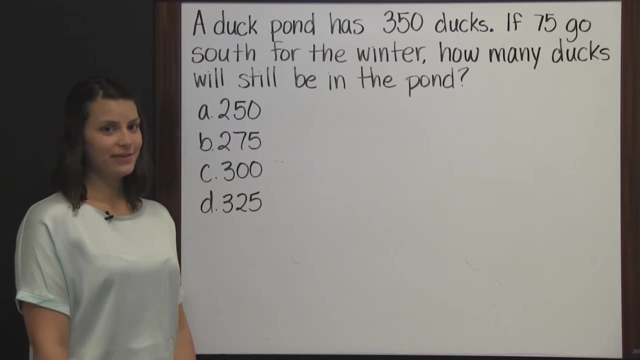 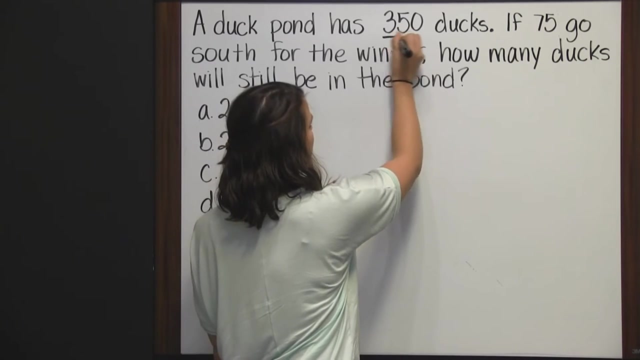 which would be answer A. A duck pond has 350 ducks. If 75 go south for the winter, how many ducks will still be in the pond? This is a subtraction problem. We're starting with 350 ducks and 75 leave. 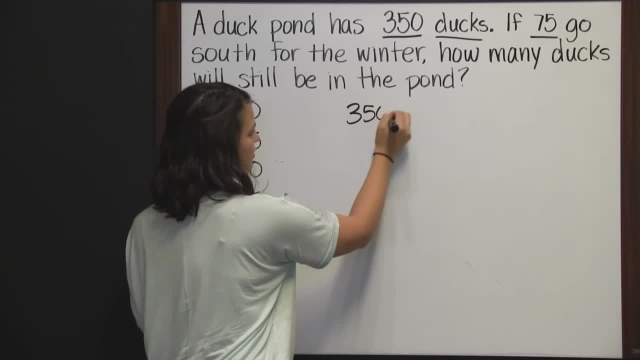 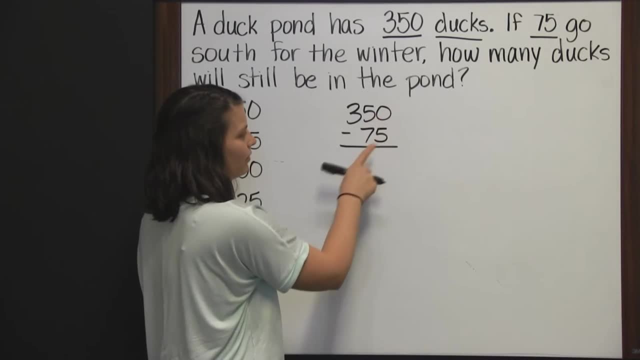 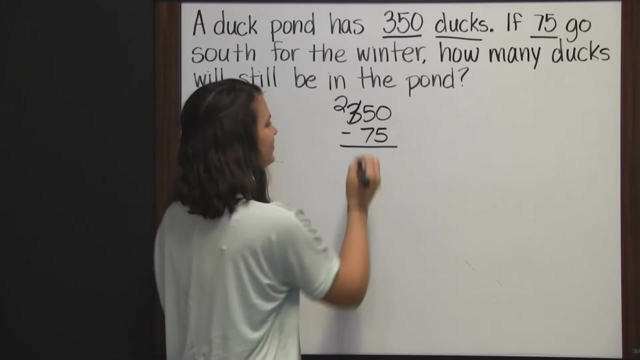 So we start with our 350 ducks and we take away the 75 ducks that left. We can't take 5 from 0 or 7 from 5.. So we start from borrowing from our 3. And it becomes a 2.. 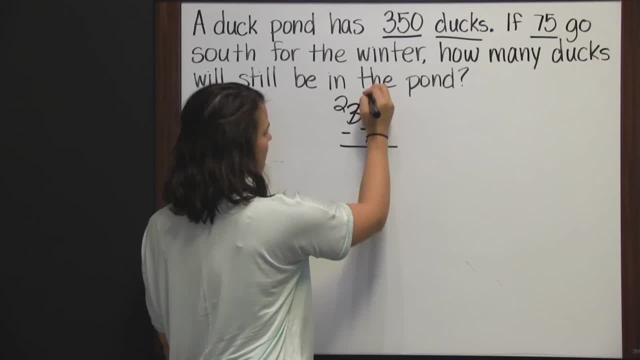 So we put our 1 here 15. But we're going to borrow from 15. So it is now 14. So that we can make 10 for our last number. So we can take 5 from 10 and get 5.. 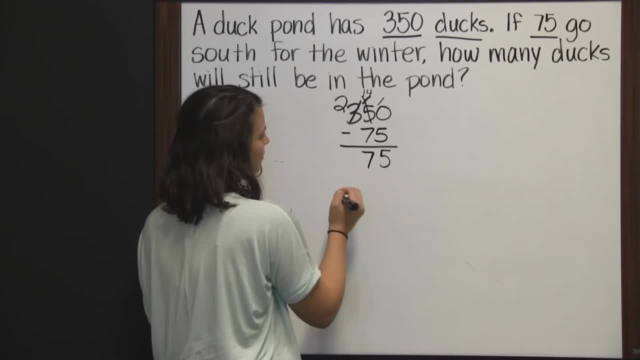 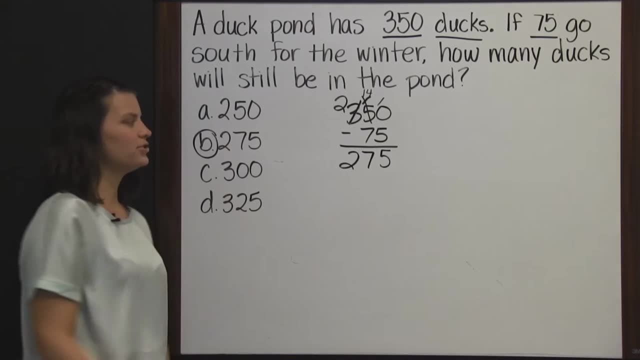 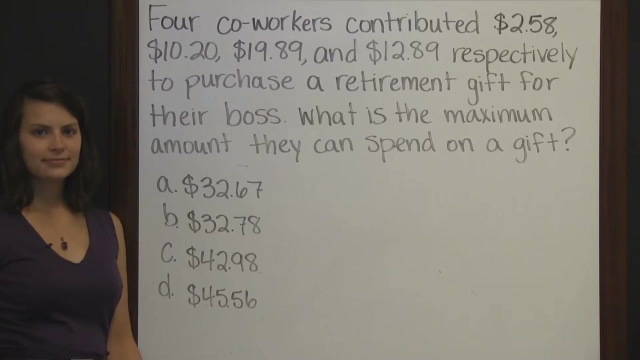 14 minus 7 is 7.. And we bring down our 2.. 2 minus nothing is 2.. So that means there are B 275 ducks left in the pond after the 75 go south for the winter. Four coworkers contributed. 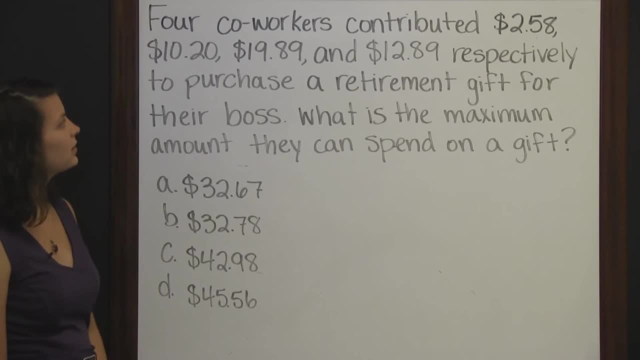 $2.58,, $10.20,, $19.89, and $12.89, respectively- to purchase a retirement gift for their boss. What is the maximum amount they can spend on a gift? So they're putting all of their money together. 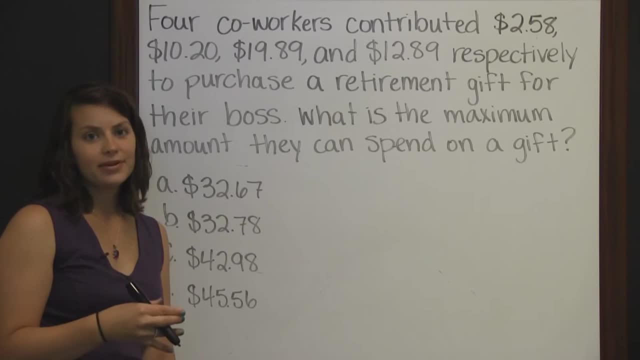 which means we're going to add it all up in order to figure out the maximum amount that can be spent on a gift, And you can add these in any order you want, Because when adding order doesn't matter. So I'm going to start with the biggest number. 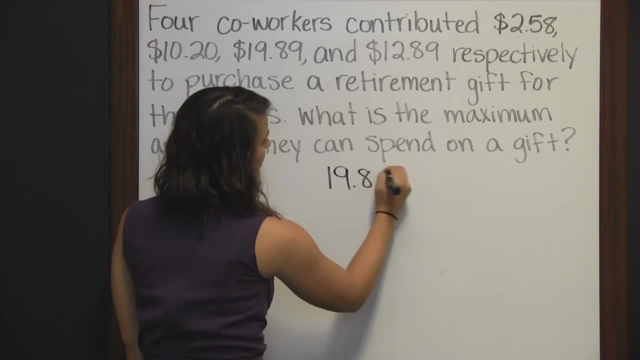 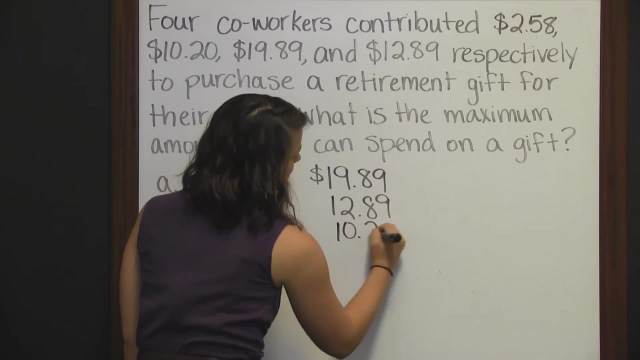 $19.89. And under that I'm going to put the next biggest, $12.89. And then below that I'll put $10.20. And then finally $2.58. And again we're trying to find a total. 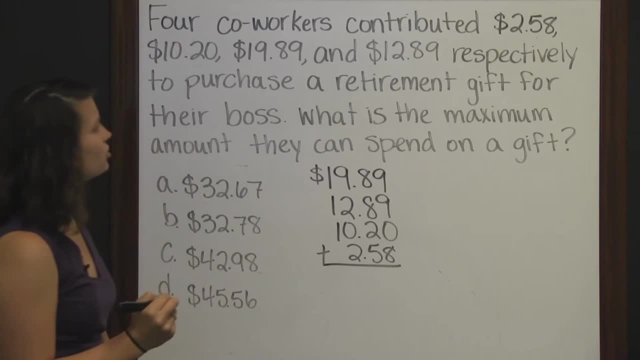 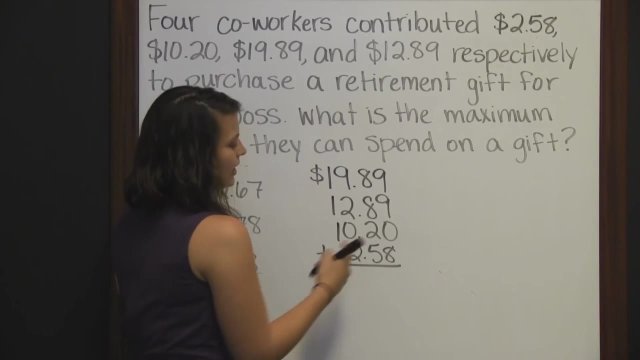 So we're just adding those four contributions up. 9 plus 9 is 18.. 18 plus 8 is 26.. Write the 6,, carry the 2.. 2 plus 8 is 10.. And again, 8 plus 2 is 10.. 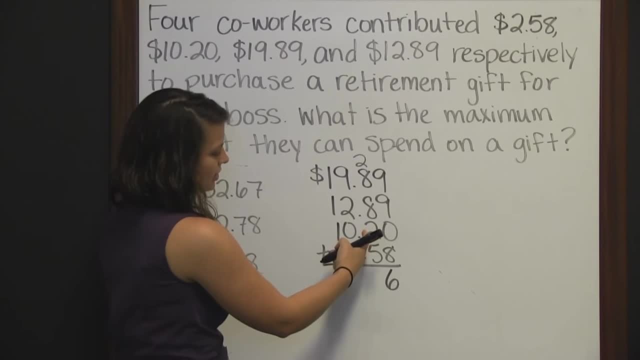 So we have 10 and 10,, which is 20.. And 20 plus 5, 25.. So write the 5 and carry the 2.. Then we have 9 and 2, 4, 6. So 9 plus 6 is 15.. 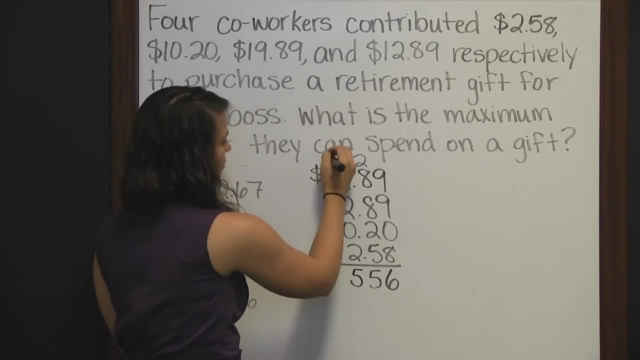 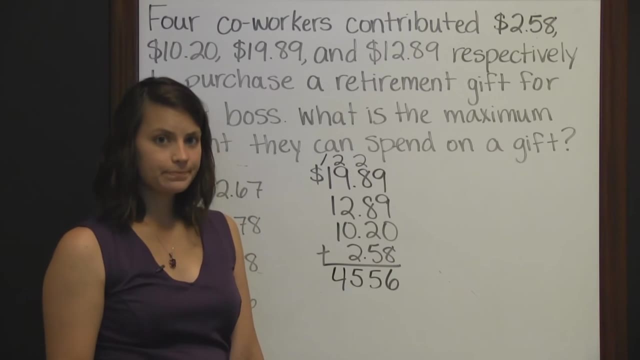 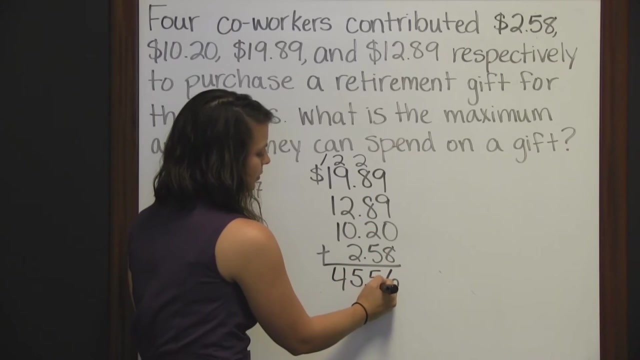 So write the 5.. Carry the 1.. 1,, 2,, 3,, 4.. And where does that decimal go? Well, remember, when adding you must line up the decimal, which we did, and you just bring it down into your answer. 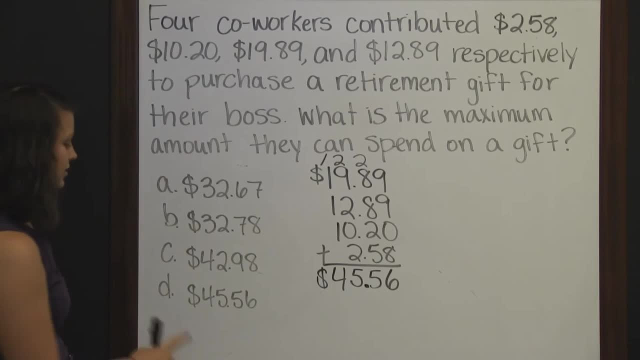 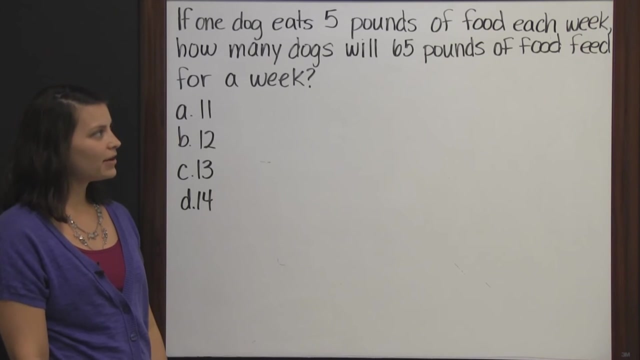 So we have $45.56, which would be answer choice D. That's the maximum amount of money that can be spent on a gift. If one dog eats 5 pounds of food each week, how many dogs will 65 pounds of food feed for a week? 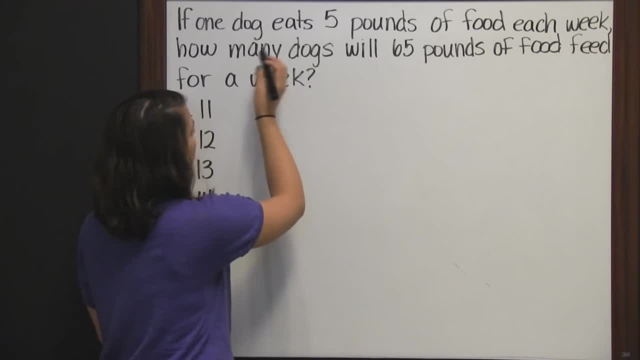 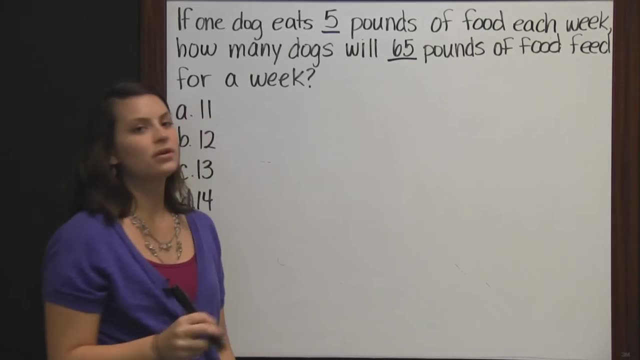 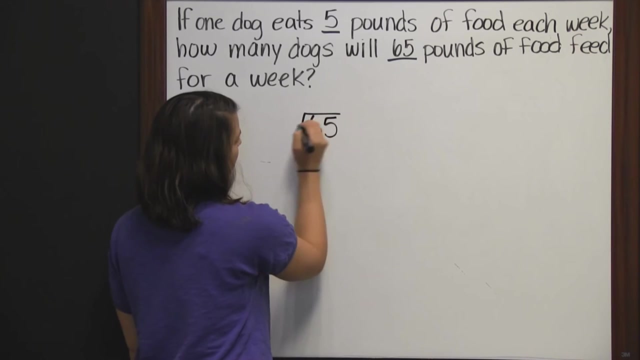 So we know that one dog eats 5 pounds of food in a week. If we have 65 pounds of food, how many dogs can we feed? We just need to take the 65 pounds of food and divide it by 5, since each dog requires 5 pounds of food. 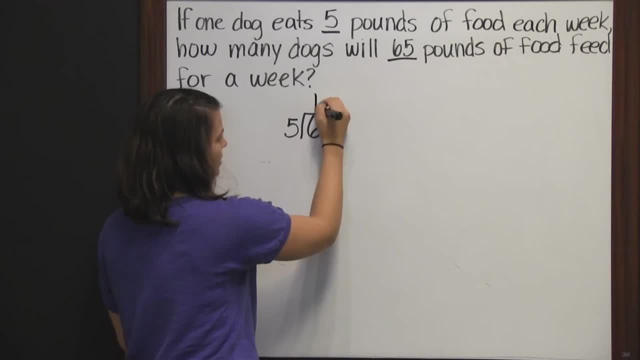 5 goes into 6 one time. 5 times 1 is 5.. Subtract and we get 1.. And then we bring down the 5.. 5 goes into 15. three times 5 times 3 is 15.. 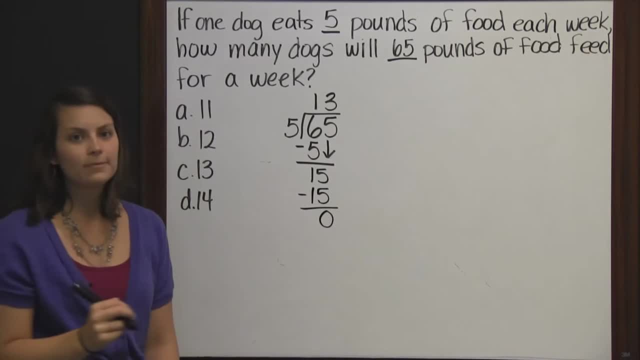 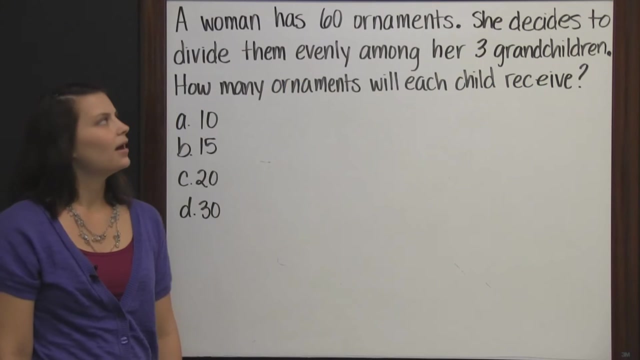 We subtract and we get a 0 right away And we get a 0 remainder. So that means that 13 dogs can be fed the 5 pounds a week. which is answer choice C. A woman has 60 ornaments. She decides to divide them evenly. 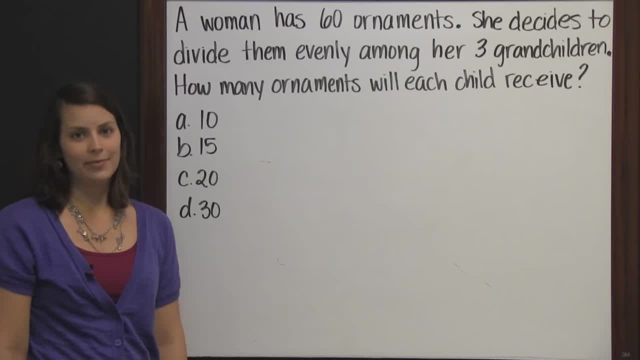 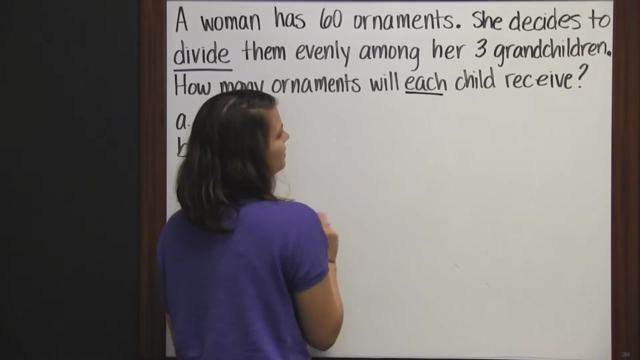 among her three grandchildren. How many ornaments will each child receive? Well, they gave us a big clue on what to do here, since it says divide. So to find out how many ornaments each child will receive, we need to take our total number of ornaments. 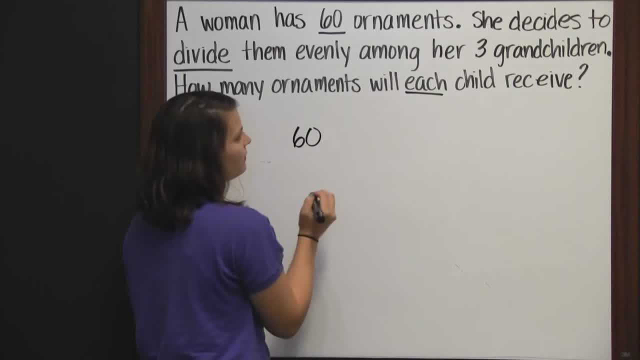 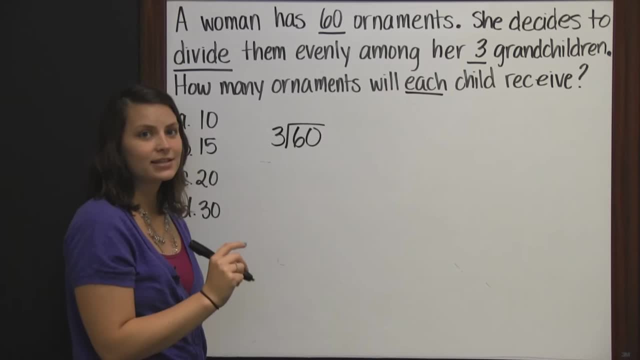 60, and divide that by how many grandchildren she has, 3 goes into 6. two times 3 times 2 is 6.. If we subtract we get 0. And then we bring down 0. And 3 goes into 0, zero times. 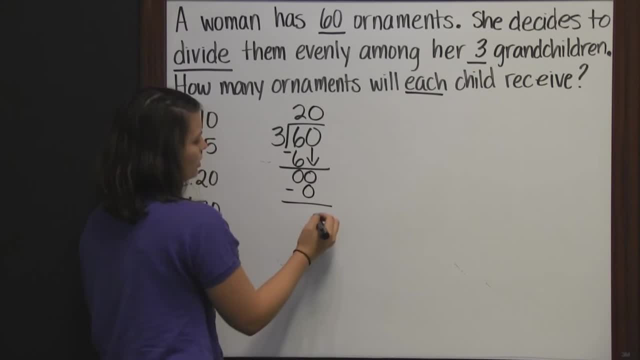 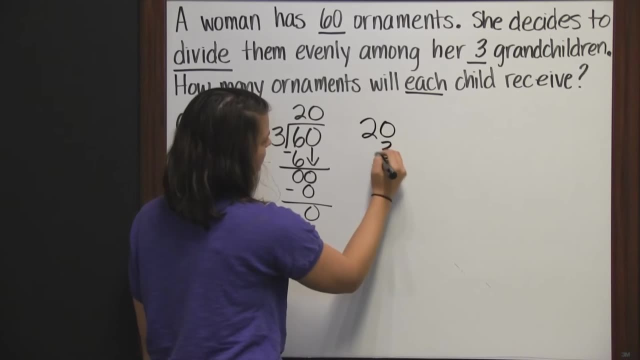 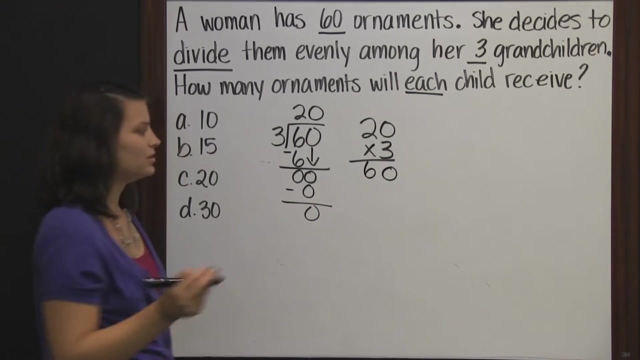 And 3 times 0 is 0. And you subtract and get 0.. We can check this by multiplying 20 times 3.. 3 times 0 is 0. And 3 times 2 is 6. And we do in fact get 60.. 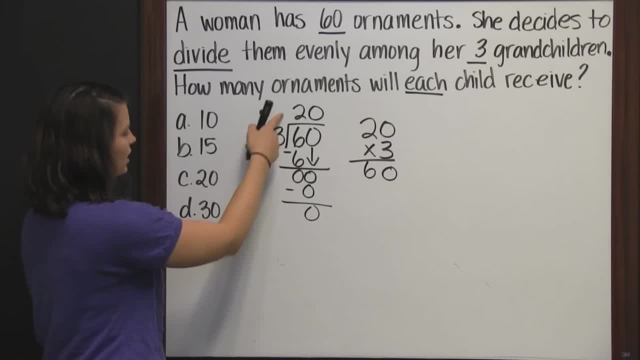 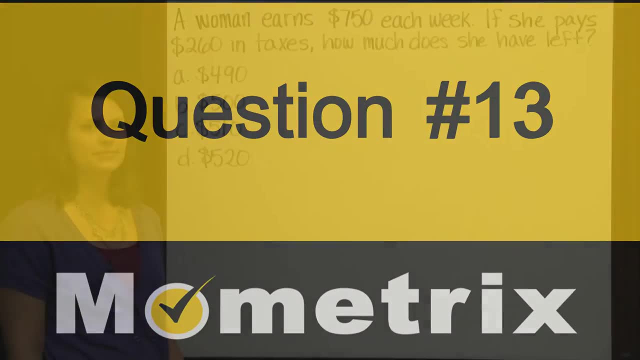 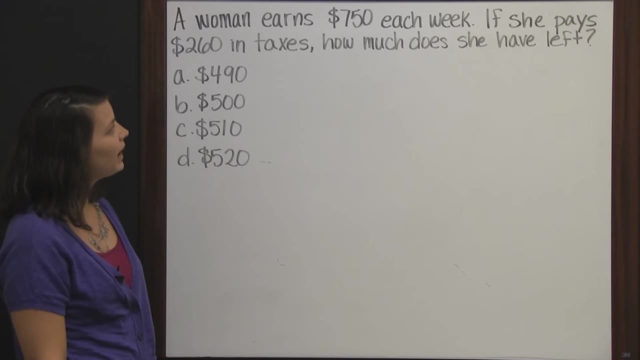 So that means that each one of her grandchildren is going to get 20 ornaments? which is answer? choice C. A woman earns $750 each week. If she pays $260 in taxes, how much does she have left? Now? this phrase right here. 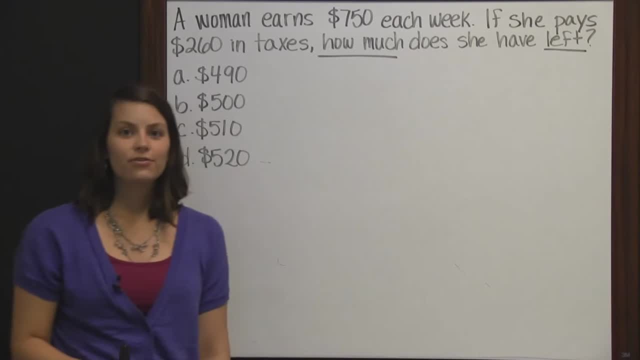 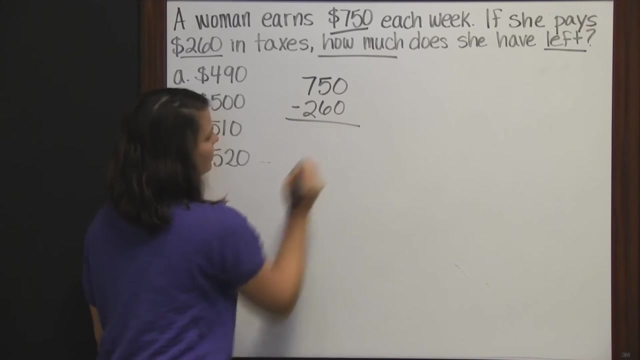 how much is left, tells you that you need to subtract. She gets paid $750, but taxes that's money that's taken out of her check. So we need to subtract 260 from 750.. 750 minus 260.. 0 minus 0 is 0. 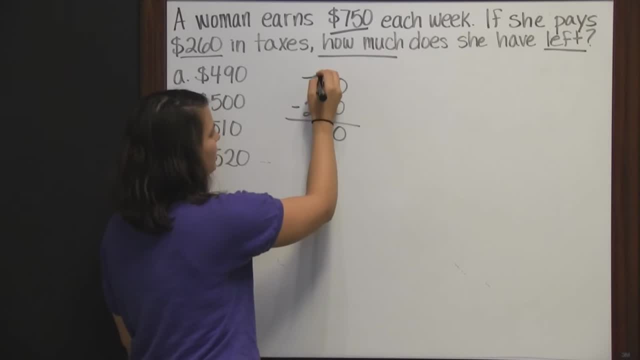 We cannot take 6 from 5.. So we need to borrow from the 7.. It becomes a 6.. And then we have 15 here. 15 minus 6 is 9. And 6 minus 2 is 4.. 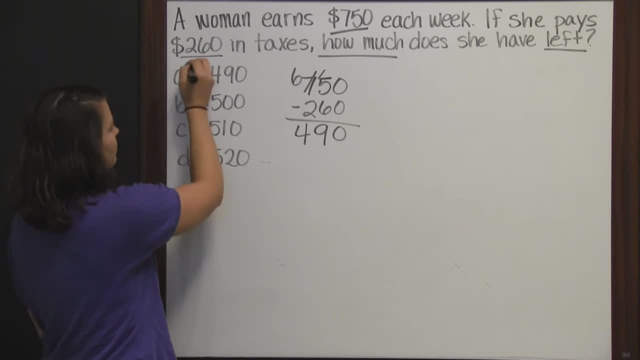 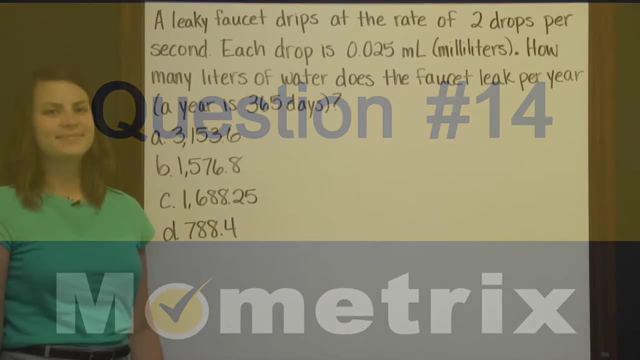 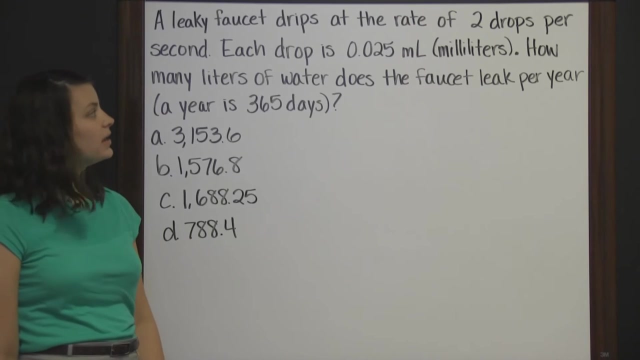 So that means after the taxes are taken out, she's left with $490.. And that's $570.. So let's see this question here: How much time does it take for a faucet to leak water? If I'm lucky enough to gon' prevent a water leak? 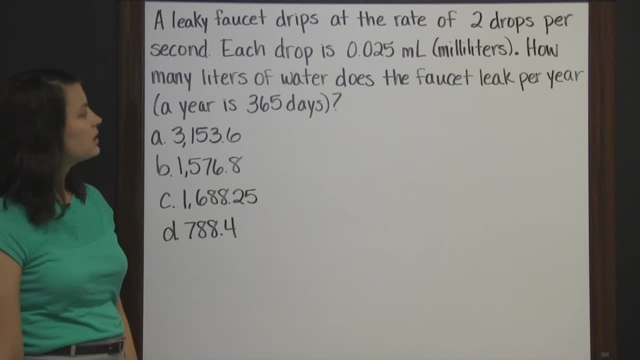 I'm gonna drop a 6 on top of it, because it's $5. So I'm gonna drop a 6.. Now you may be wondering why is it so difficult to do this? We can use the air purifier system. 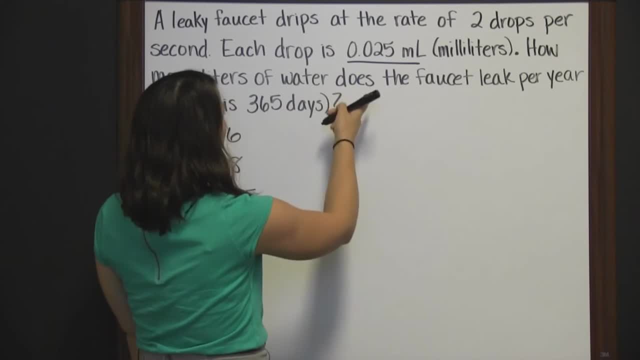 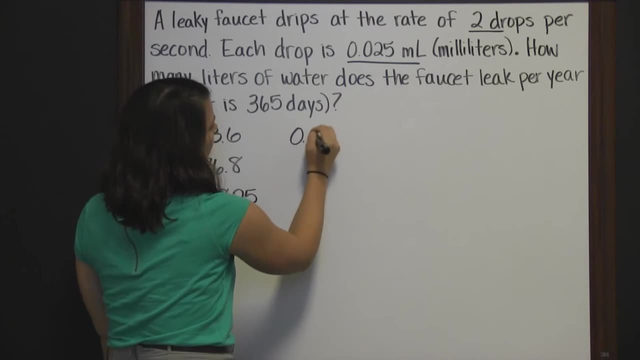 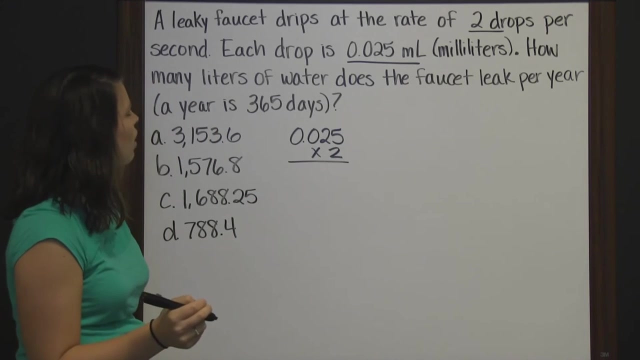 to do the work because it says it drips at a rate of 2 drops per second, but each drop is 0.025 milliliters, so I need to multiply that times 2 to figure out how much water is in drips each second. 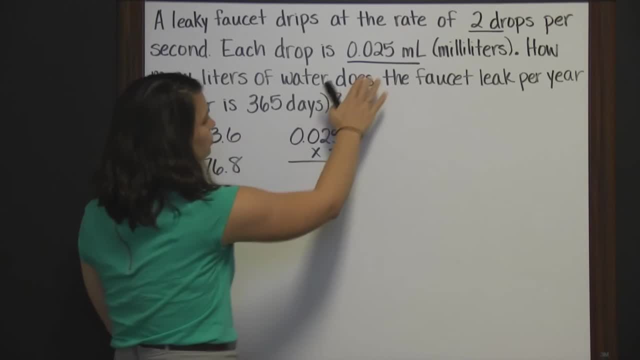 because it drips 2 drops per second. so 2 drops. I need to multiply 0.025 times 2.. 2 times 5 is 10, carry the 1. 2 times 2 is 4, plus 1 is 5.. 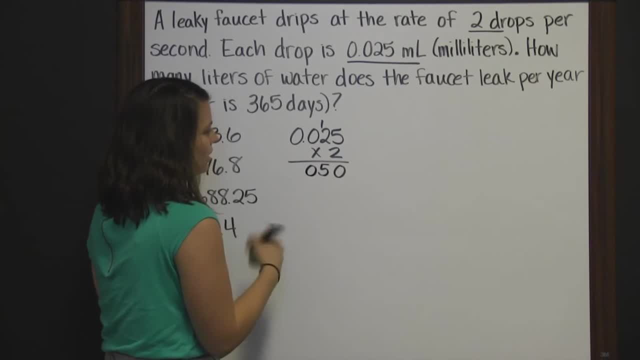 2 times 0 is 0, and obviously 2 times 0 again would be 0.. We have 1,, 2,, 3 numbers behind the decimal, so our answer should also have 3 numbers behind the decimal. Really, we can get rid of this 0, it's unnecessary. 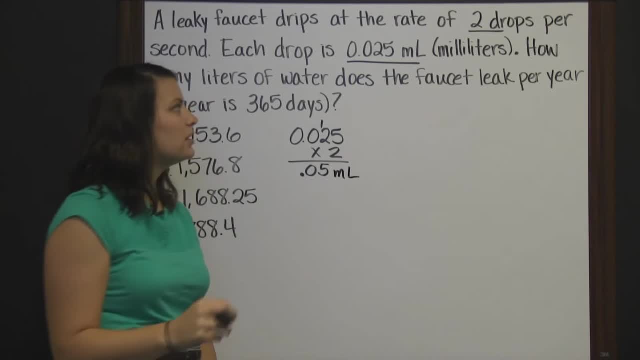 So it's 5 hundredths milliliters of water drips out each second. So it's 5 hundredths milliliters of water drips out each second. So it's 5 hundredths milliliters of water drips out each second. 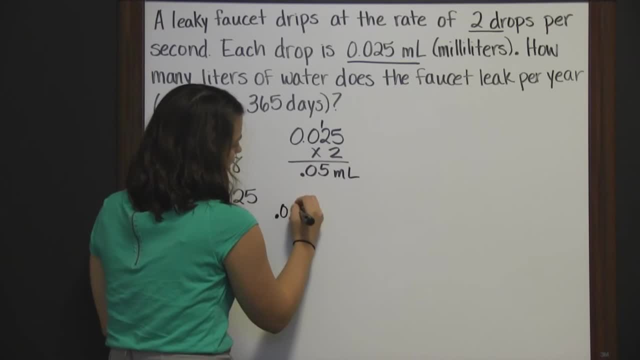 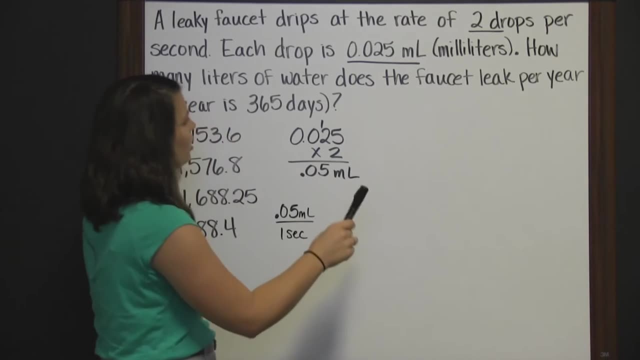 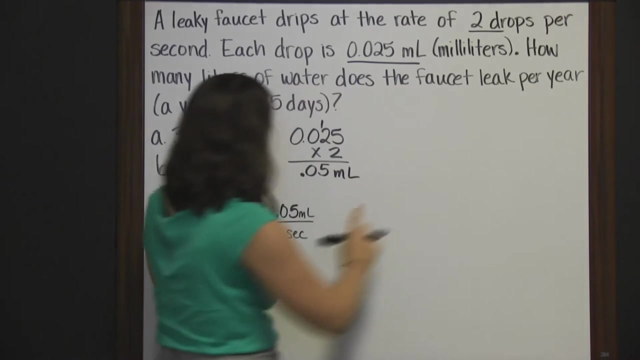 So that's 1 second, So 5 hundredths milliliters per 1 second. But they want to know how much in liters and we're going to convert that in just a minute. leak out per year, So I need to convert from seconds to years. 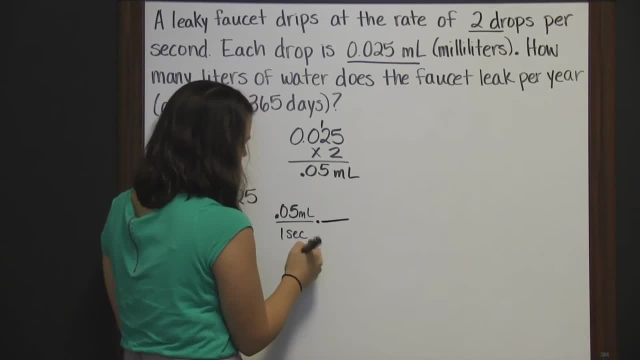 and I'm going to do that by multiplying by conversion factors. So if I have seconds in my denominator, then I need to have seconds in my numerator, and I know that 60 seconds is 1 minute. Now, the reason I put seconds in these diagonal positions is that we're multiplying fractions. 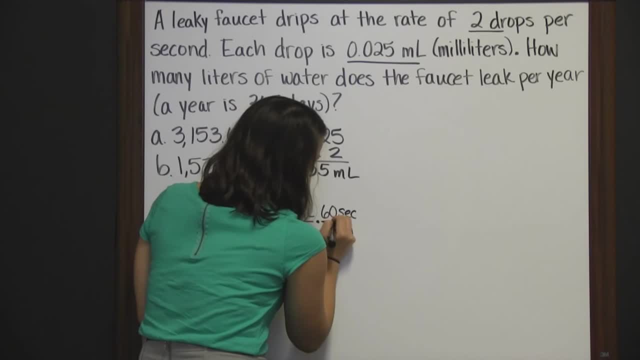 and so those units will cross-cancel. So I'm going to continue on converting. so I've converted now from seconds to minutes. So now I need to do the same thing with minutes, so minutes in my numerator, and I'm going to convert minutes into hours. 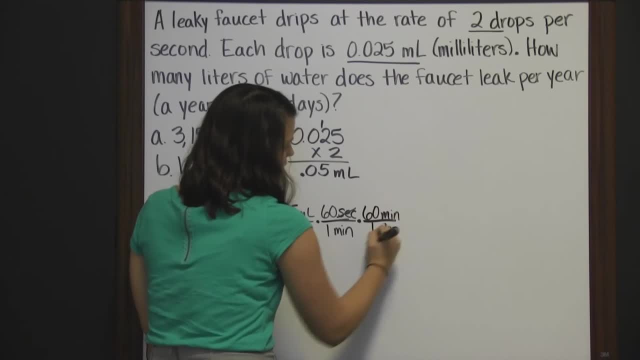 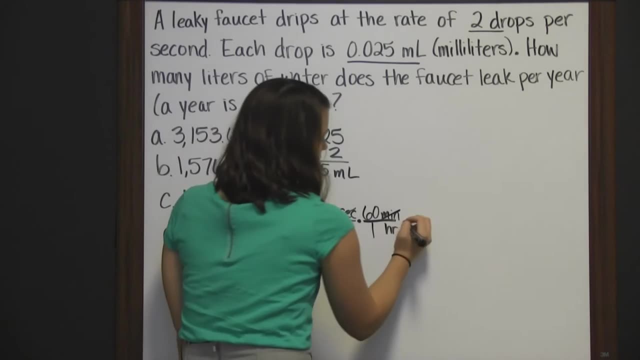 and I know that 60 minutes makes 1 hour. So now see my minutes again are in those diagonal positions so I can cross-cancel them. I need to continue on converting. so now hours needs to go in the numerator and I'm going to convert hours to days or day. 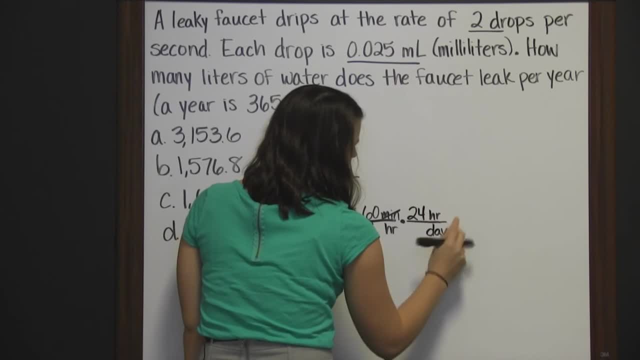 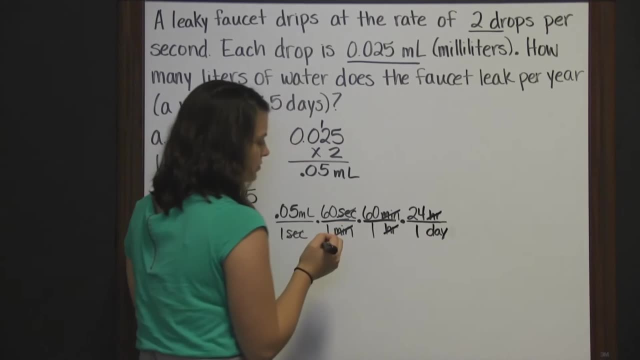 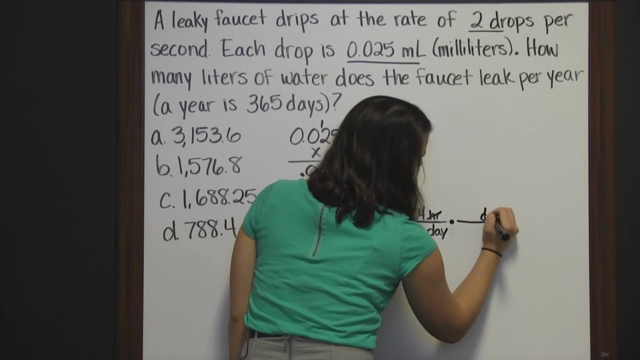 I know that there are 20 minutes. I know that there are 24 hours in 1 day, So my hours cross-cancel and I've converted now into days, so I'm almost there per year, so now I need to multiply times. how many days are in a year? 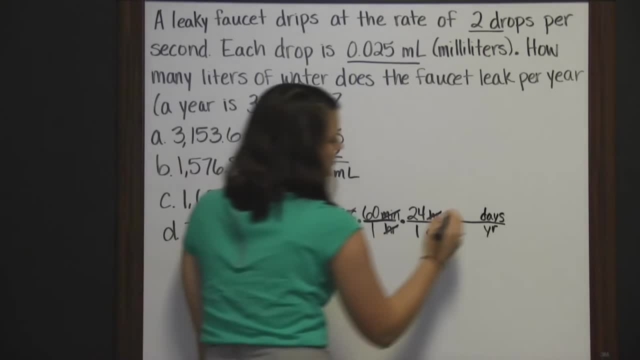 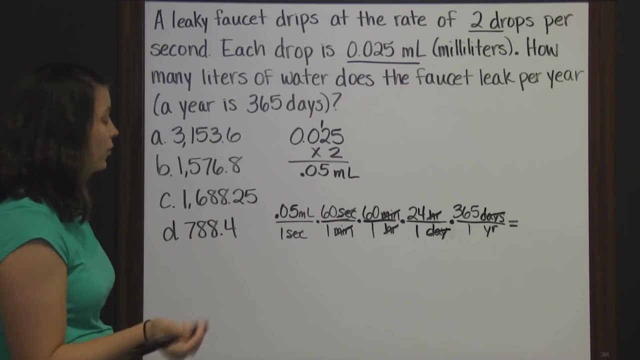 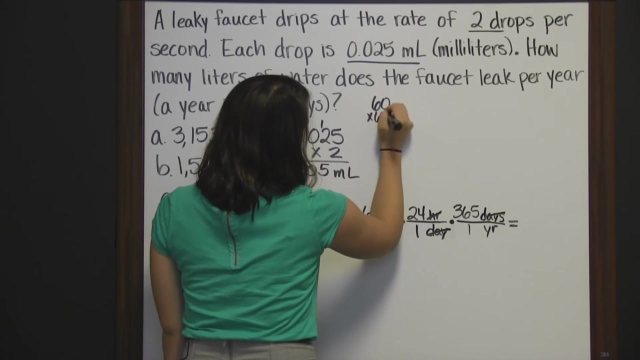 And that one. they told us 365 days in 1 year. Whew, So I have a lot to multiply. I cross-cancel these days So we can start anywhere. Say, we could multiply 60 times 60 first, So 60 times 60, 0. 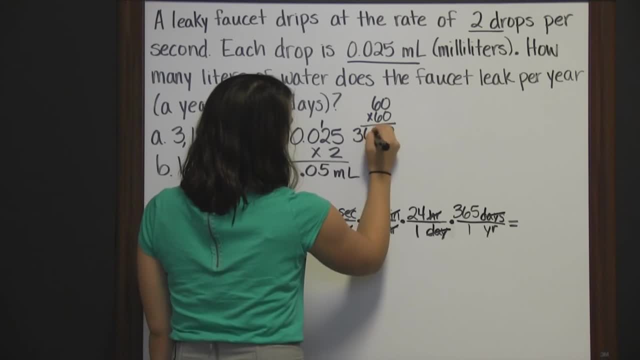 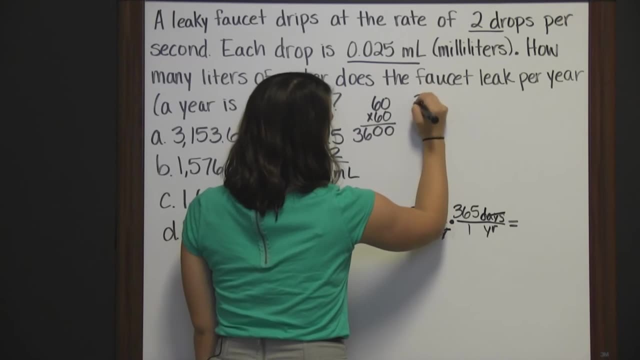 6 times 0 is 0.. 6 times 6 is 36.. So 3,600.. And then maybe multiply that times 24.. 3,600 times 24.. 4 times 0 is 0.. 4 times 0 is 0.. 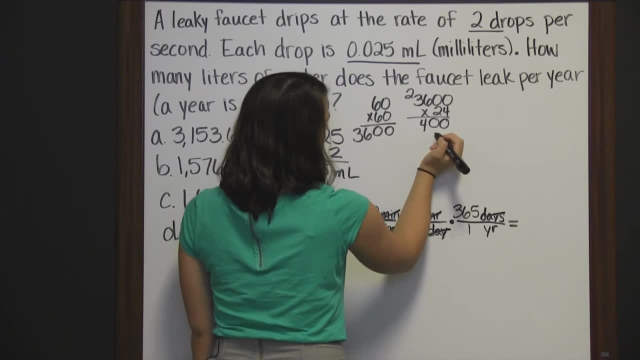 4 times 6 is 24.. Carry the 2.. 4 times 3 is 12.. 13,, 14.. Put a 0 placeholder for the 4, and move on to the 2.. 2 times 0 is 0.. 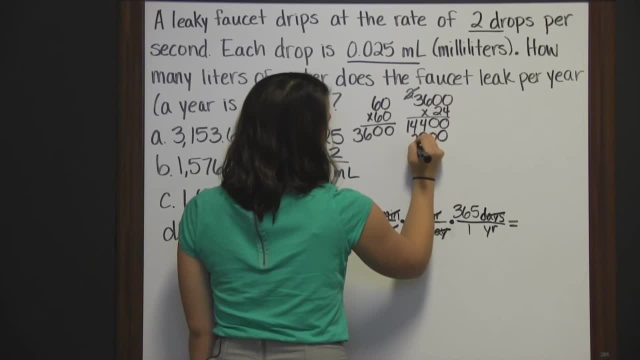 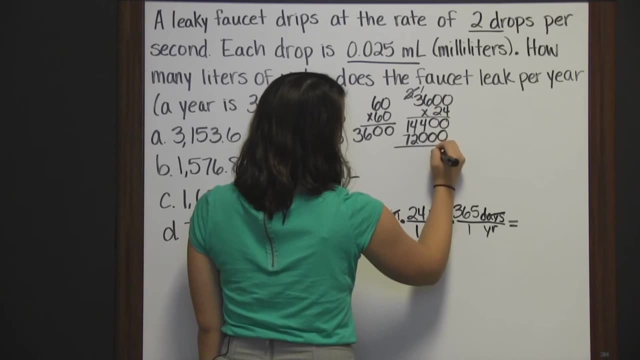 2 times 0 is 0.. 2 times 6 is 12.. Carry the 1. And 2 times 3 is 6, plus 1 is 7.. Add up your 0s: 4 plus 0 is 4.. 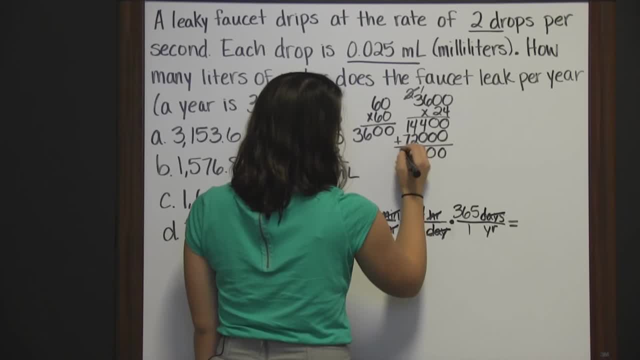 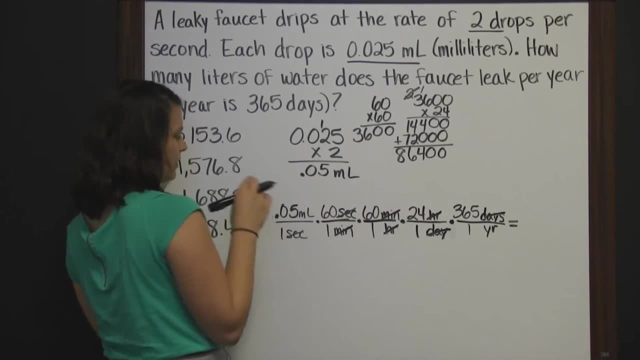 4 plus 2 is 6.. 1 plus 7 is 8.. Okay, so so far I've multiplied 60 times 60 times 24.. We can go ahead and take this number and multiply it times our 5 hundredths. 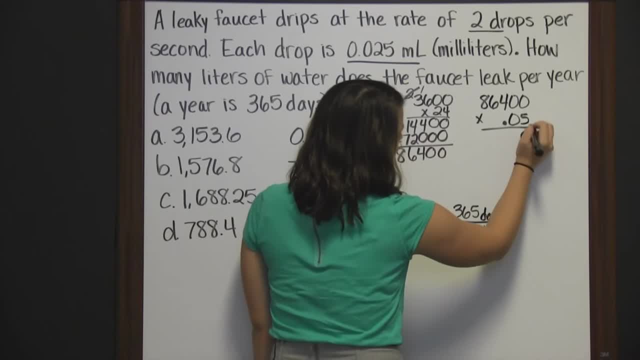 So 5 times 0 is 0.. 5 times 0 is 0.. 5 times 4 is 20.. Carry the 2.. 5 times 6 is 30, plus 2 is 32.. Carry the 3.. 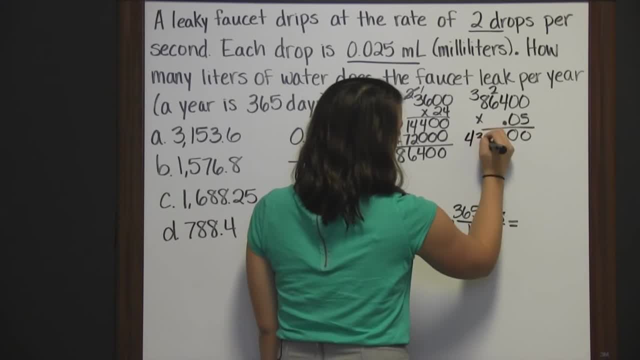 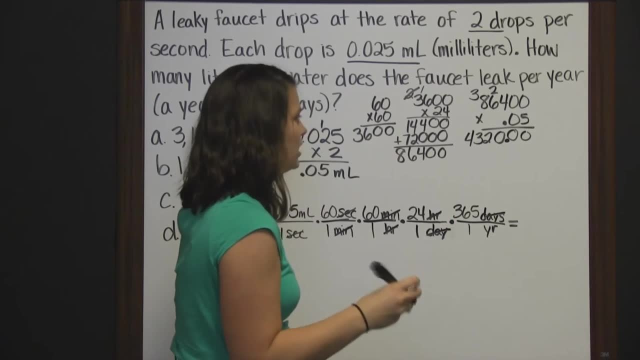 5 times 8 is 40, plus 3 is 43. And we have two numbers behind the decimal, so our answer should also have two numbers behind the decimal. And then we have one last number to multiply by, and that's 365. 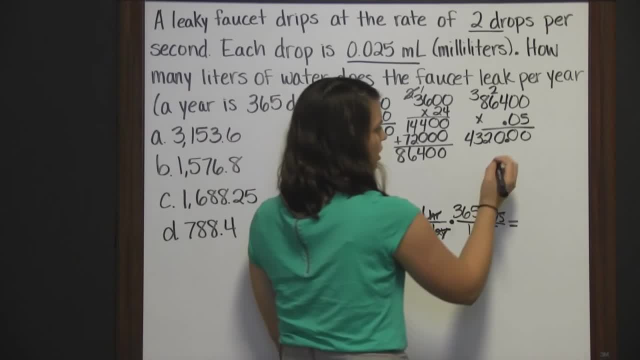 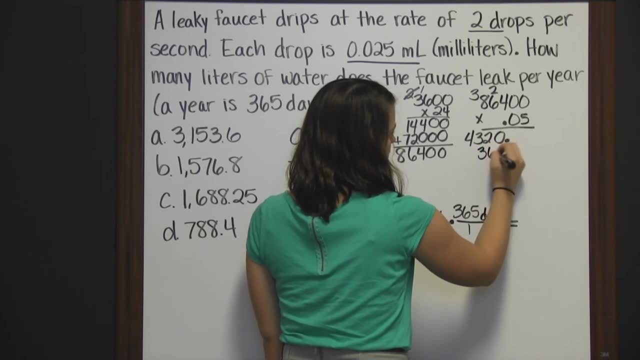 So let's see- I'm just going to try and squeeze it in right here- I can get rid of these 0s back here. They don't affect my number, So I'm just going to multiply times 365.. 5 times 0 is 0.. 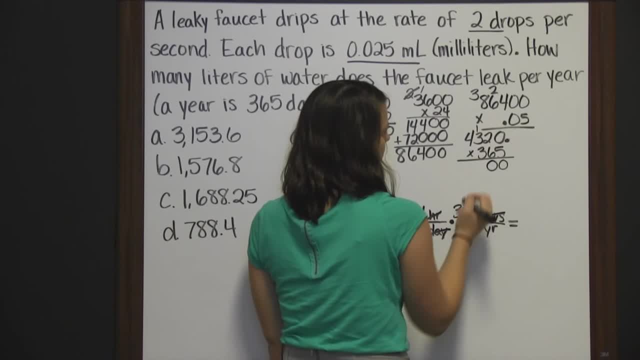 5 times 2 is 10.. Carry the 1. 5 times 3 is 15, plus 1 is 16.. Carry the 1. 5 times 4 is 20, plus 1 is 21.. 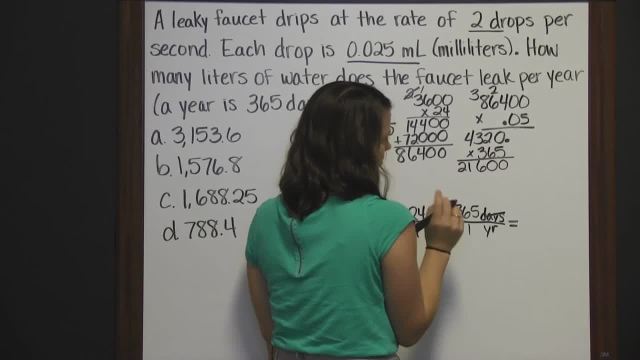 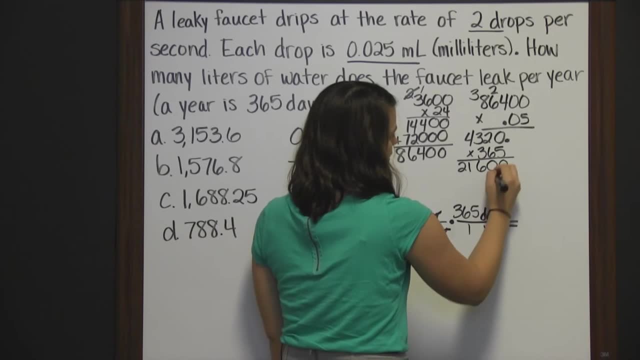 Okay, so get rid of these so that we can move on to our next number, which is 6.. So first I need to put a 0 placeholder for the 5.. 6 times 0 is 0.. 6 times 2 is 12.. 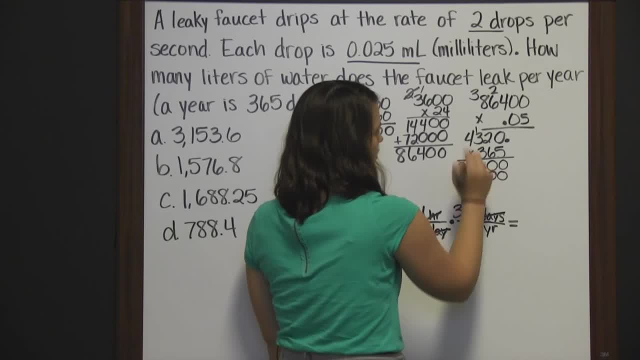 Carry the 1. 6 times 3 is 18, plus 1 is 19.. Carry the 1. 6 times 4 is 24, plus 1 is 25.. Get rid of those, And then we need now 2 0s. 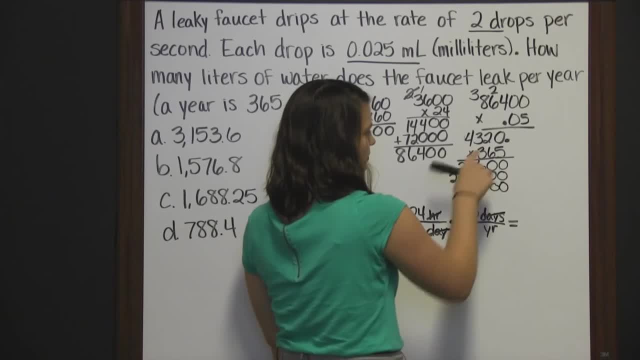 Placeholders for the 6 and the 5.. And now we're multiplying times, the 3.. So 3 times 0 is 0.. 3 times 2 is 6.. 3 times 3 is 9.. 3 times 4 is 12.. 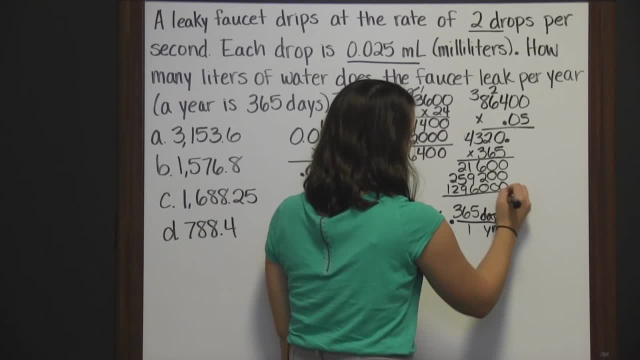 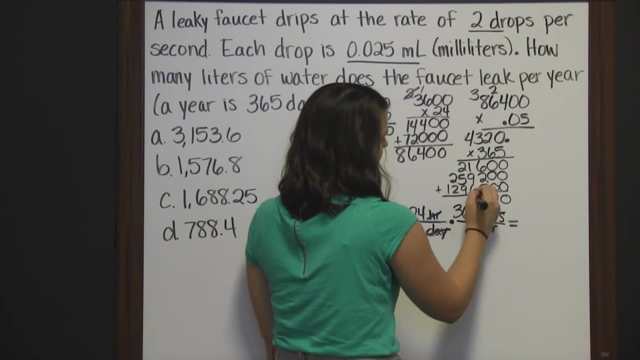 And we need to add all this up. So we get 0 here and 0 here. 6 plus 2 is 8.. 1 plus 9 is 10, plus 6 is 16.. Carry the 1.. 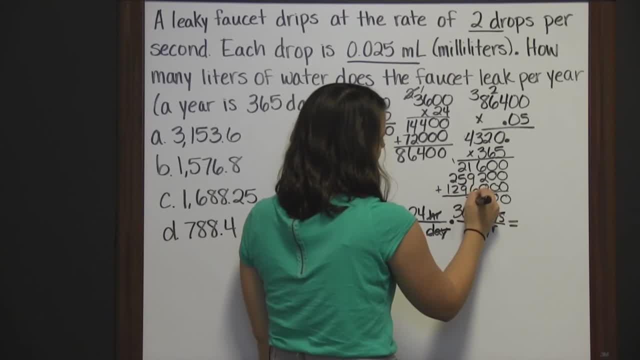 9 plus 1 is 10. 15,, 17. Carry the 1., 2,, 4,, 5.. So 1. We have 1, 2, 3, comma. 1, 2, 3, comma. 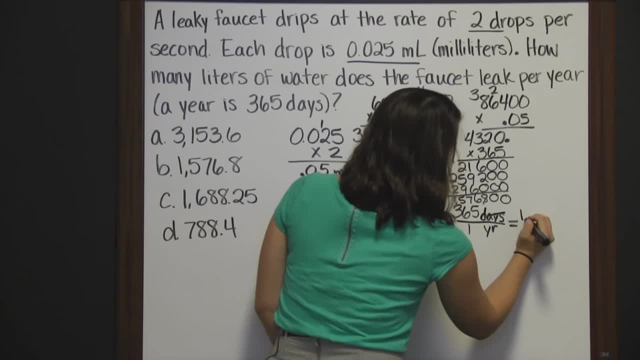 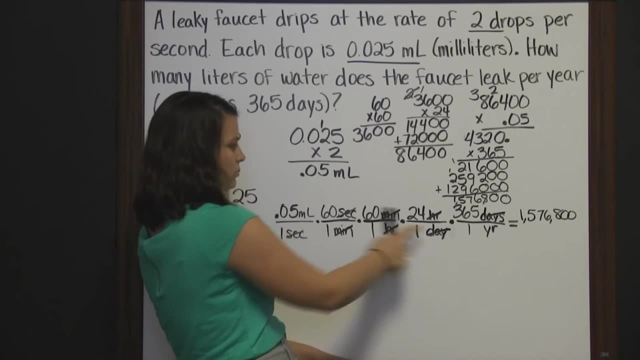 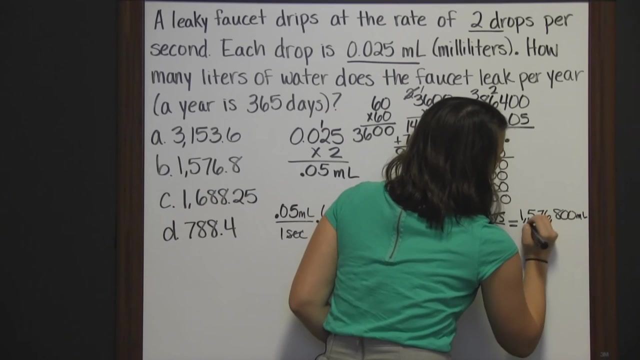 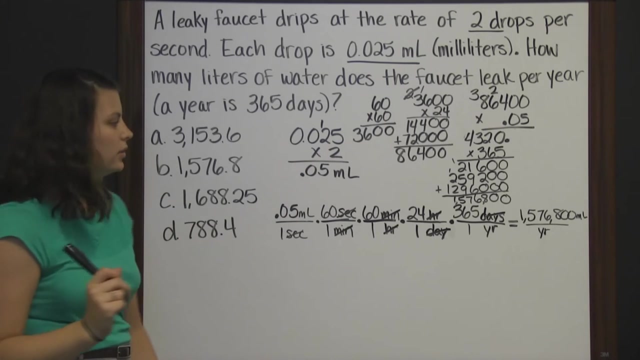 So that is 1,576,800 milliliters per year. Notice, all of our other units are canceled out except for milliliters per year. So that's milliliters Per year. But if you recall, they wanted to know how many liters of water were leaked out per year. 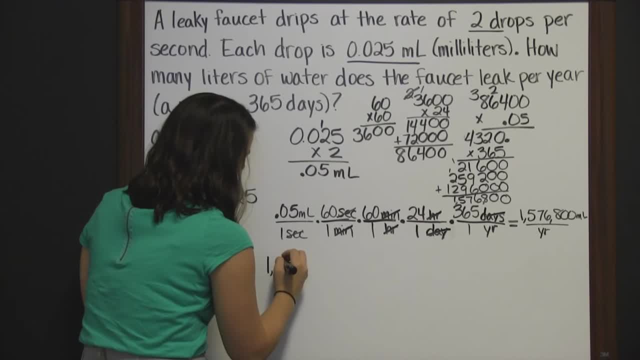 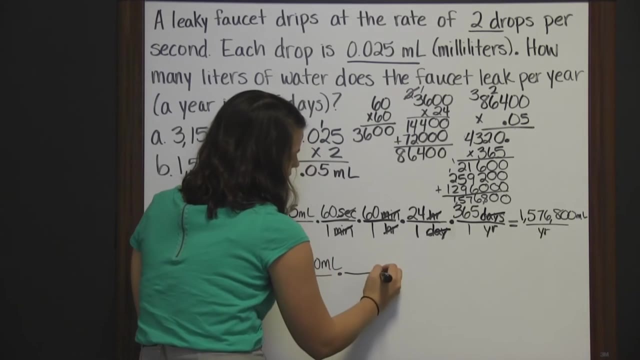 So we need to convert this 1,000, or sorry, 1,576,800 milliliters per year into liters So we can again use a conversion factor. So milliliters goes in our denominator so that it cross cancels out when we multiply. 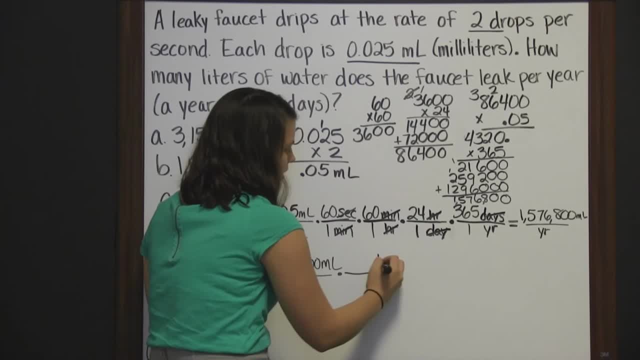 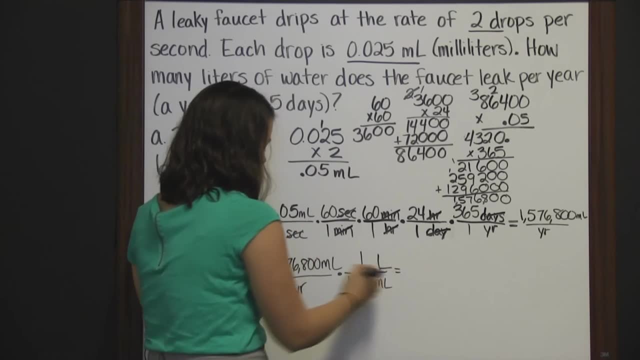 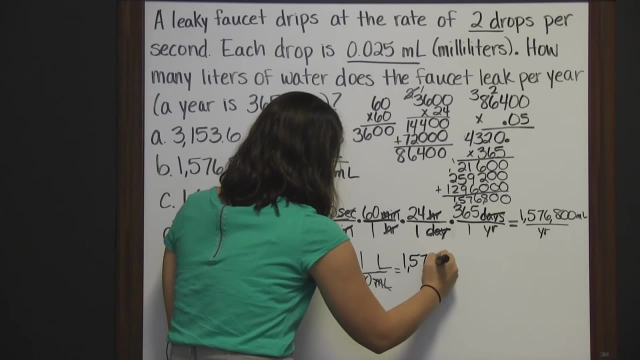 And I know that 1 liter is 1,000 milliliters. So when we multiply across we get our milliliters cross cancel And we get 1,576,800 divided by 1,000.. So we can cancel these two zeros. 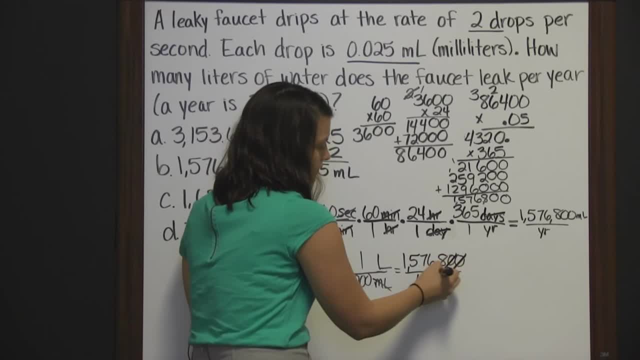 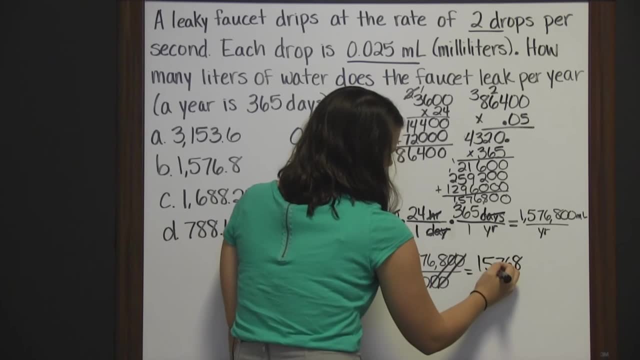 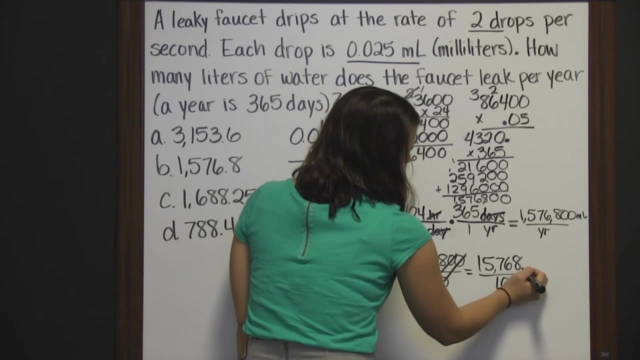 And dividing by 10 means that our decimal moves in one place. So what we have after we cancel our zeros is 15,768 divided by 10.. And when we divide by 10, that just means to take your decimal and move it one place to the left. 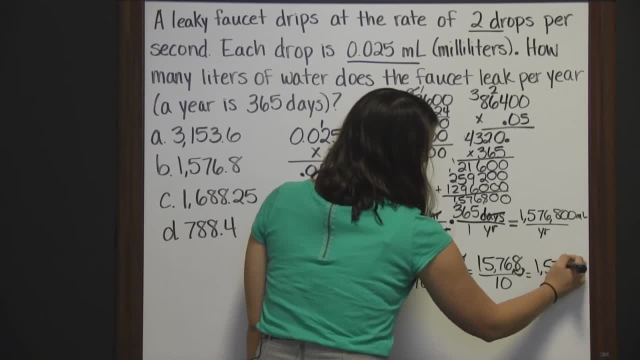 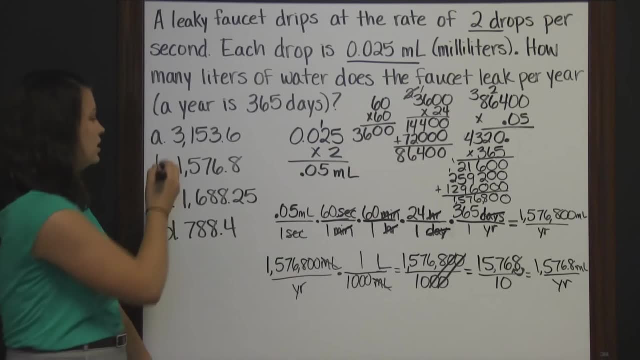 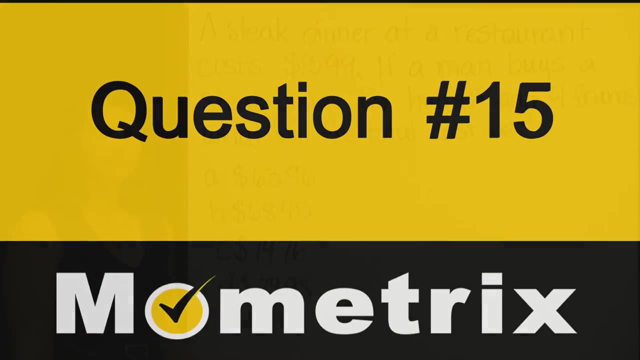 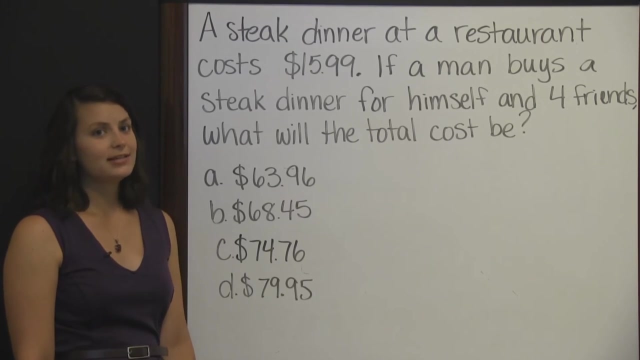 So that's 1,576,800 milliliters per year, Which is answer choice B. So a lot of converting on this one. A steak dinner at a restaurant costs $15.99.. If a man buys a steak dinner for himself and four friends, what will the total cost be? 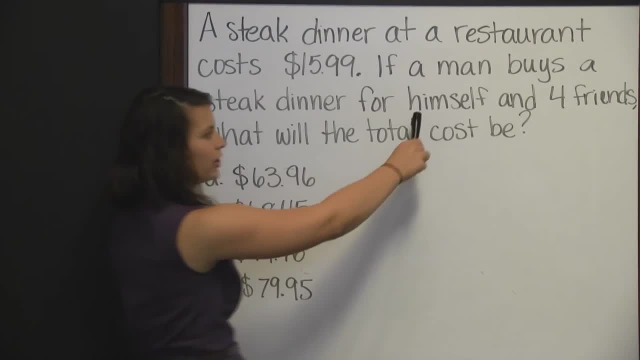 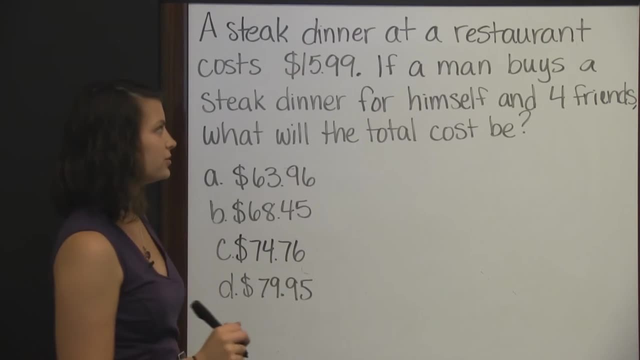 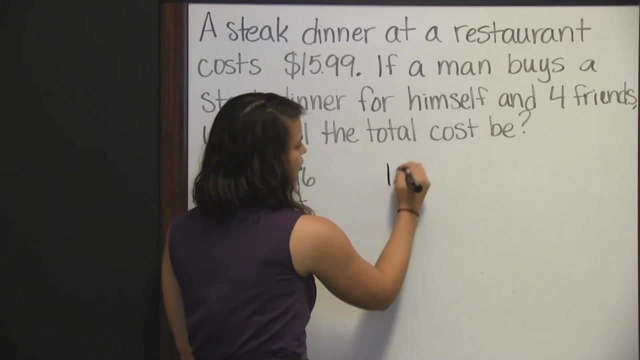 So this man is buying a steak dinner for himself and four friends, which means he's buying a total of five steak dinners. So he's going to pay for this steak dinner. five times Times means multiplication, So to find our total cost we're going to take how much one steak dinner costs. 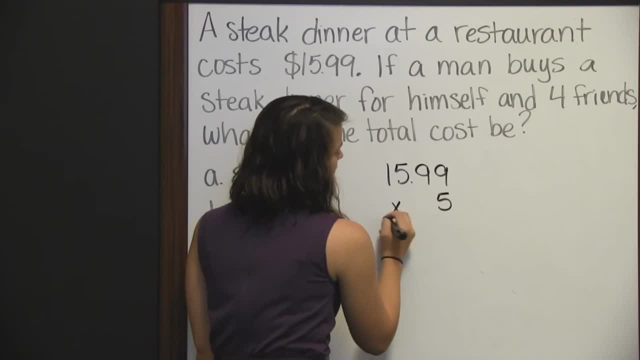 and multiply it times the number of steak dinners being purchased, which is five. Five times nine is 45, so write the five and carry the four. Five times nine again is 45, plus four is 49, and carry the four. 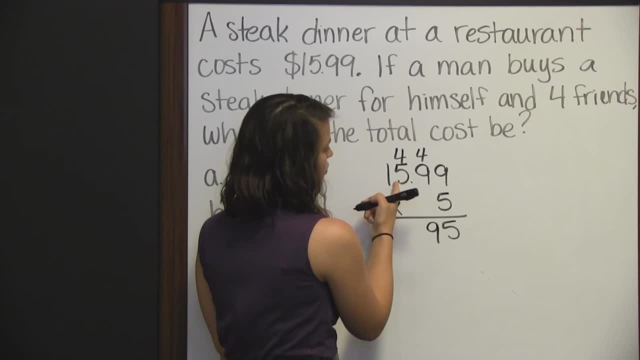 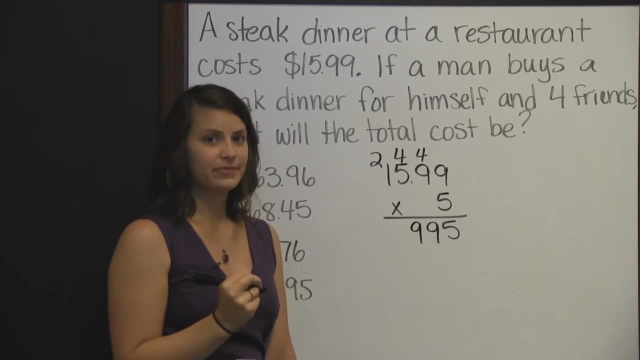 Five times five is 25, plus four is 29,. write the nine and carry the two. Five times one is five plus two is seven. And now, looking at that answer, that looks way too big, And the reason for that is we haven't put our decimal place in yet. 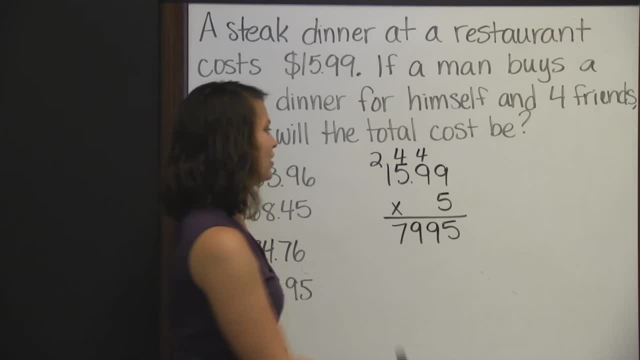 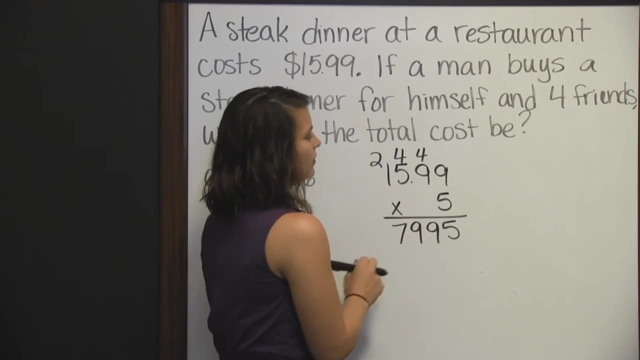 When multiplying numbers, the number of numbers behind the decimal place depends on the number of numbers behind the decimal in the two numbers you multiplied together. So here we have two numbers behind our decimal, and so we have two numbers behind our decimal in our answer. 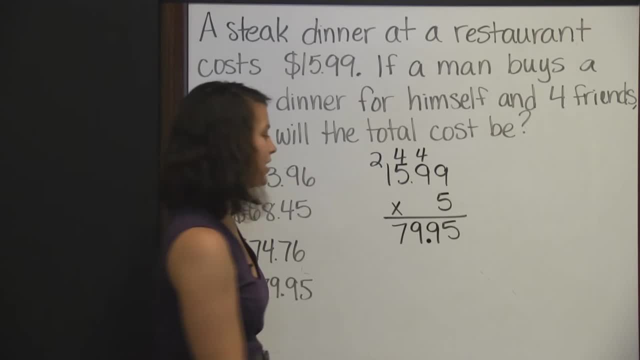 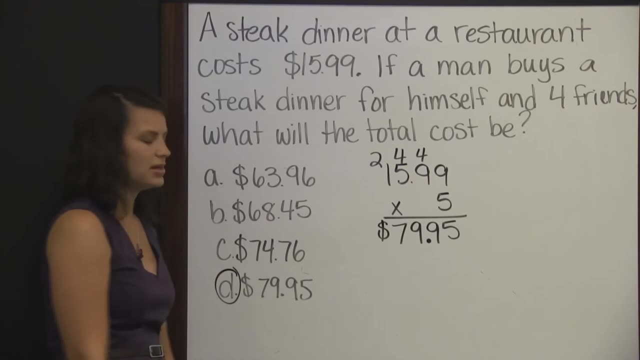 So we have two numbers behind our decimal, And so we have two numbers behind our decimal in our answer as well. So the answer is $79.95, which is answer choice D. It's going to cost him $79.95 to pay for his steak dinner. 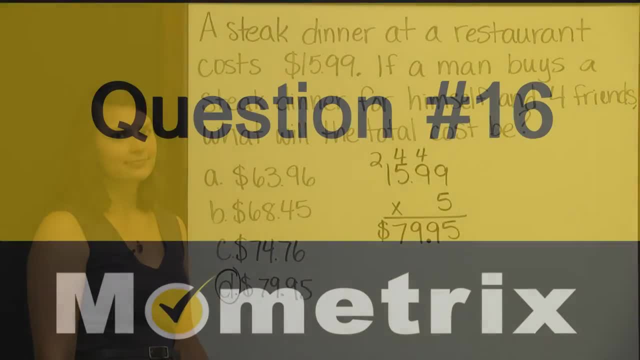 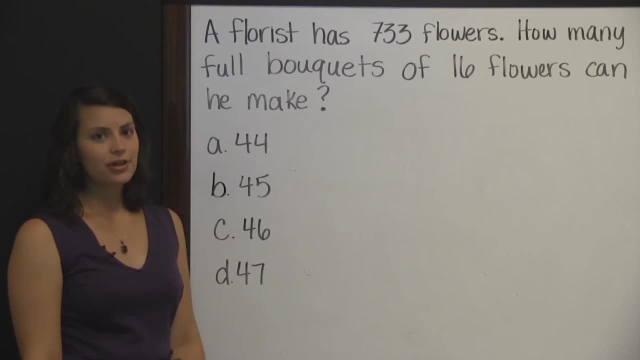 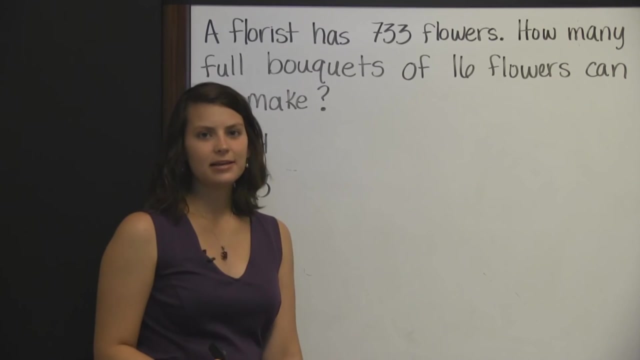 and the steak dinners of his four friends. A florist has 733 flowers. How many full bouquets of 16 flowers can he make? We want to take this number, 733, and divide it by 16, because we're dividing the flowers up into bouquets. 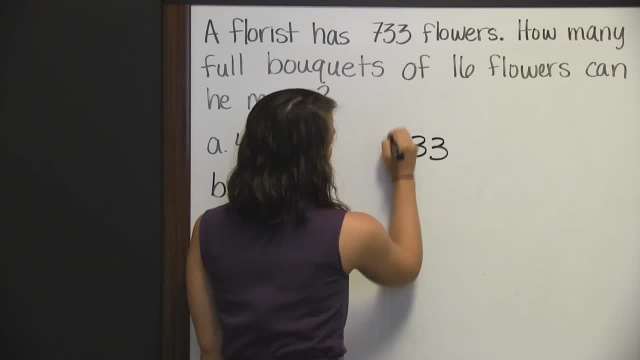 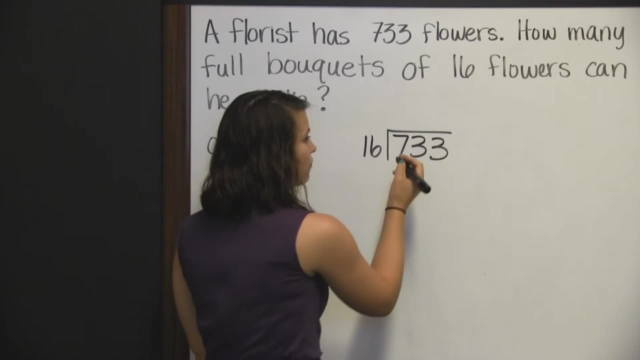 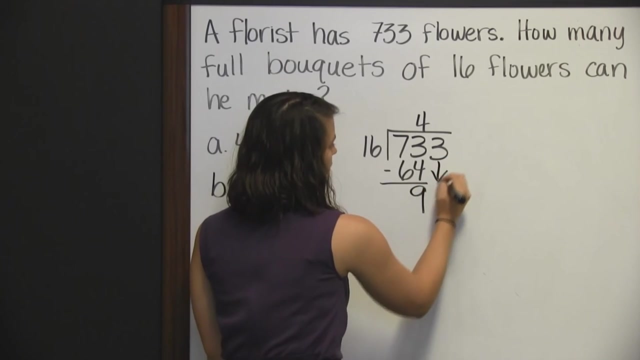 So we take 733 and divide it by 16. 16 goes into 73 four times 16 times 4 is 64. And then we subtract And we get 9.. Bring down the 3. And 16 goes into 93 five times. 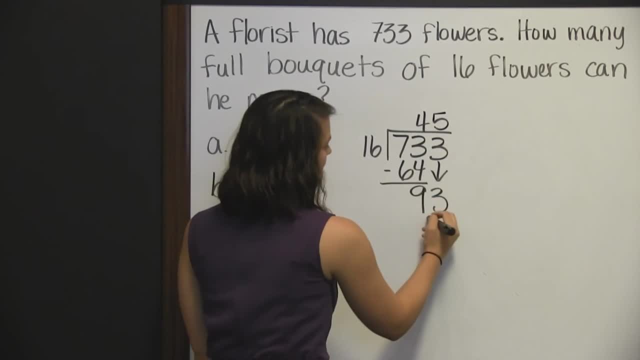 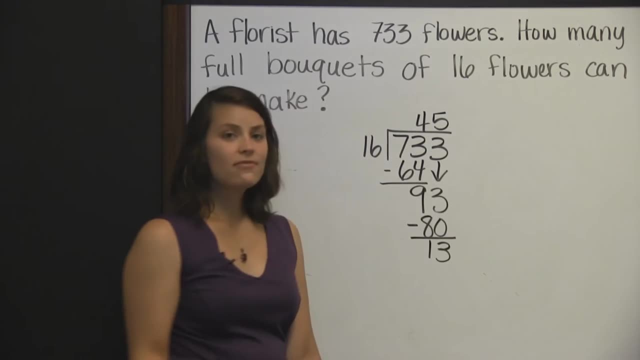 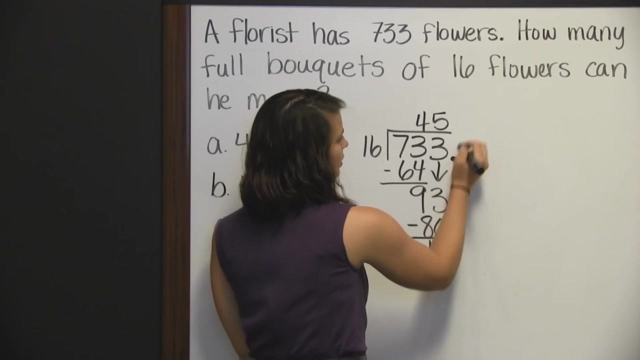 16 times 5 is 80.. We subtract again, We get 13.. So we have a remainder And we could stop here. Or we could add a decimal And add a decimal here in our answer And add a 0.. 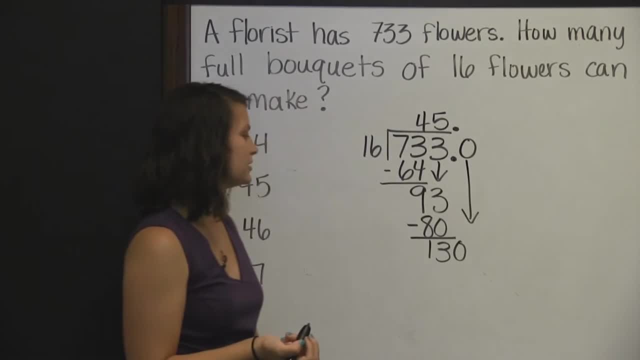 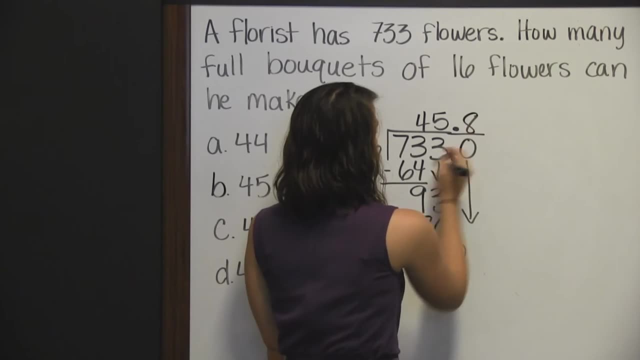 And then we could bring that 0 down And we could find out what our decimal is. So 16 now goes into 130. eight times 16 times 8 is 128.. And again we subtract And we get a remainder of 2.. 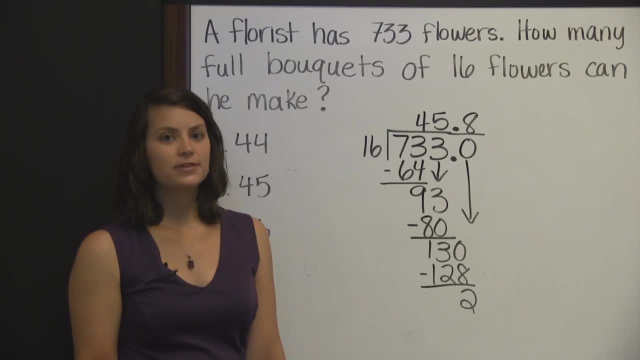 And we could continue on until we have no remainder left And we could find out what our whole answer is, the whole decimal number. But really it's not necessary. If we look at our answer choices, we've already found our answer. 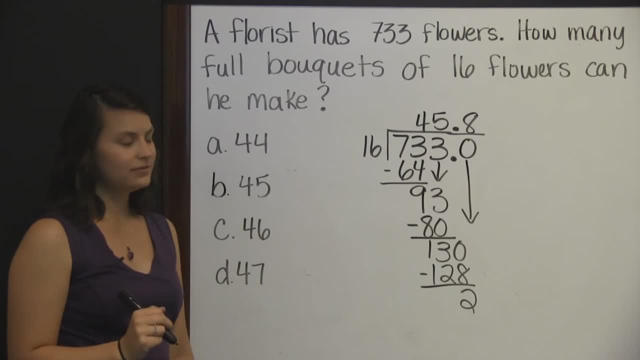 We were asked how many full bouquets could be made out of 733 flowers, And we found it. You can make 45 full bouquets with some flowers left over. Actually, 13 flowers is what would be left over, Or 8 tenths. 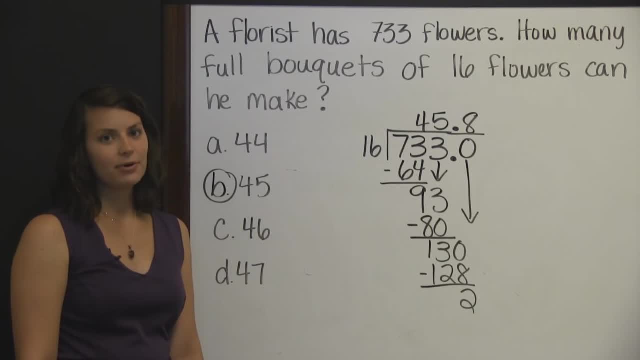 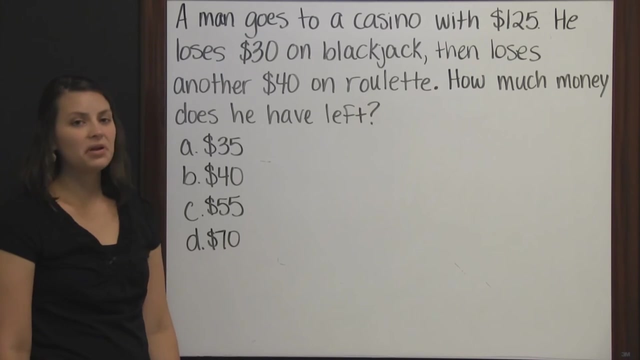 So our answer is B. 45 full bouquets of flowers can be made out of the 733 flowers, using 16 in each bouquet. A man goes to a casino with $125.. He loses $30 on blackjack, Then loses another $40 on roulette. 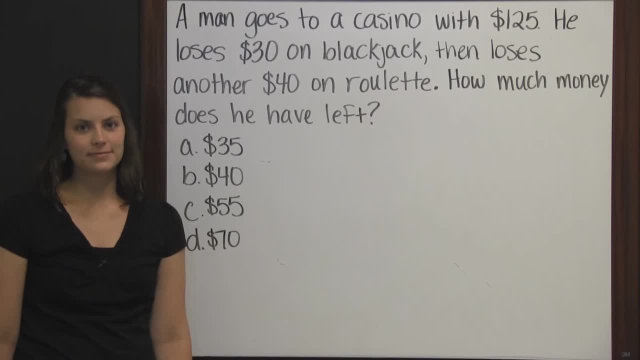 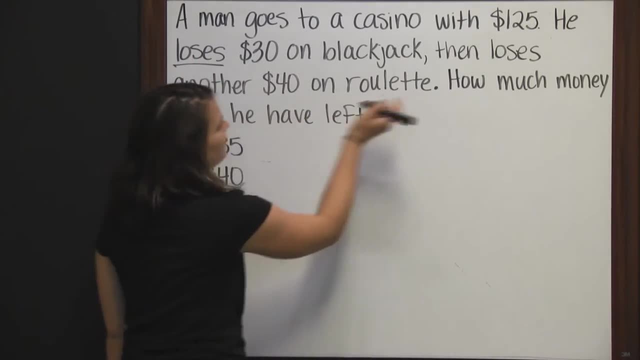 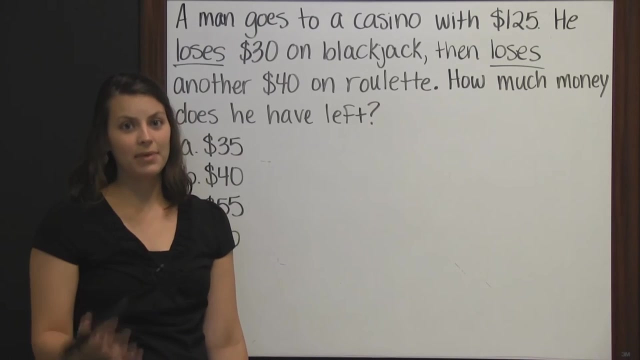 How much money does he have left? So the key word here is loses. He's losing money. You see it in two different places. He's losing money, which means that's money that is taken away from him or subtracted from his total. 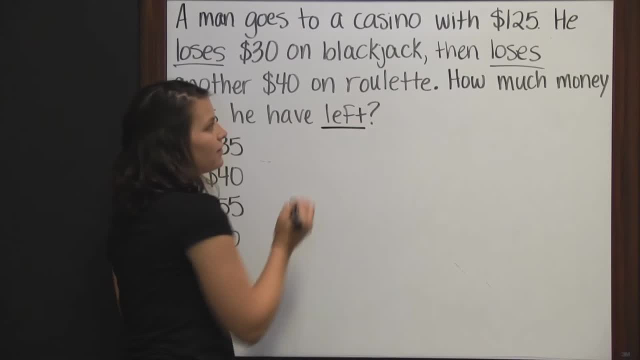 So to determine what he has left, we're going to subtract the money he lost from what he came with. So he started with $125.. Then he lost $30.. So subtract $30 from how much he has. 5 minus 0 is 5.. 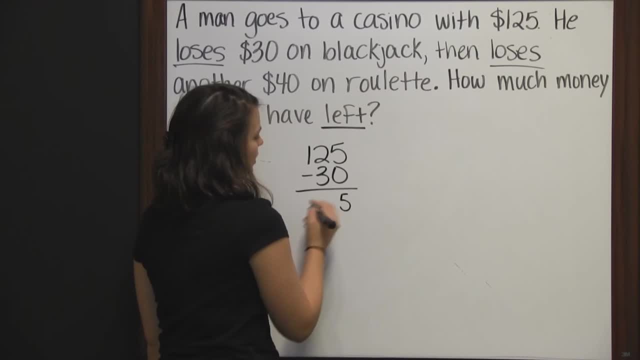 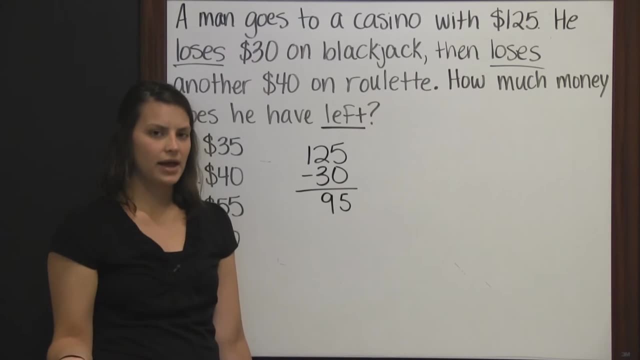 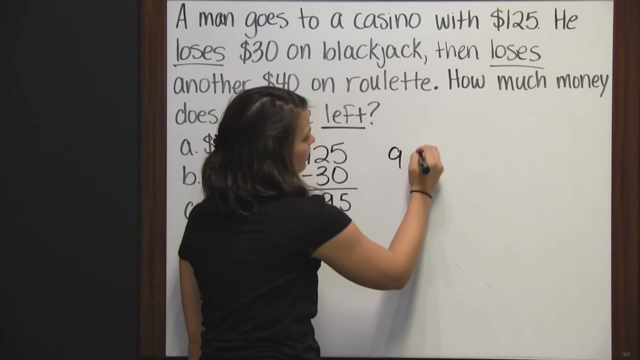 And 12 minus 3 is 9.. So after he lost that $30, he still had $95 left, But then he lost $40.. So from that $95 he had he lost another 40.. 5 minus 0 is 5.. 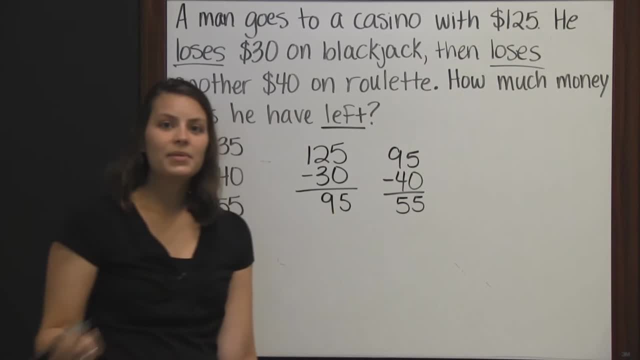 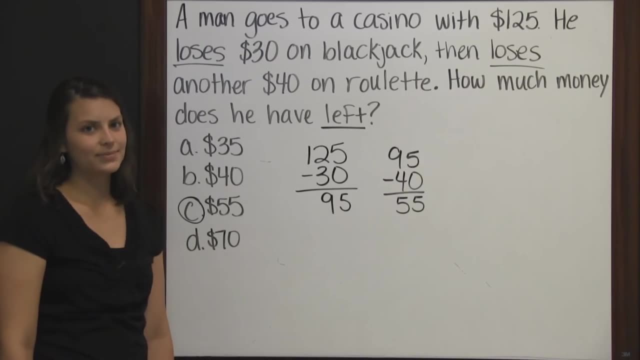 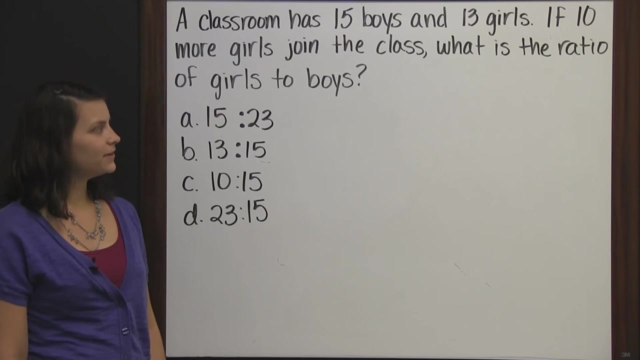 And 9 minus 4 is 5.. So that means after all the money he lost, he was left with $55.. Answer choice C: A classroom has 15 boys and 13 girls. If 10 more girls join the class, 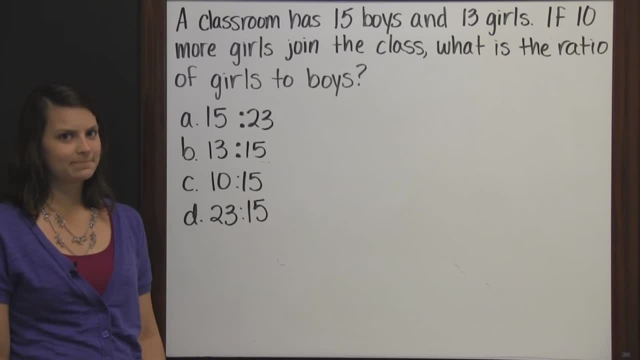 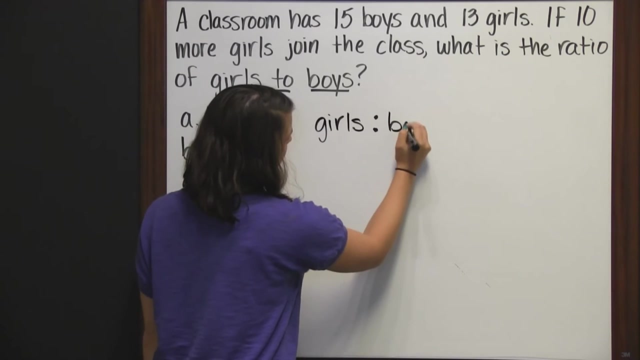 what is the ratio of girls to boys? Well, this last sentence tells us how to set this up. What is the ratio of girls to boys? So we're going to have girls to boys, And there are lots of ways to write ratios. 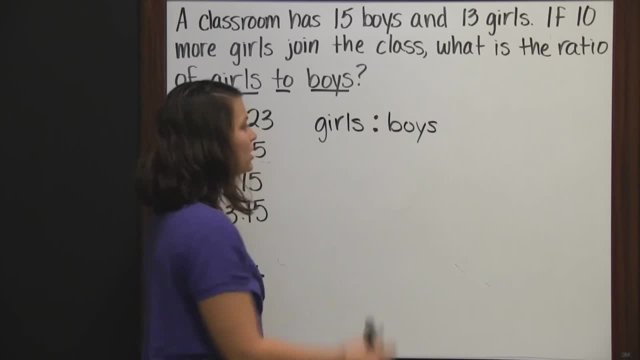 You could actually write out the word 2 like they did in the question, Or you could write it as a fraction, with girls on the top and then boys as the denominator. But if we look at our answers we can see they used a colon for 2.. 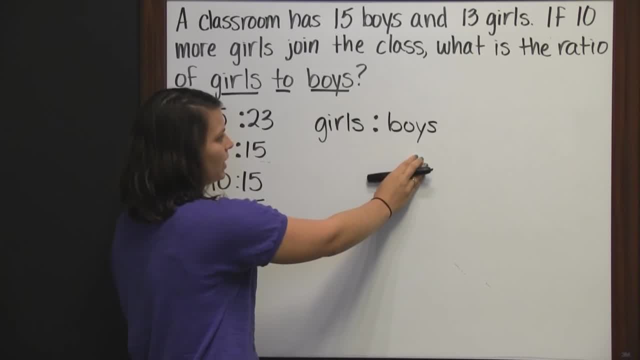 So I wrote mine the same way, Girls to boys, And before we can write our ratio we need to know how many girls there are. So it says the classroom has 15 boys and 13 girls, And then 10 more girls join the class. 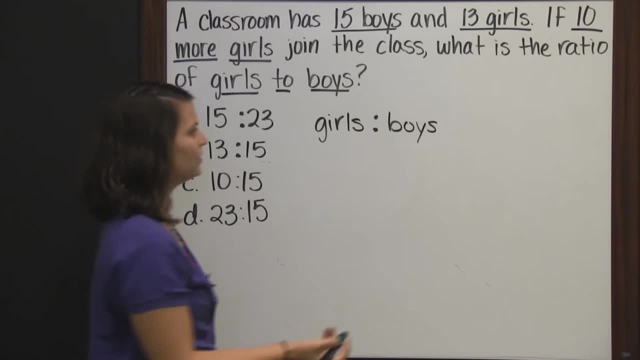 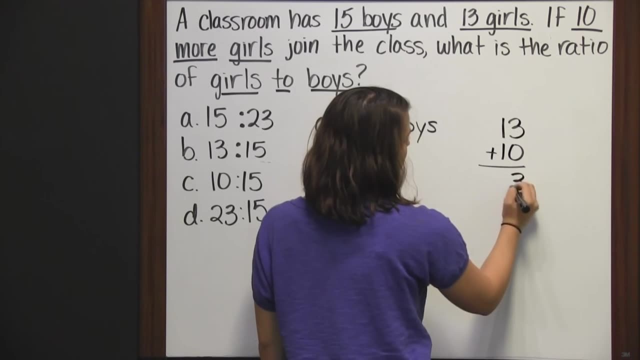 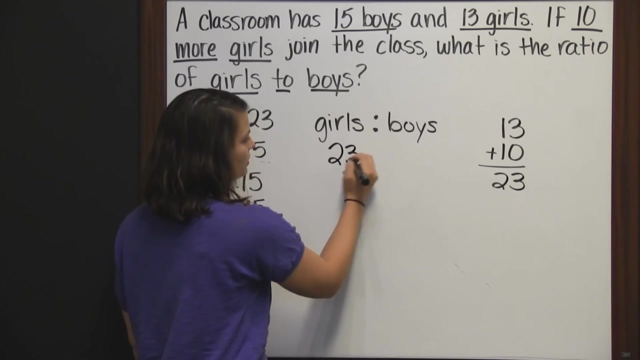 10 more means that we have to add 10.. So we had 13 girls, and then we add 10 more to that. 3 plus 0 is 3.. 1 plus 1 is 2. Which means now there's a total of 23 girls. 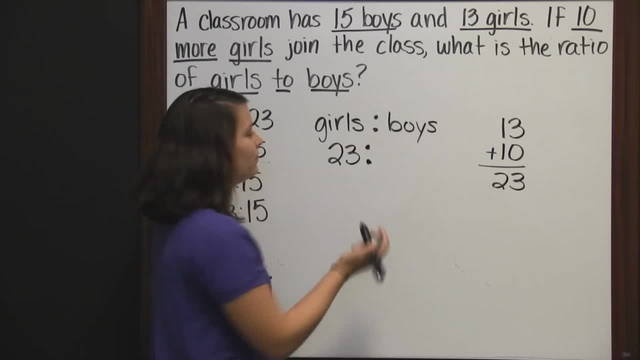 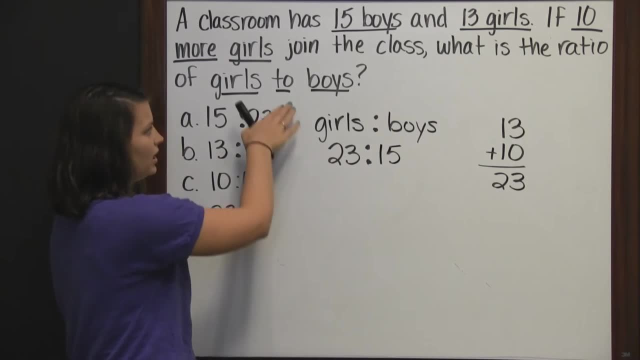 to 2. And then boys didn't change. We had 15 boys, so we still have 15 boys, And it is very important that the ratio is written in the way it's asked to be written. So if you look at A, 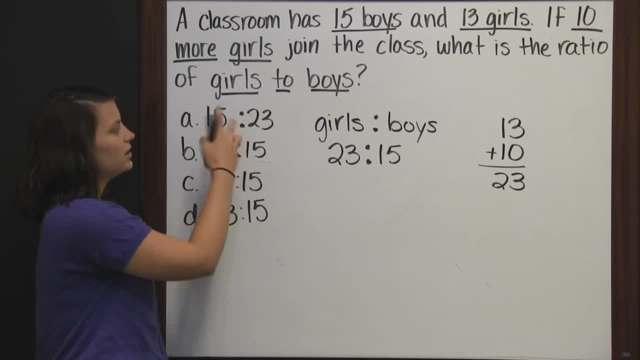 you can see, it's the same that we have 23 to 15, except it's reversed, And so that would not be the ratio of girls to boys. This is the ratio of boys to girls, which is not the same. 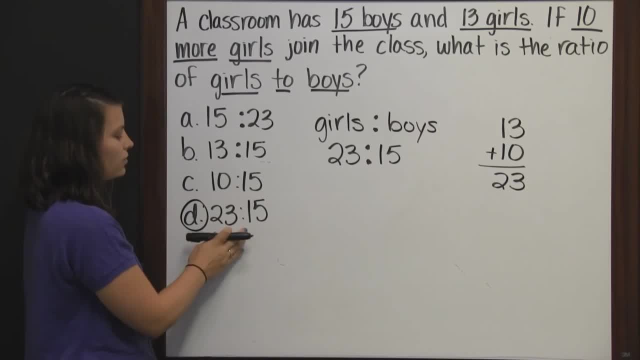 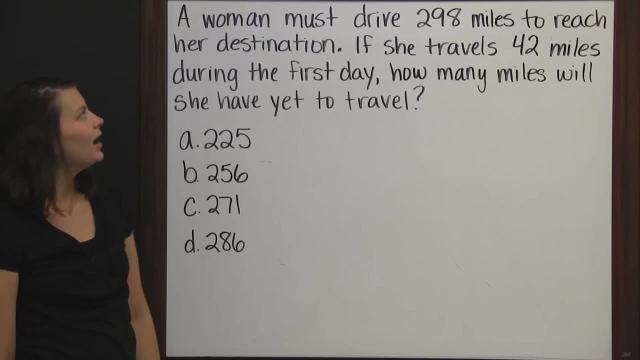 So our answer is answer D: 23 girls to 15 boys. A woman must drive 298 miles to reach her destination. If she travels 42 miles during the first day, how many miles will she have yet to travel? 298 miles. 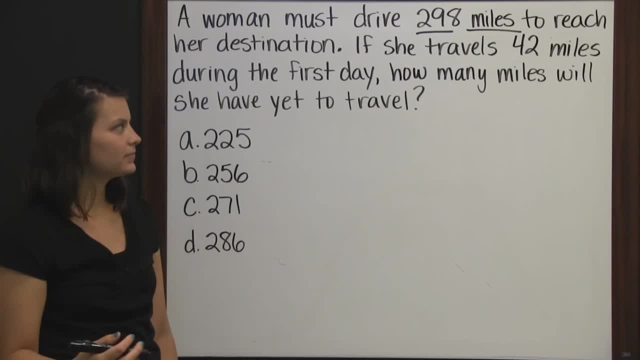 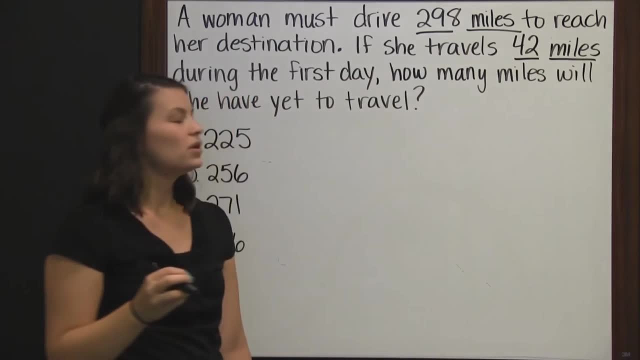 is the total that must be driven. It says on the first day she drove 42 miles. So she's already taken care of 42 of those 298 miles that she has to travel. So if we want to figure out how many she has left, 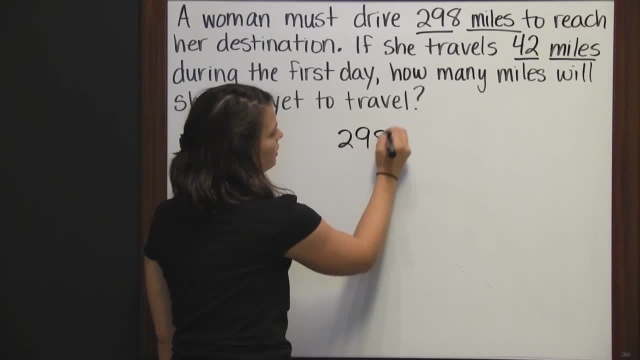 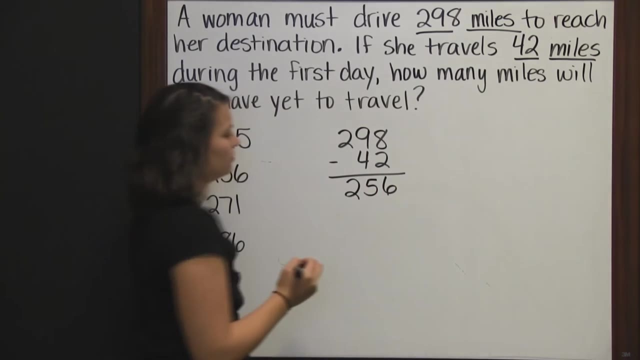 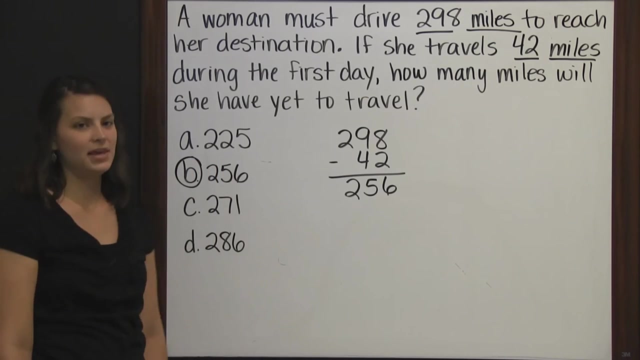 we need to subtract 298 minus 42.. 8 minus 2 is 6.. 9 minus 4 is 5.. And we bring down the 2.. That means she has 256 miles left to travel. Answer choice B: 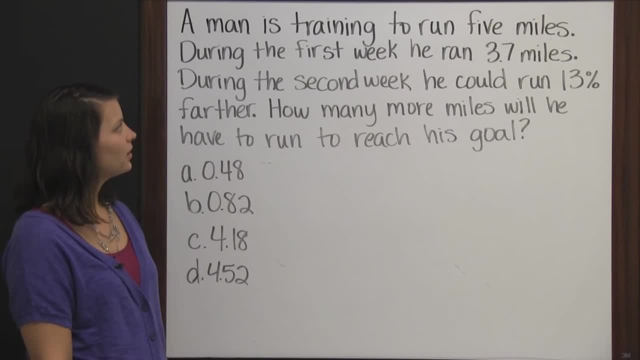 A man is training to run 5 miles. During the first week he ran 3 and 7 tenths miles. During the second week he could run 13% farther. How many more miles will he have to run to reach his goal? 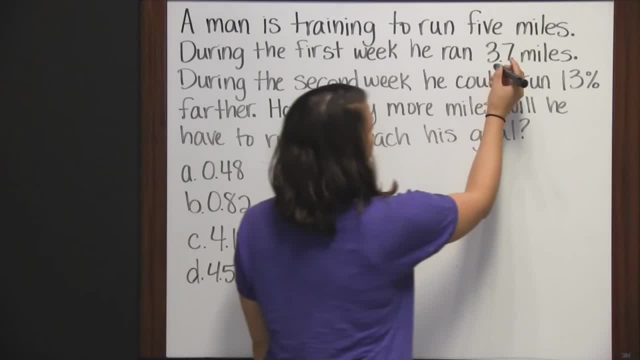 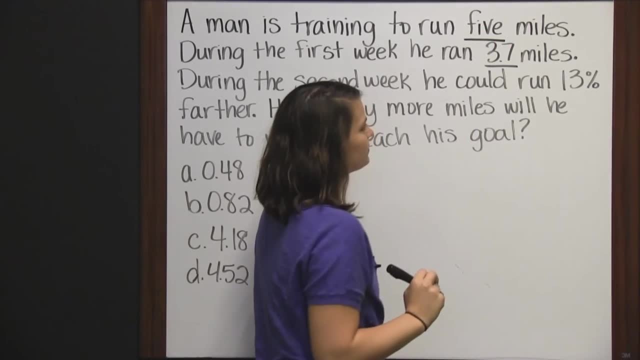 So in this first week he was able to run 3 and 7 tenths miles, And let's keep in mind what the goal is: 5 miles. In the second week he could run 13% further than the week before. 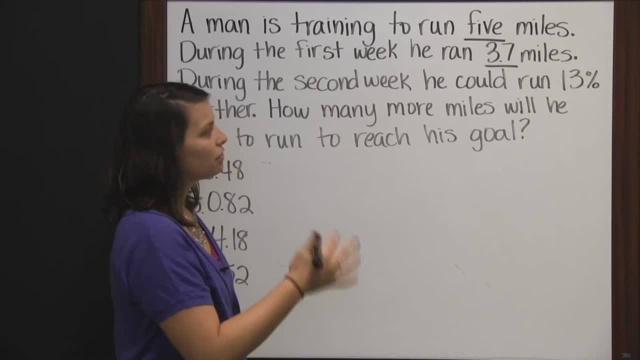 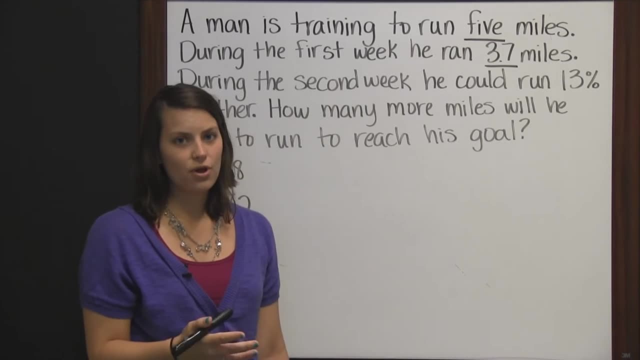 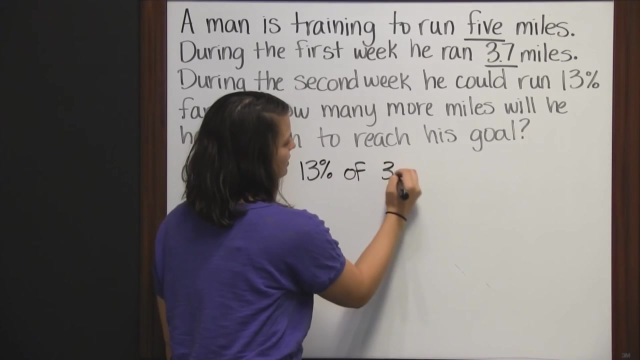 So let's figure out what that is. He could run the 3 and 7 tenths miles and then even 13% more than that. So first we have to figure out what 13% of 3 and 7 tenths miles is. 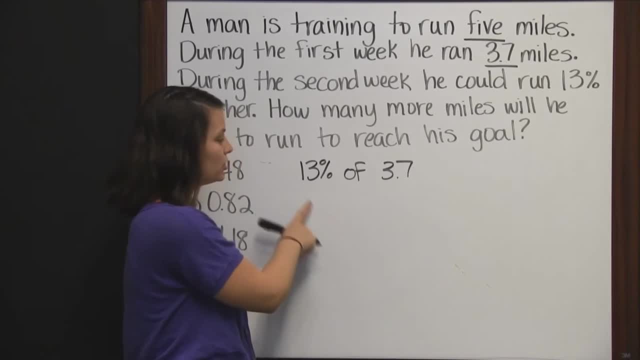 And of means to multiply. So we're going to take our percent and change it to a decimal, Move it two places to the left, And then we're going to multiply 3 and 7. tenths times 13. hundredths 3 times 7 is 21.. 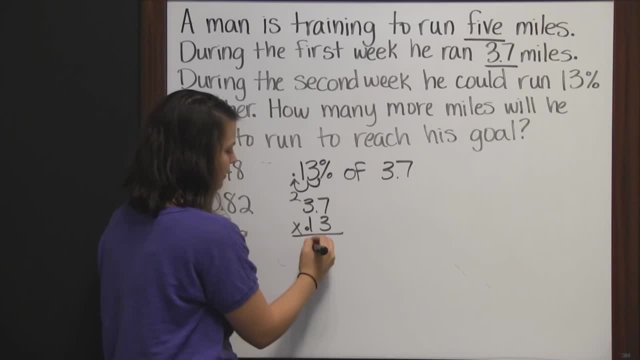 3 times 3 is 9,, 10,, 11.. 0 placeholder 1 times 7 is 7. And 1 times 3 is 3.. Add those together: 1,, 8,, 4.. 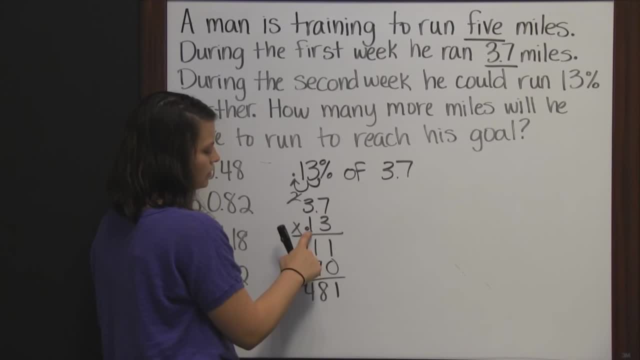 And then we have 1,, 2,, 3 numbers behind the decimal, Which means our answer will have 3 numbers behind the decimal. So when it said he could run 13% farther, then that means the 3 and 7 tenths miles. 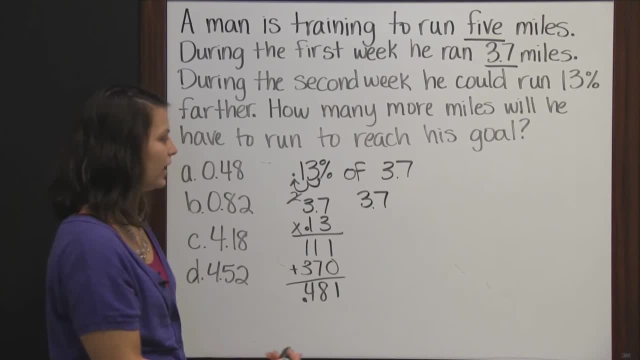 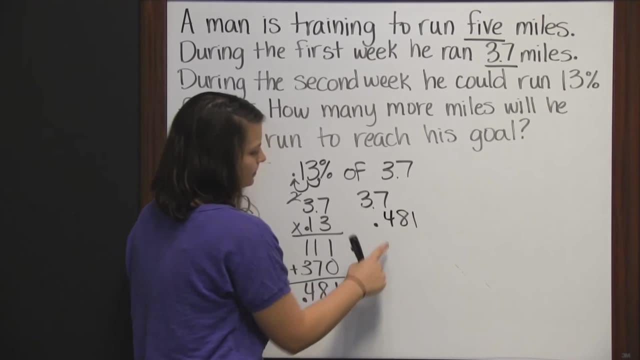 plus the 13% of 3 and 7 tenths. So we have to line up the decimal And we have 481 thousandths that we need to add to 3 and 7 tenths. We can put 0 placeholders here. 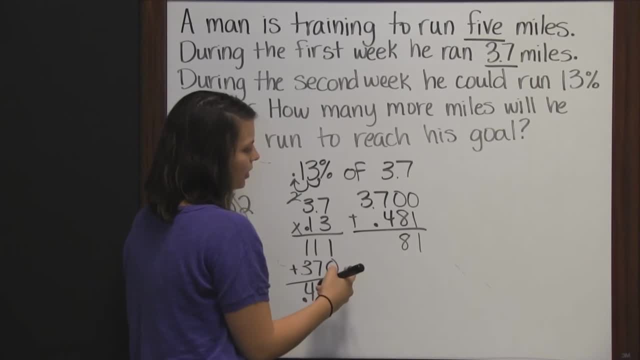 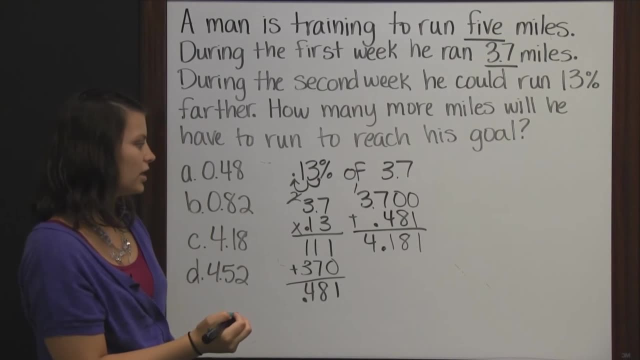 So we get 1,, 8.. 7 plus 4 is 11.. Carry the 1. So we get 4.. Bring down our decimal And we have 1,, 8,, 7.. And now we have: 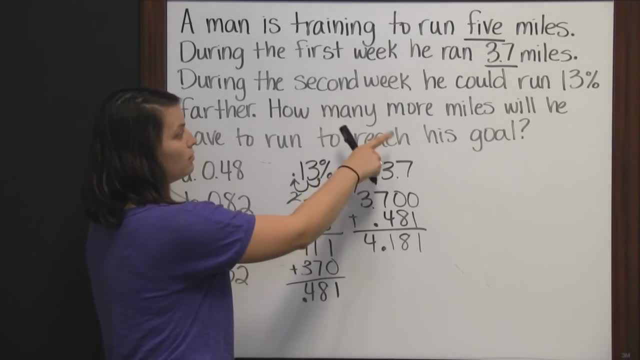 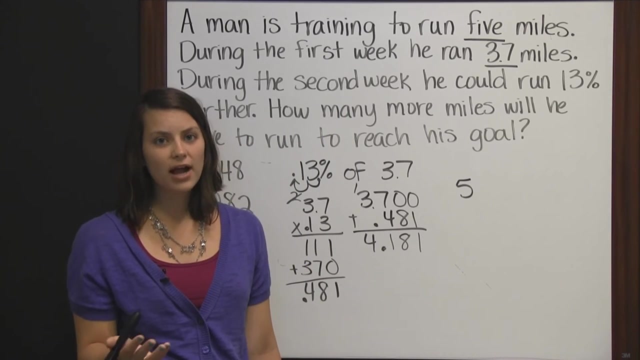 3,, 8,, 7.. And then we have 5., And now we have 6., And now we have 3.. And now we have 4.. And now, Well, if you can't find the decimal, then the decimal is behind the number, or if you. 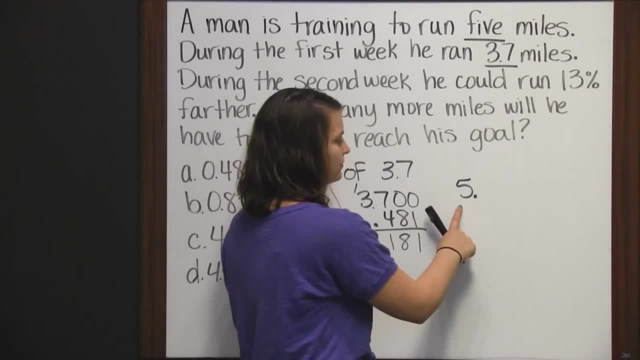 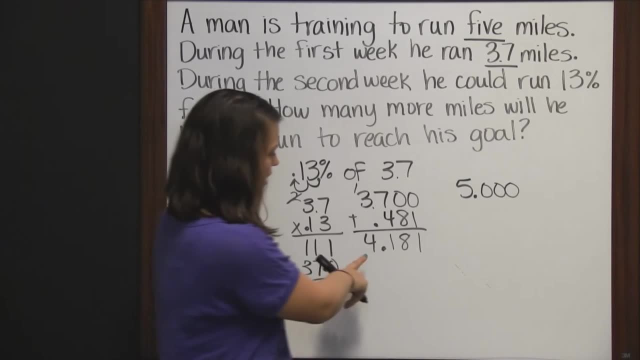 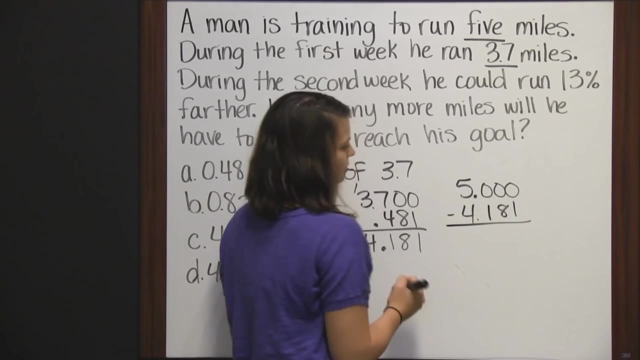 can't find it. it's behind it. So this is 5, and you can add as many 0s as you want to add, and the number doesn't change. And then we're going to subtract 4 and 181 thousandths from that. 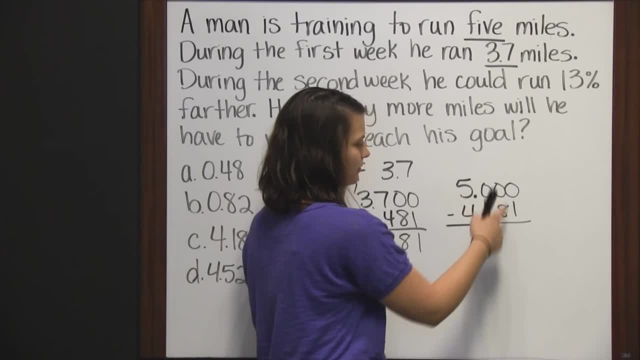 So we're going to need to borrow, because we can't take 1 from 0, or 8 from 0, or 1 from 0. So we're going to borrow from the 5, it becomes 4.. So this is 10, and then we'll borrow. 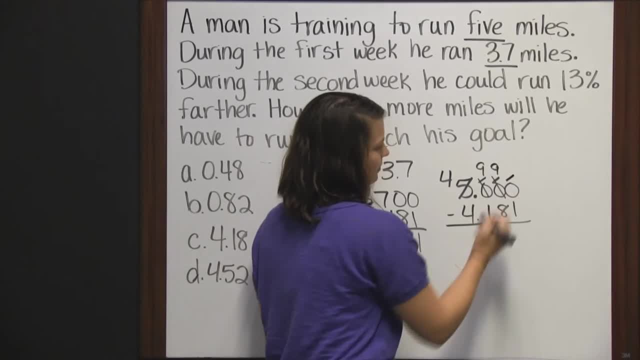 So this is 10, and then we'll borrow, And then finally we have 10 in our first position. So 10 minus 1 is 9,, 9 minus 8 is 1,, 9 minus 1 is 8.. 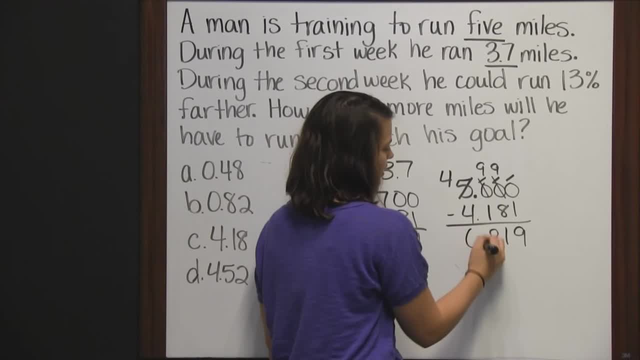 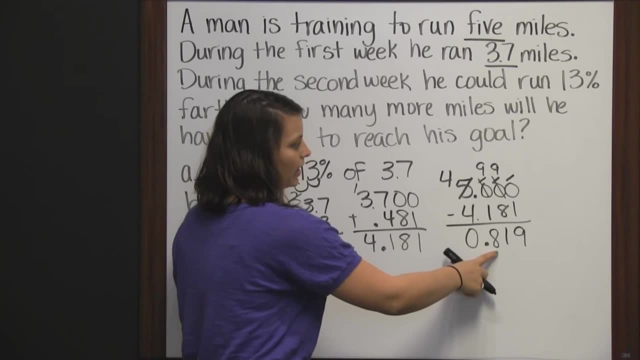 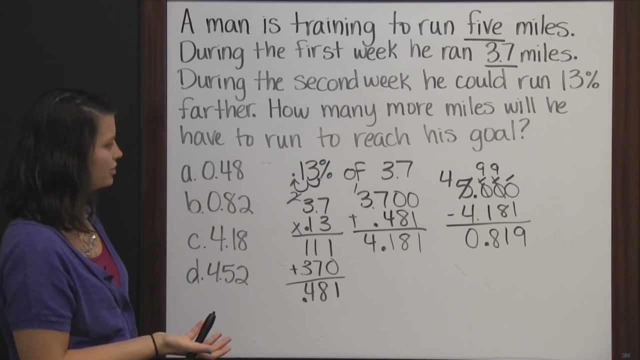 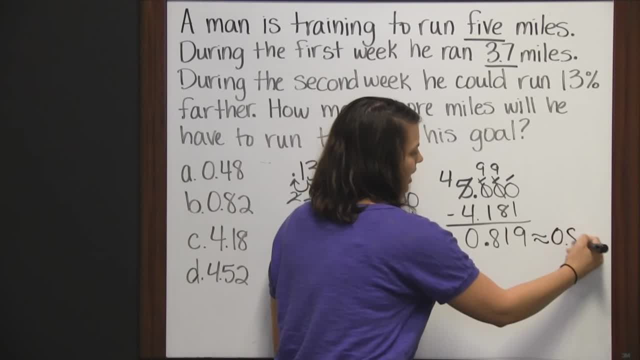 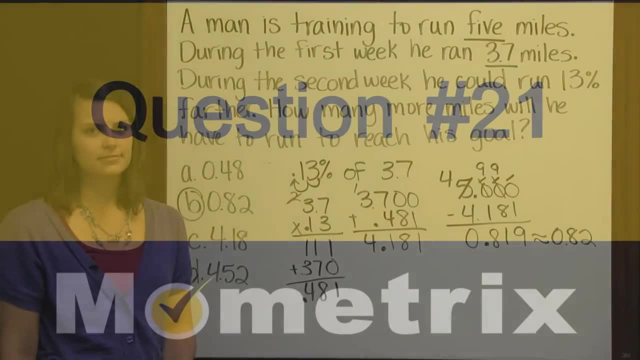 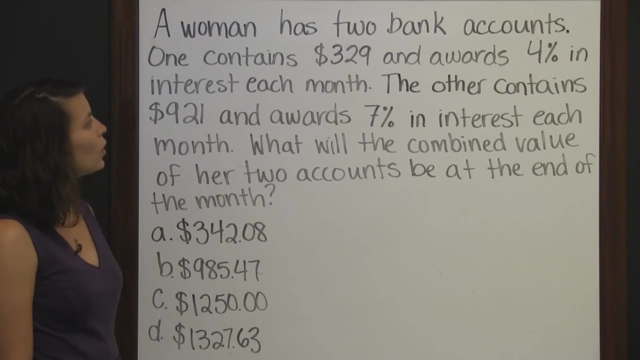 So the 9 tells the 1 to go up to a 2. So this is approximately 82 hundredths, which would be answer choice B. A woman has two bank accounts. One contains $329 and awards 4% in interest each month. 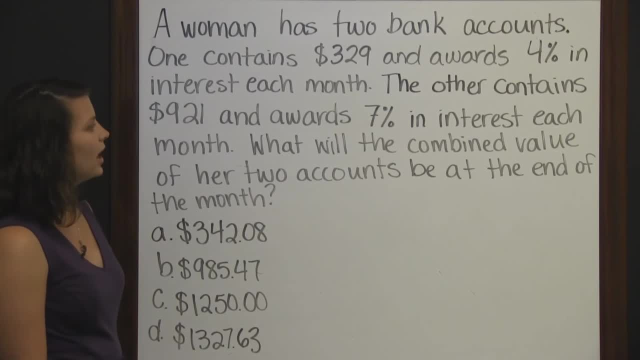 The other contains $921 and awards 7%. What will the combined value of her two accounts be at the end of the month? Combined means that we're going to add the totals of those two accounts together. So, looking at these answer choices, we can already eliminate a couple. 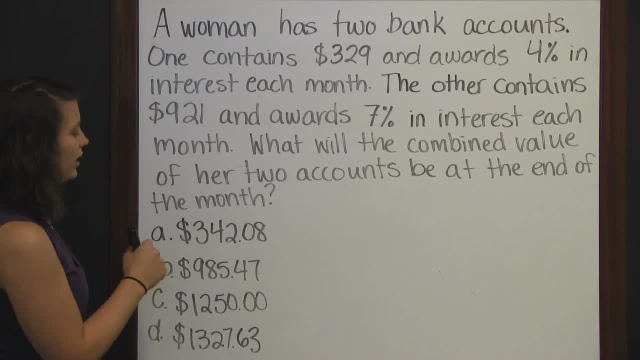 If you add together 921 and 329, you're definitely going to get more than $342.08.. So we already know we can eliminate this answer. So same with B as well: $921 plus $329 is going to be more than $985.47. 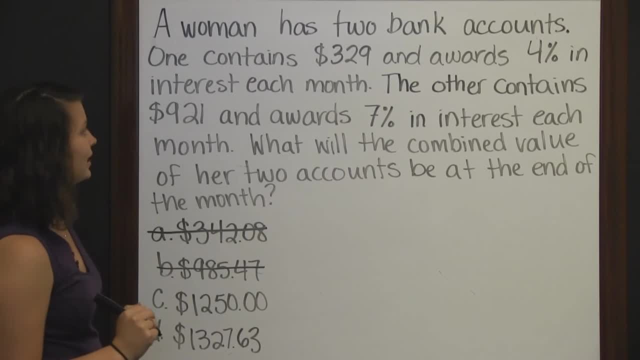 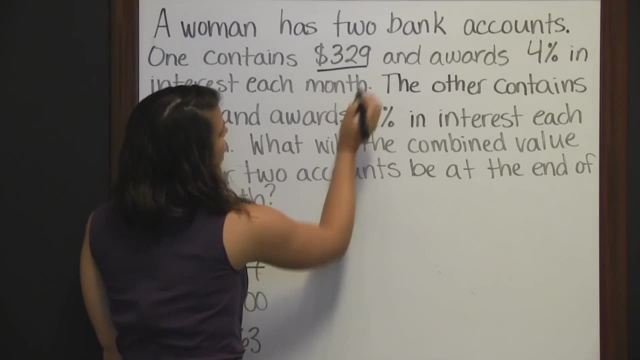 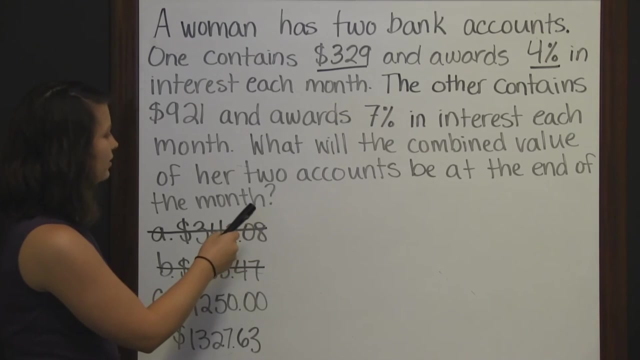 With these last two. we may actually have to do a little bit of calculating to figure those out. So it says her first account is $329 and she gets 4% in interest. So she's earning $329 in interest for each month. 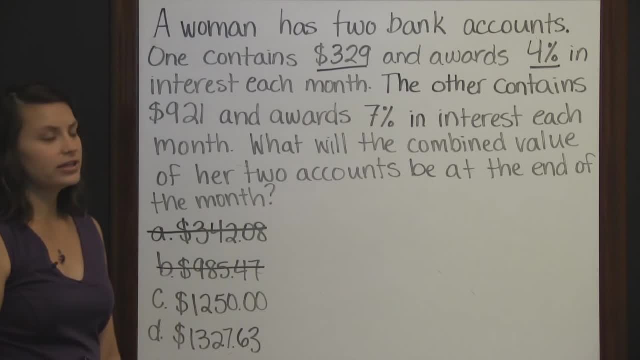 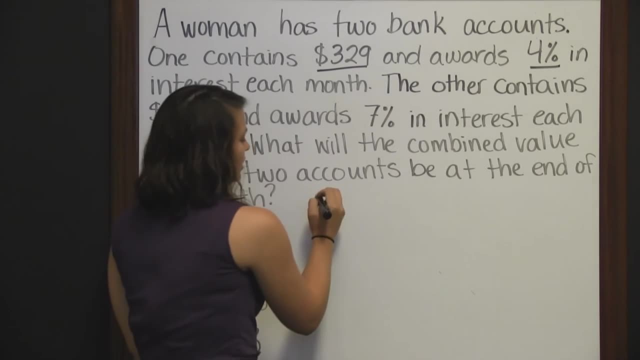 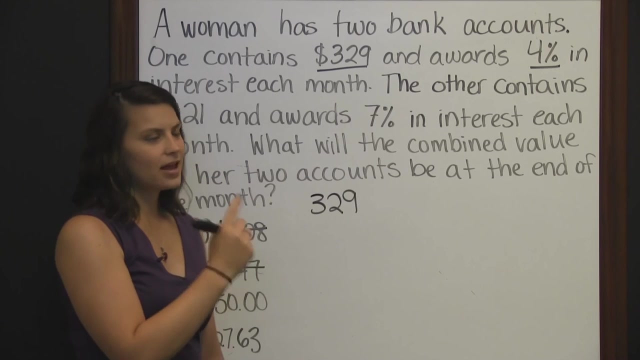 We're trying to find the combined value at the end of the month, which means that she has earned that interest for each one of her accounts. So let's start with the account with $329 in it. She has $329, and she earns 4% of that every month. 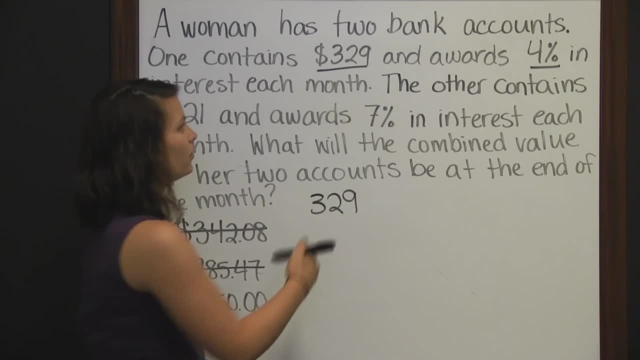 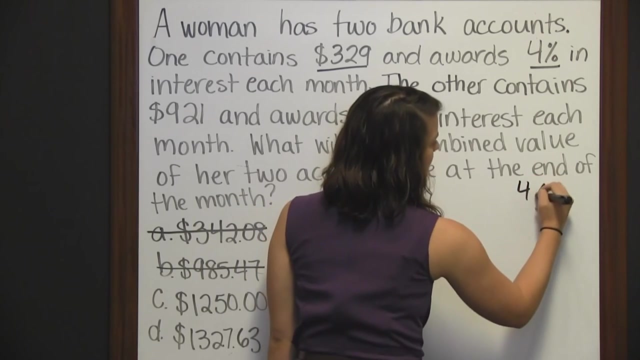 Of means to multiply. she earns on an account. we need to multiply $329 times 4%, which means we have to change our percent 4% into a decimal, So 4% as a decimal. the decimal is in the back move. 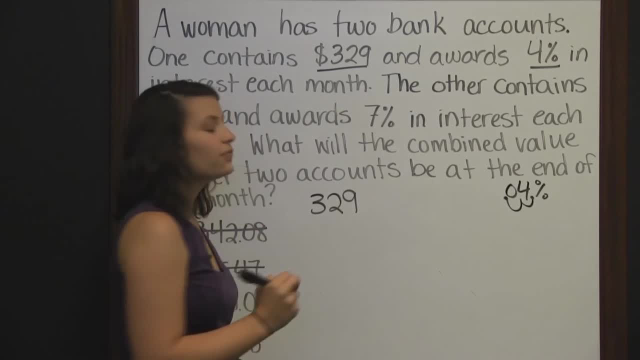 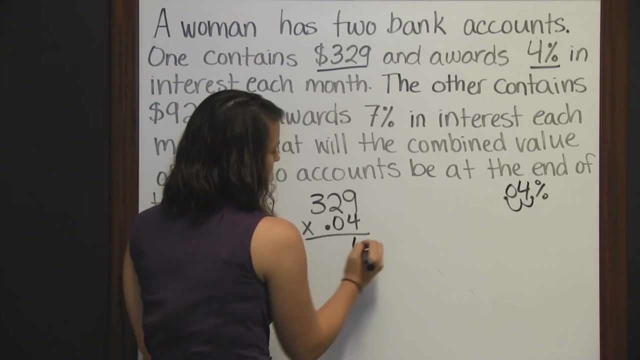 it two places to the left is 4 hundredths. So we're multiplying $329 times 4 hundredths And again this is defined how much interest was earned in this account. So 4 times 9 is 36, write the 6 and carry the 3.. 4 times 2 is 8, plus 3 is 11, write the 1 and carry. 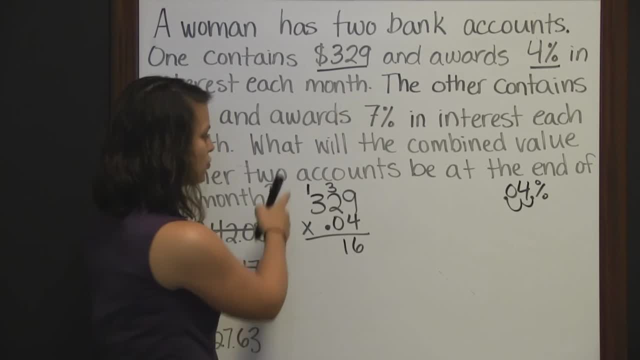 the other 4 times 3 is 12. And 12 plus 1 is 13.. Since we have two numbers behind the decimal place here, then we have two numbers behind the decimal place in our answer. so that means that this account with 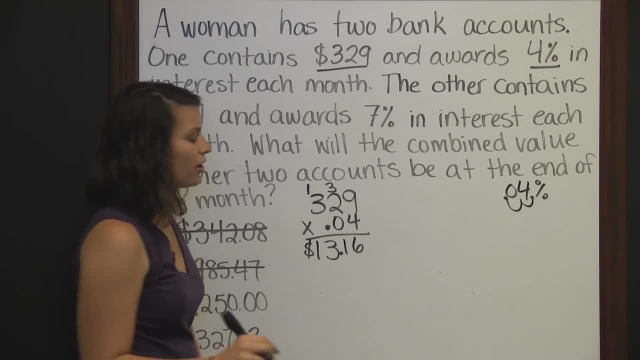 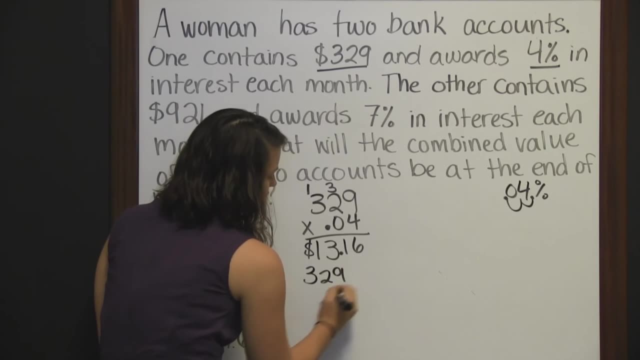 $329 in, it earned $13.16 in interest. So together this account has a total 329 plus $13.16.. When you're adding, you have to make sure that you're adding the correct number. So 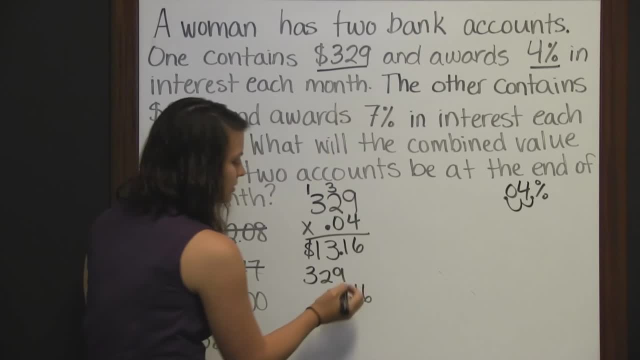 you're adding the correct number. So you're adding the correct number. So you're adding: to make sure to line up the decimal places. The decimal in 329 is at the back and you can add a 00 there to just line everything up. We add those together: 0 plus 6 is 6,. 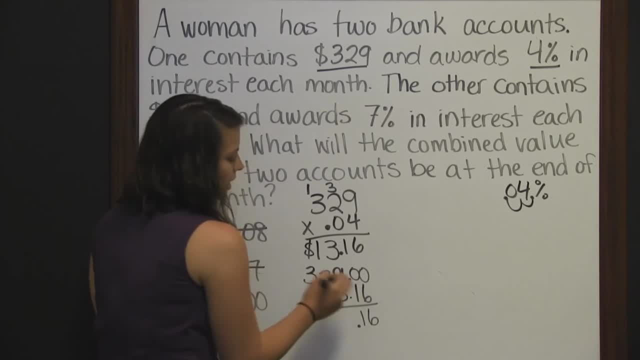 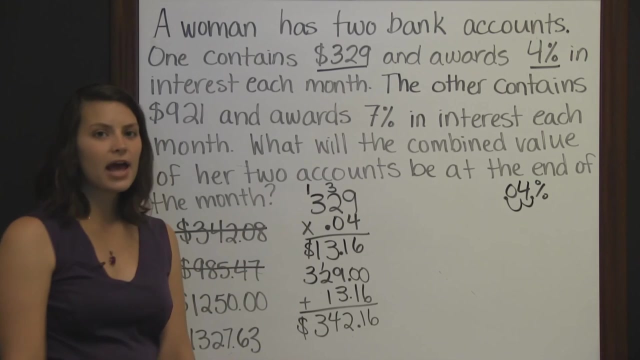 0 plus 1 is 1, bring down the decimal. 9 plus 3 is 12, write the 2, carry the 1,, 2, 3, 4.. $342.16 is what's in the first account. at the end of the month, The next account starts. 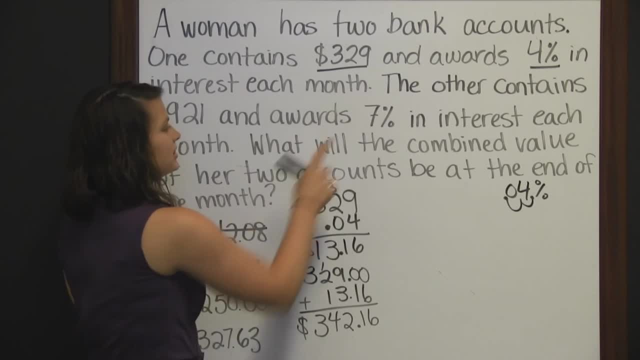 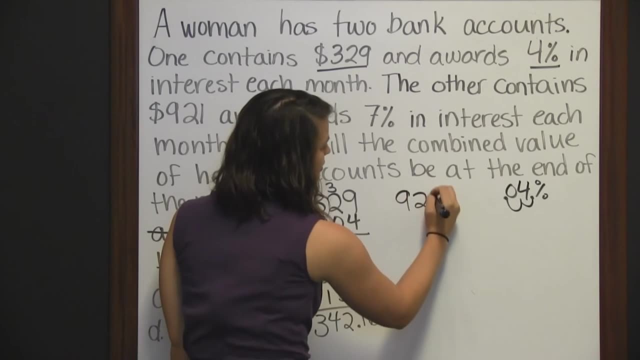 with $921 in it and it earns 7% in interest each month. that means that we are going to take our $921 and multiply that times 7%, This account earns $aturable interest daily. We just sum it up Then again, the amount goes up If we 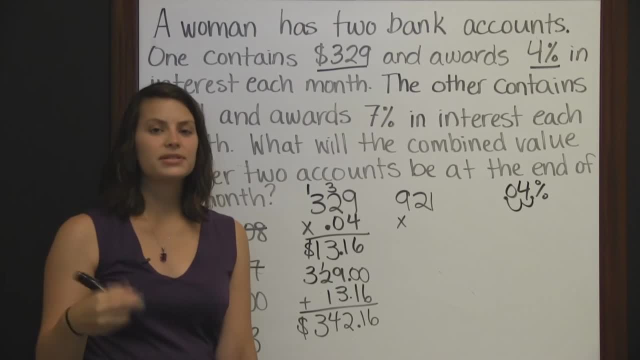 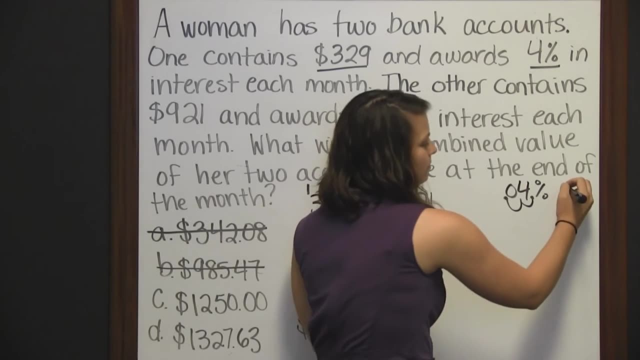 add that in here. first check the. & is the final sum- branch of 921.. The decimal place 7%, interest, 7% of the total and of means to multiply. So we've got to do the same thing we did with 4%. 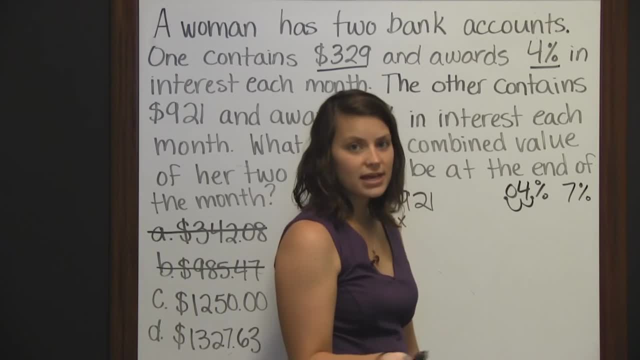 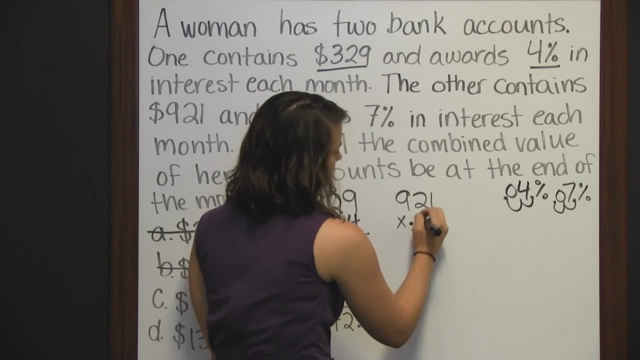 Take our 7% and change it to a decimal, The decimal's in the back, move it two places to the left and it's 7 hundredths. So we multiply 921 times 7 hundredths so that we can find out how much interest was earned in this account. 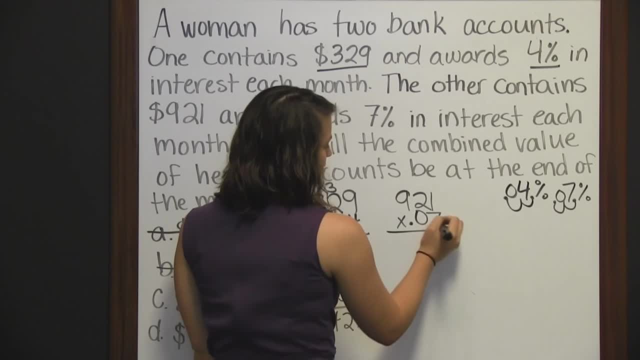 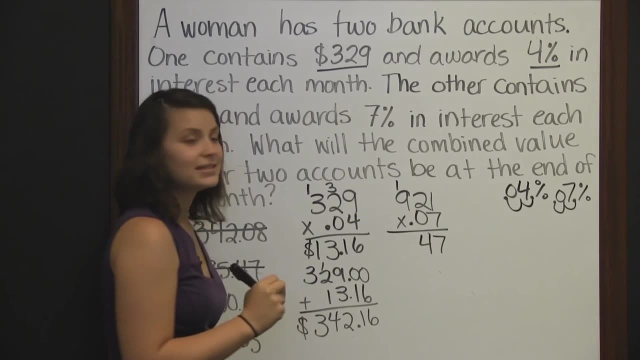 7 times 1 is 7.. 7 times 2 is 14, write the 4, carry the 1.. 7 times 9 is 63, plus 1 is 64.. And since there are two numbers behind the decimal place, 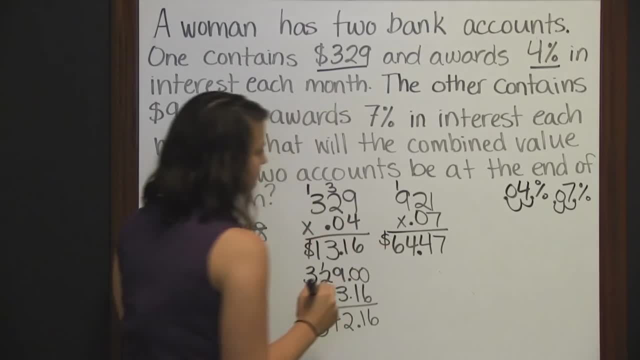 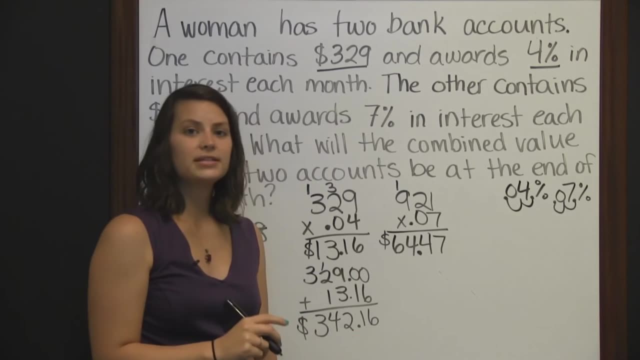 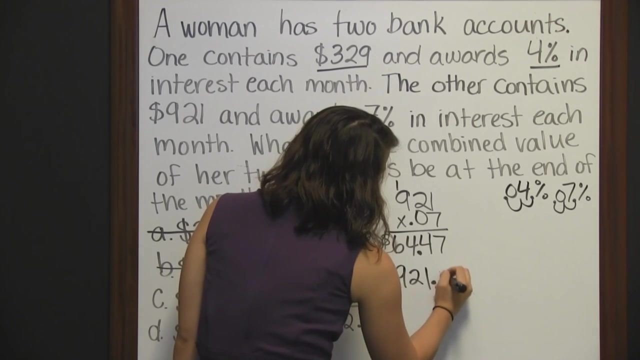 we need to have a decimal, So we have two numbers behind our decimal place. So this account with 921 dollars in it earned 64 dollars and 47 cents in interest. So all together, when we add 921, again, we can put that decimal at the zeros. 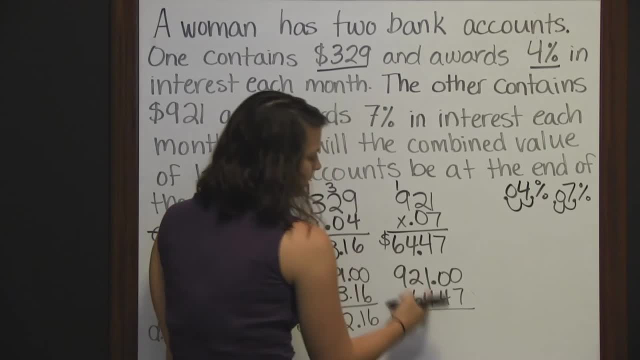 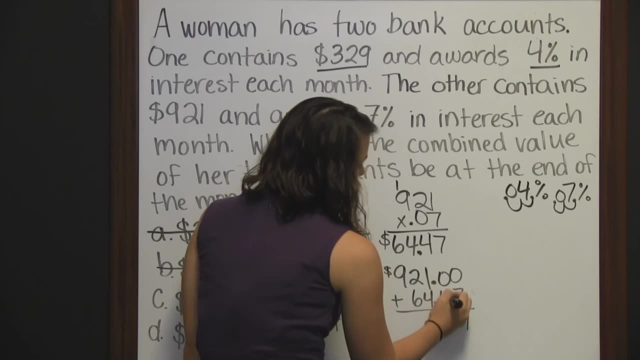 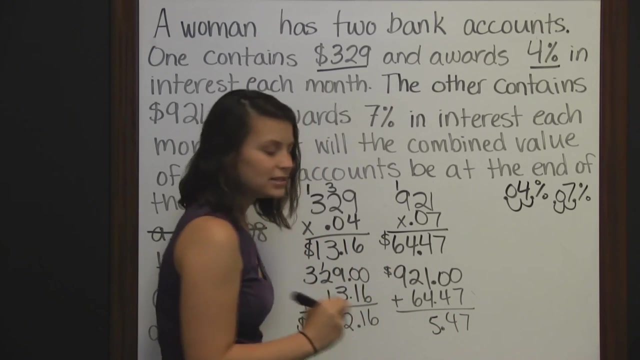 and then the 64 dollars and 47 cents. line up those decimals when you're adding: 0 is 7,, 0 plus 4 is 4,. bring down the decimal: 1 plus 4 is 5,, 2 plus 6 is 8,, 9 plus nothing is 9.. 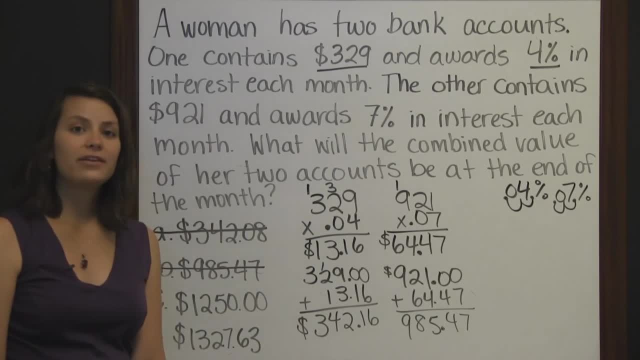 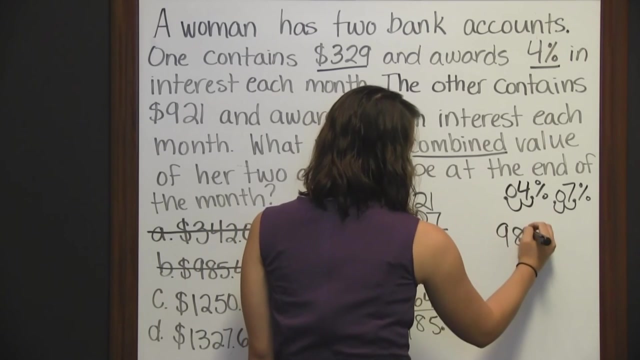 So that account has a total of 985 dollars and 47 cents in it. Now again, we're looking for the combined value of her two accounts, which means that we've got to add those two accounts together. So we have 985 dollars and 47 cents. 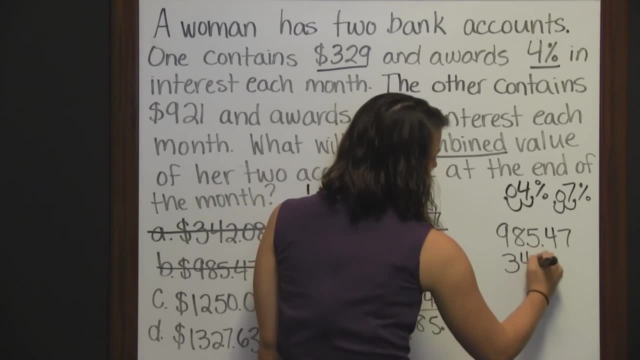 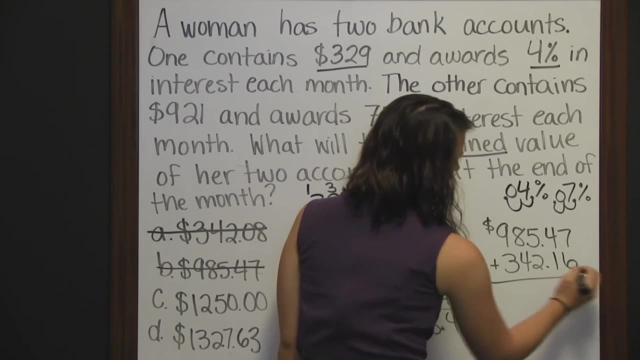 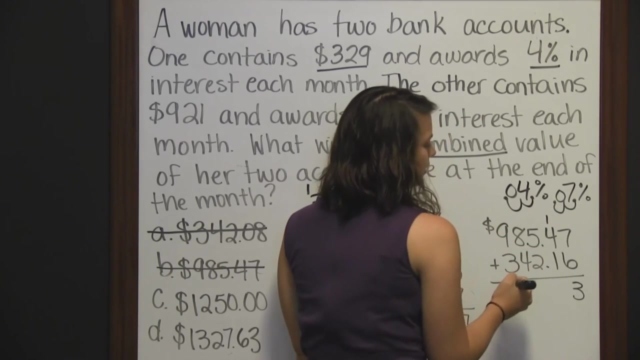 And then we add to that the 342 dollars and 16 cents. Line up those decimals. 7 plus 6 is 13,. write the 3,, carry the 1.. 4,, 5,, 6, bring down the decimal. 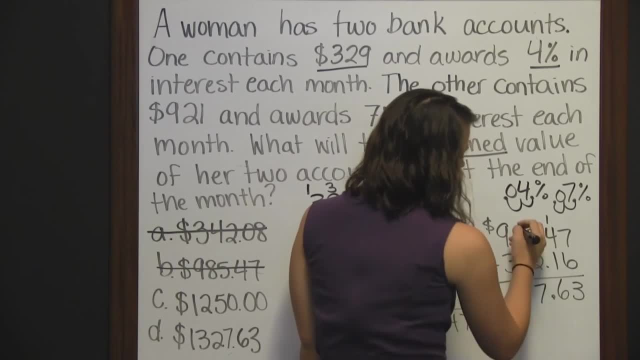 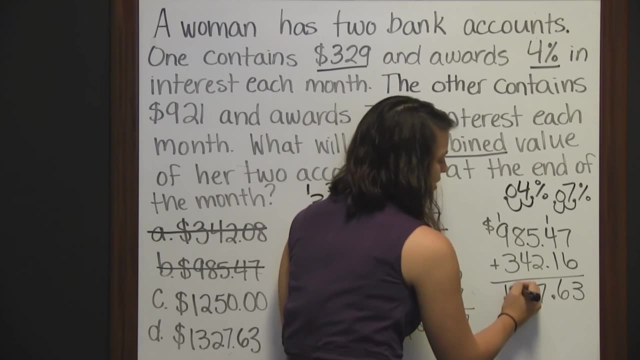 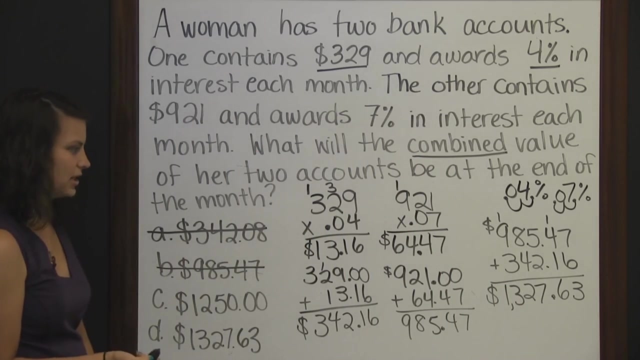 5 plus 2 is 7.. 8 plus 4 is 12, write the 2, carry the 1.. 9,, 10,, 11,, 12,, 13.. So we get 1327 dollars and 63 cents, which we can see is answer choice D. 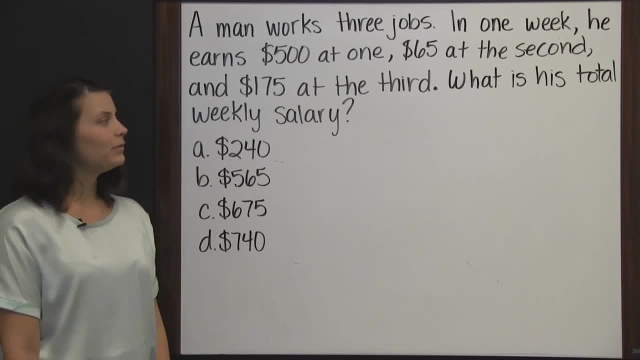 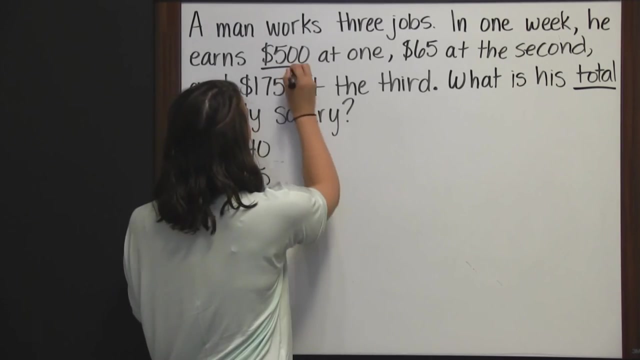 A man works three jobs In one week. he earns 500 dollars at one, 65 dollars at the second and 175 dollars at the third. What is his total weekly salary? This word total tells us that we need to add up all of the money he earns. 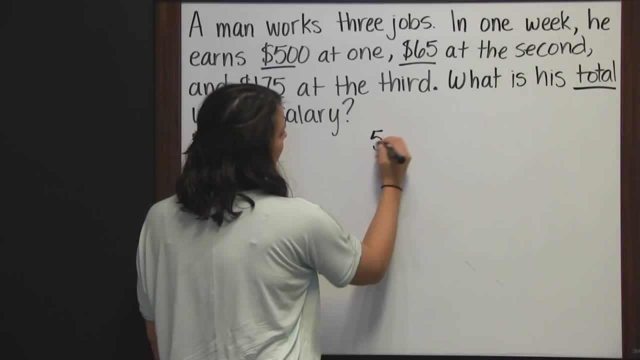 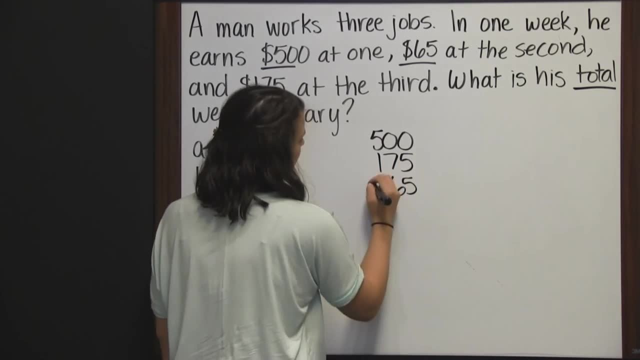 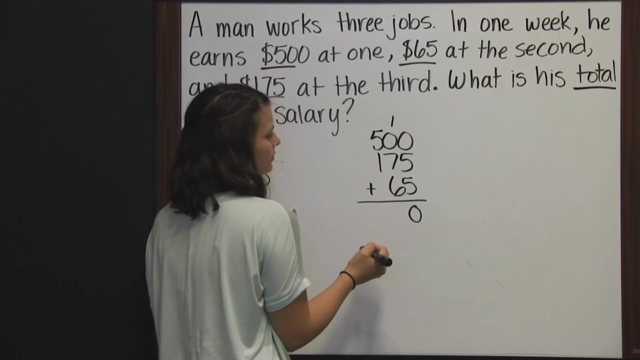 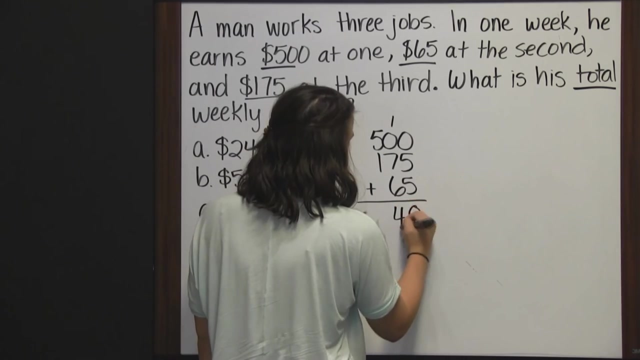 from all three of his jobs, So 500 plus 175 plus 65.. 5 plus 5 is 10,, so write the 0,, carry the 1.. 6 plus 1 is 7, and 7 plus 7 is 14,, so write the 4,, carry the 1.. And then 5,, 6,, 7.. So that means from his three jobs he makes 740 dollars. If one acre of forest contains 294 pine trees, how many pine trees are contained in 25 acres? This is a multiplication problem. 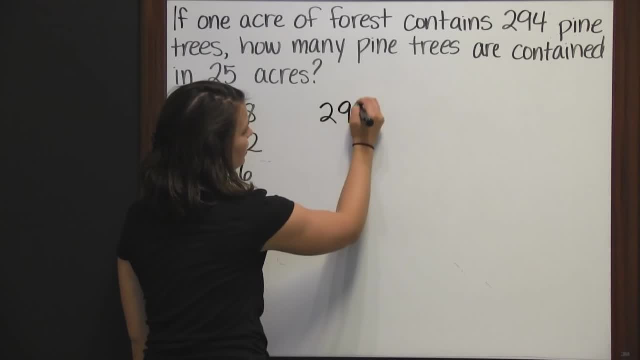 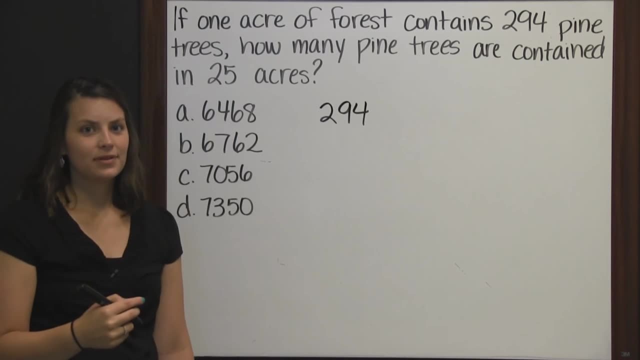 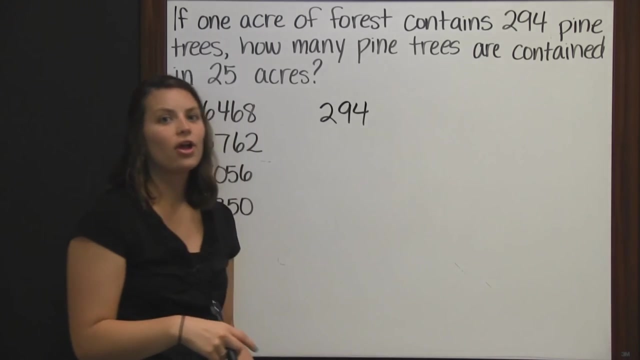 There are 294 pine trees, 294 pine trees in one acre and we have 25 of those. So there are 294 pine trees here, 294 pine trees in this acre, 294 pine trees in this acre, So you could add 294 to itself 25 times. 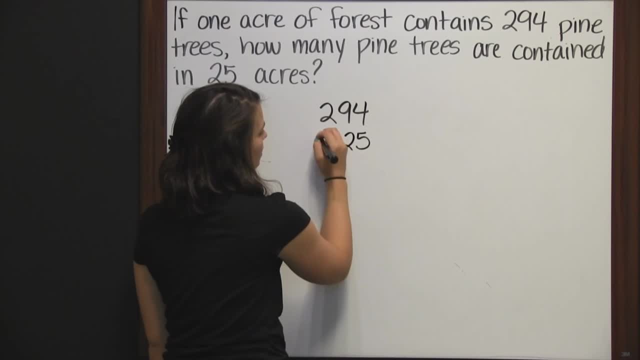 or you could just multiply 294 times 25.. 5 times 4 is 20,, so write the 0 and carry the 2.. 5 times 9 is 45, plus 2 is 47,, so write the 7, carry the 4.. 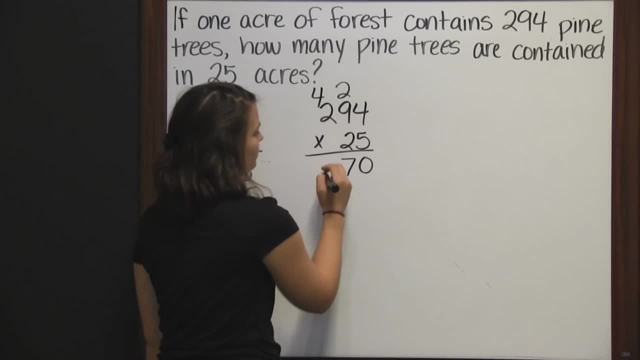 5 times 2 is 10, plus 4 is 14.. And we'll get rid of these. Put a 0 placeholder to move over to the 10s place and multiply 2 times 4 is 8.. 2 times 9 is 18, so write the 8 and carry the 1.. 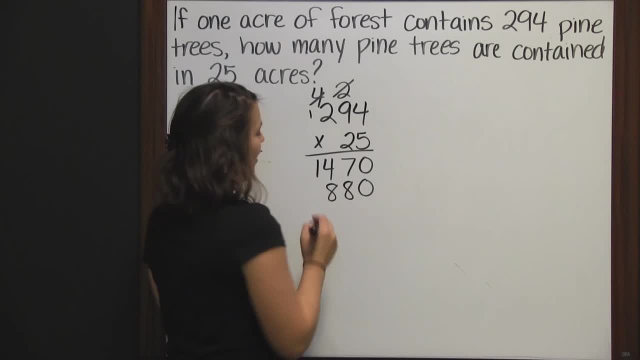 2 times 2 is 4, plus 1 is 5.. And then we add these together to get our final answer: 0 plus 0 is 0.. 7 plus 8 is 15, write the 5, carry the 1.. 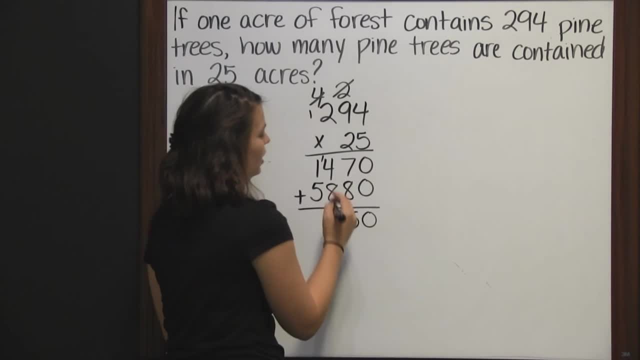 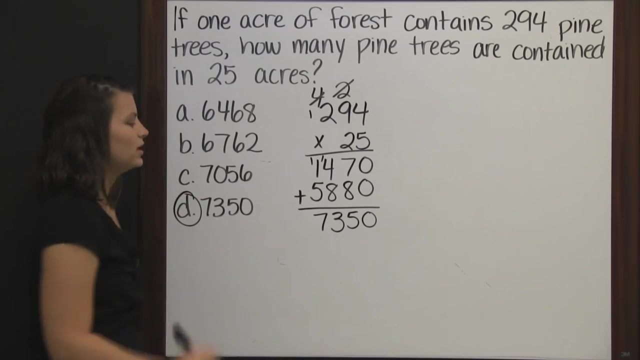 8 plus 4 is 12, plus 1 is 13,. so write the 3,, carry the 1.. And we have 5,, 6,, 7.. So there are 7,350 trees in 25 acres, which is answer choice D. 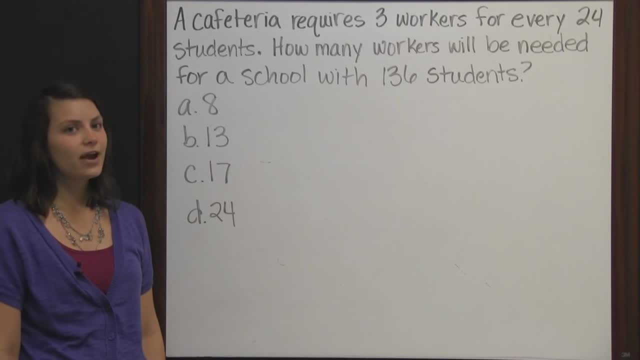 A cafeteria requires 3 workers for every 24 students. A cafeteria requires 3 workers for every 24 students. How many workers will be needed for a school with 136 students? So first we need to determine how many students there are for every 1 worker. 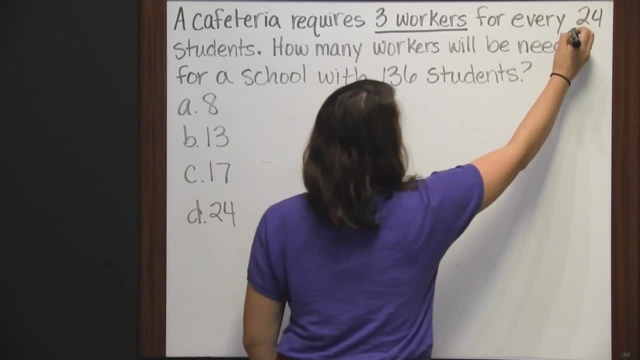 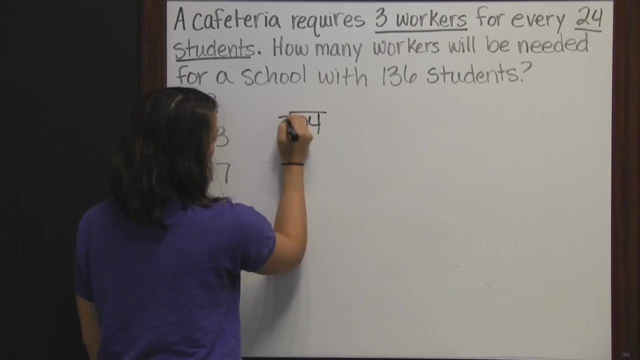 So we're going to start with this information: 3 workers for every 24 students. So we take 24 and divide it by 3.. 3 goes into 24. 8 times 8 times 3 is 24.. So there's no remainder. 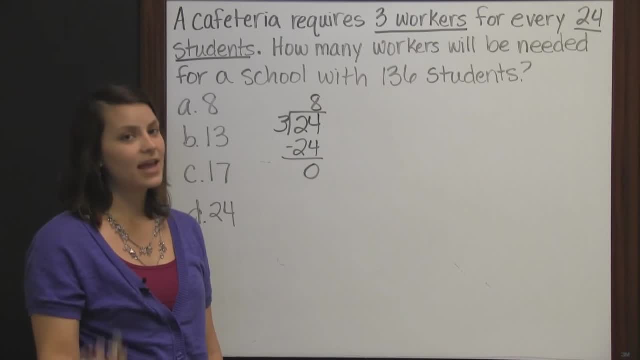 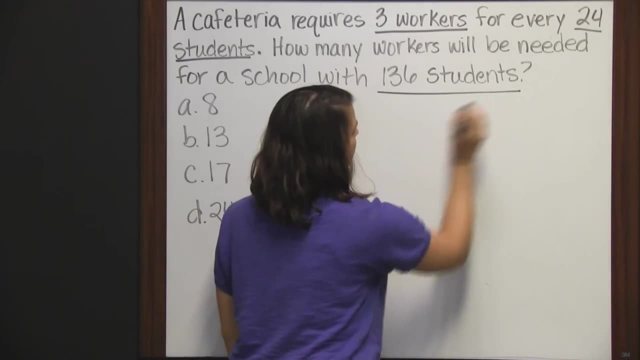 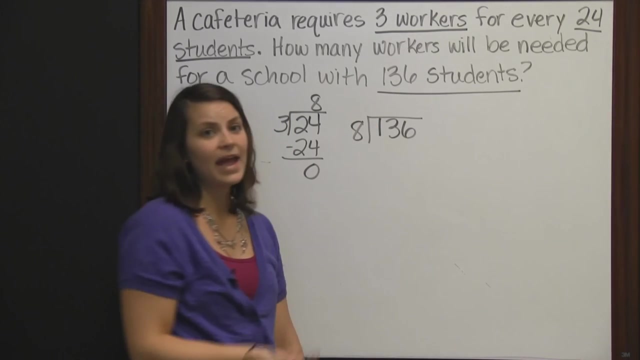 That means there's 1 worker for every 8 students. With that information we can figure out how many workers are needed for 136 students. So we take 136 students and divide it by 8 students to figure out how many workers we need. 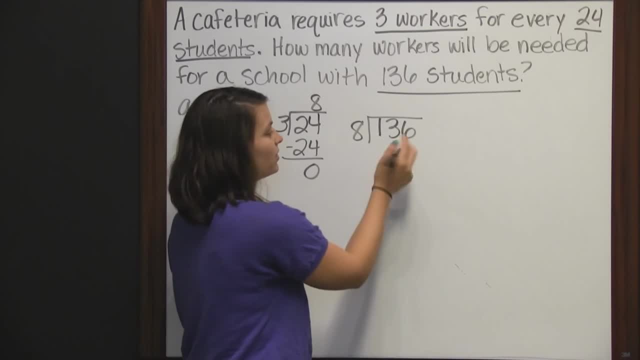 8 does not go into 1, but it does go into 13.. 8 goes into 13. one time 8 times 1 is 8. And when we subtract 13 minus 8, we get 5.. Then we bring down our 6.. 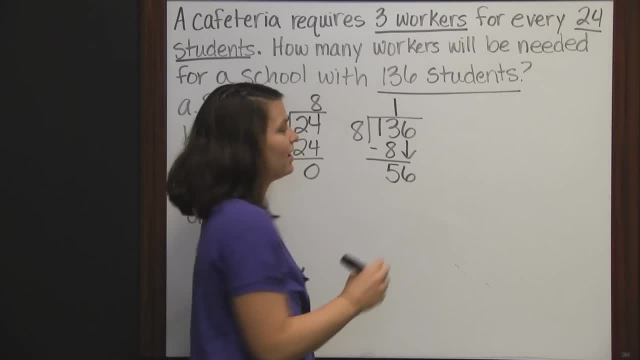 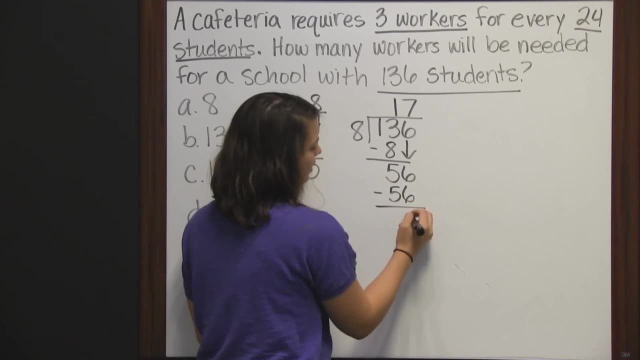 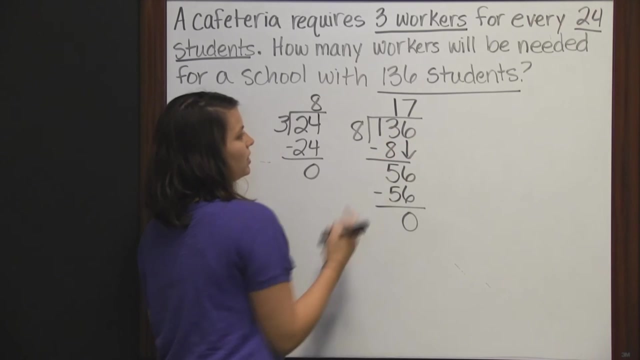 8 goes into 56. seven times 8 times 7 is 56. And we subtract and have no remainder. So that means we're going to need a total of 17 workers for these 136 students, which is answer choice C. 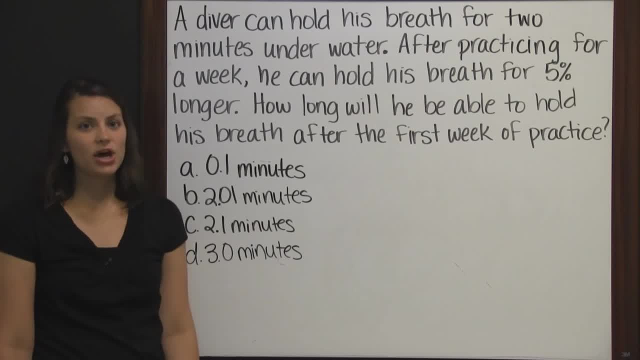 A diver can hold his breath for 2 minutes underwater After practicing for a week. he can hold his breath for 5% longer. How long will he be able to hold his breath after the first week of practice? So he can hold his breath for 2 minutes before he starts practicing. 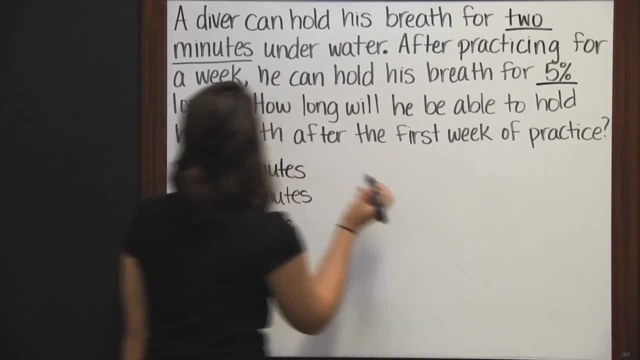 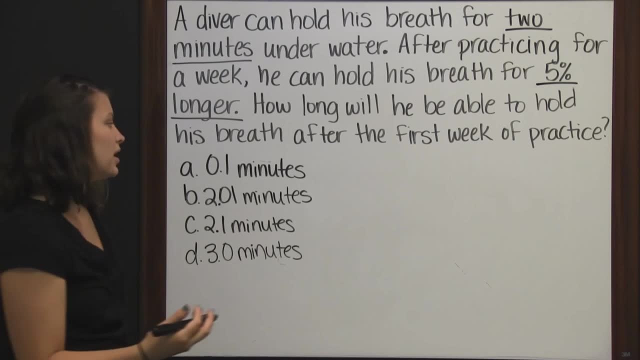 And then, after practicing, he can hold it for 5% longer. So that means that he can hold his breath for longer than 2 minutes now. So we can already eliminate answer choice A, Since it is not longer than 2 minutes. 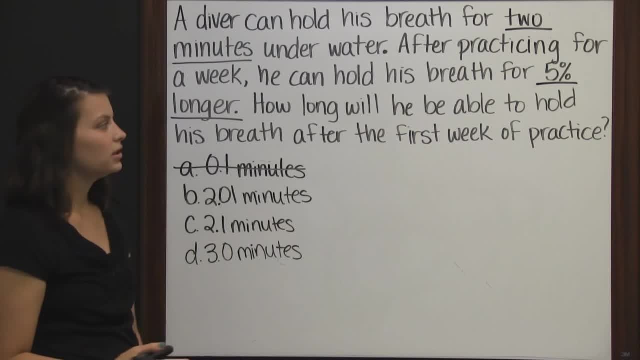 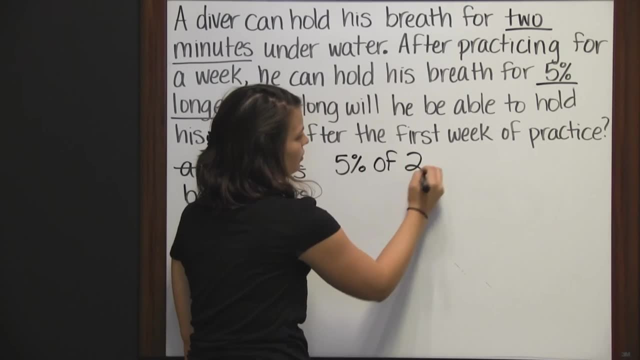 To find out how much longer he can hold his breath, we need to take 5% of 2.. Of means to multiply And we have to change our percent to a decimal. So take the decimal and move it 2 places to the left. 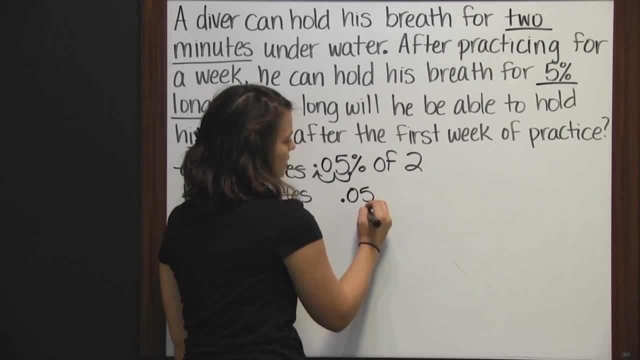 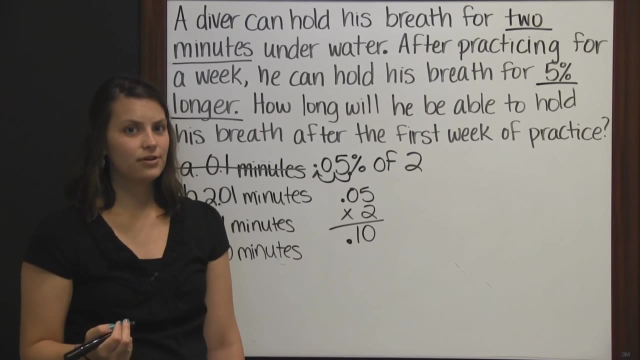 So we have 5 hundredths times 2.. 2 times 5 is 10.. 2 numbers behind the decimal means that we have 2 numbers behind the decimal in our answer. 5% of 2, then, is 1 tenth. 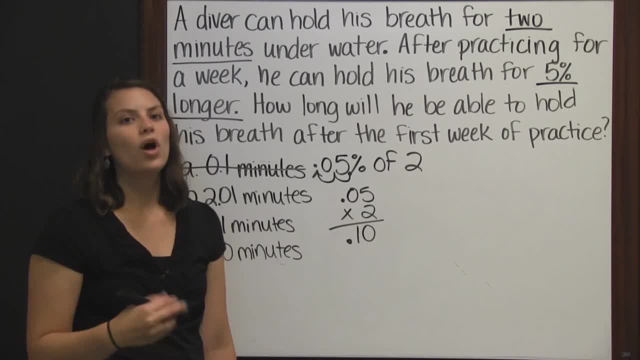 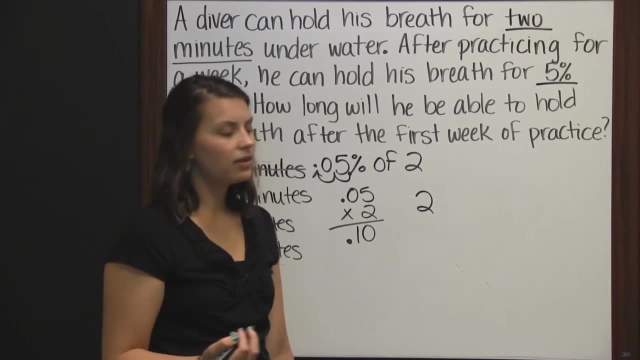 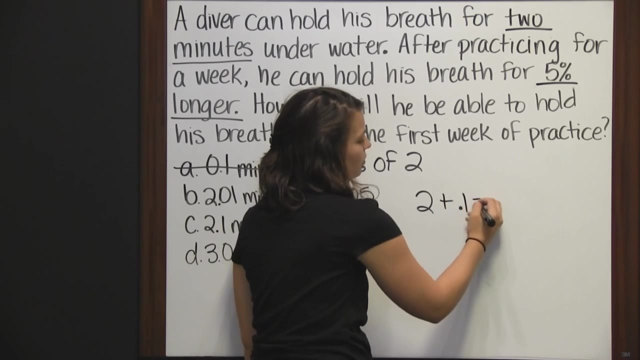 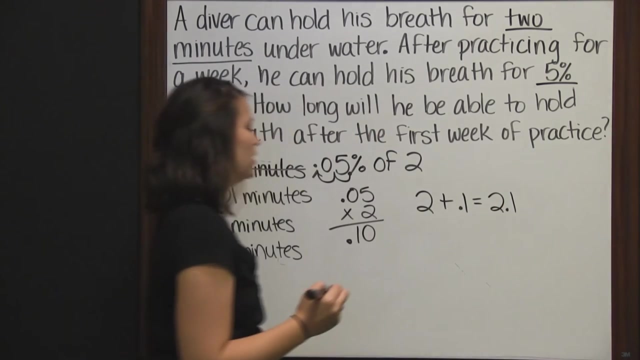 So he can hold his breath 1 tenth of a minute longer. So he started with being able to hold his breath for 2 minutes And now he can hold it for 1 tenth of a minute longer. So we add 2 plus 1 tenth and we get 2 and 1 tenth. 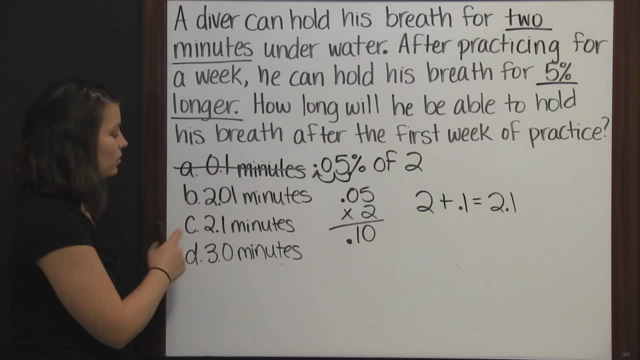 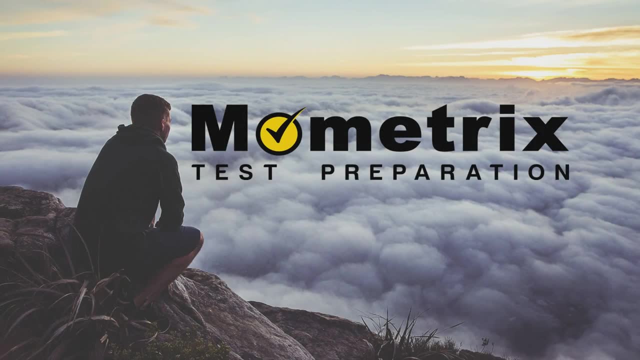 So he can now hold his breath for 2 and 1 tenth minutes. Answer choice C: Alright, let's make it simple. How do we explain this one? Well, if we raise the value of the number we want to solve in a decimal, and we will plot the number below that qualifies as 1, then what is the number below that is given as 0, and how will we calculate it? Because the answer will show that it is 12та and the value below it is 1.. The value little by the value of 1Is equal to 22.. So we can now multiply by this. If we increase the value.